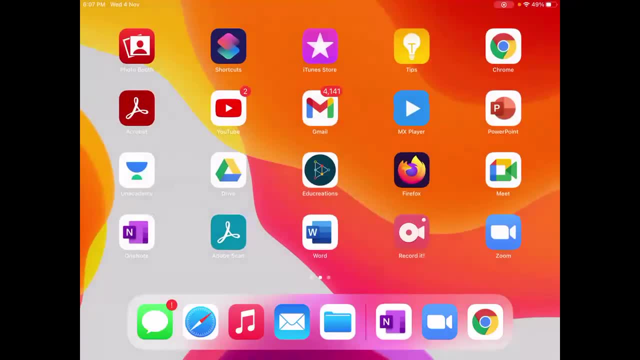 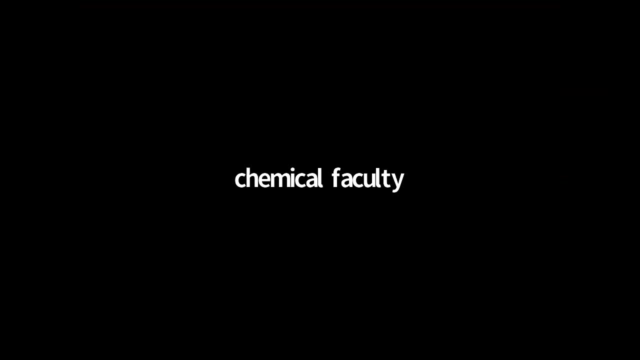 Wait for a minute. Okay, The system got hanged. Wait, Wait a second, I have to check the settings. Oh, okay, So let's talk for one minute. Okay, So that is the thing. Okay, fine, Okay, So basically this: 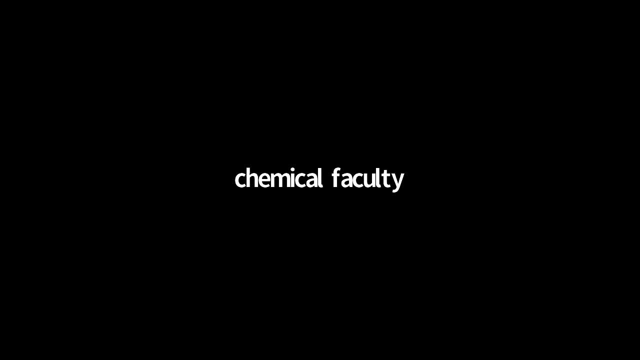 this counted cash flow, is that? suppose your friend is there. Okay, having a name Nishant, I'm not writing anything on the board. Okay, just wait for two minutes. So he has taken 100 rupees from you. Okay, in the BTEC days it is very difficult to give money to some friends. Okay, still, some friends manages to give the money. Okay, suppose Nishant has given money to some person, Aman. Okay, then Aman is clever What he told. Okay, I will return this money. 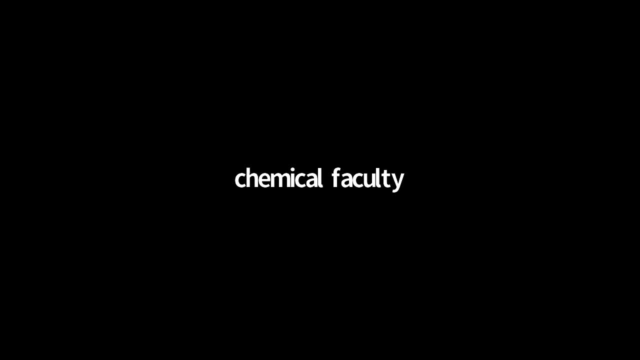 jiocide to you after one year. Okay, but I will not return 100 rupees. I will give you 150 rupees, Okay, But if you want today, I will give you 100 rupees after one year, after 150 rupees. 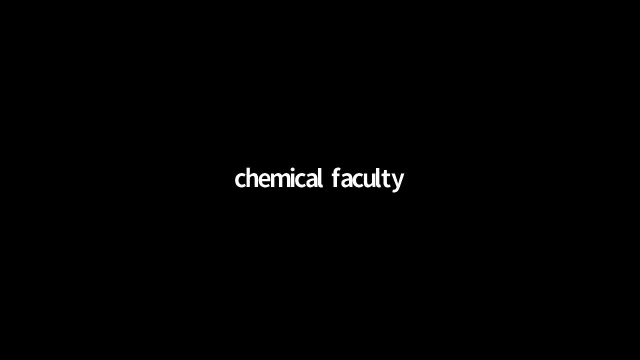 Niектор. So you might be thinking: okay, he's a very good person, He is giving 150 rupees because he has given- he has taken from me only 100 rupees. But here how much discount he is giving- after one year he will be giving 150 rupees- means how a discount he is giving to for giving today. 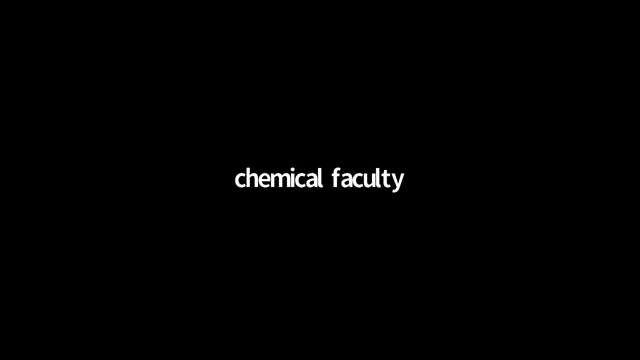 crowded. rupes discount, rupes Give, rupes discount. here is is giving. so that is the thing: the future value. he is coming comparing with the present value. okay, so you know the actual rate of interest of the market scenario. okay, so you will calculate. 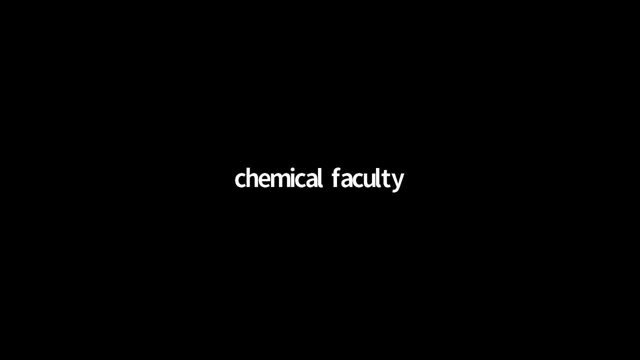 okay, suppose you have given 100 rupees, you will calculate with respect to the seven percent. okay, and you are thinking that i will invest that hundred rupees in the mutual fund, and mutual fund gives you return of seven to ten percent. so you will calculate. so it is coming one one hundred. 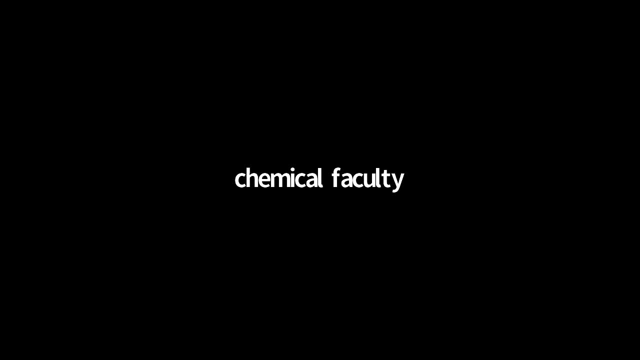 and eighty rupees. okay. so then you will tell to one that if i give this money to mutual fund or anyone else, then the money is coming 180 rupees. okay. so how can you giving me 150 rupees, one after one year? okay, so that is. discounted value means that future value will be compared with the. 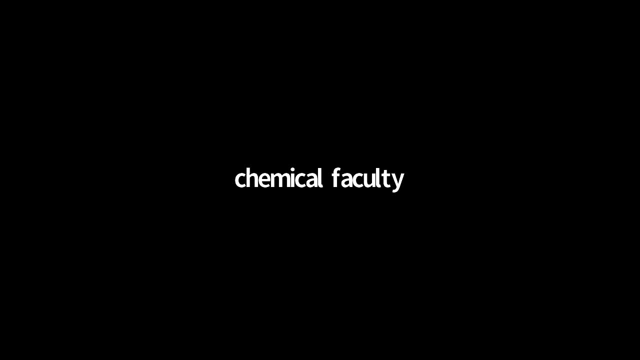 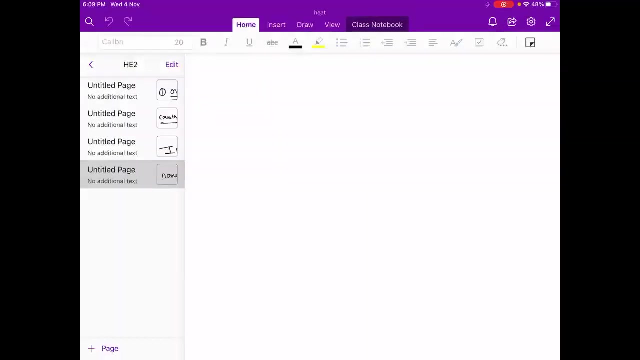 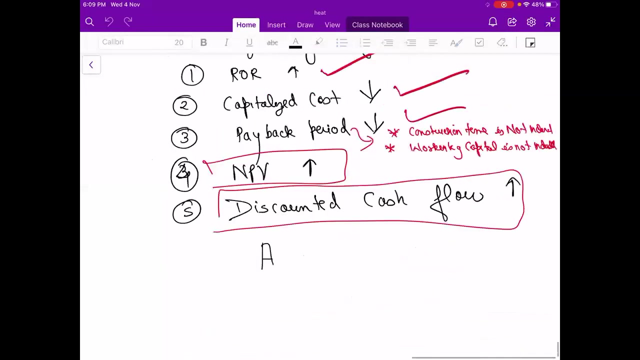 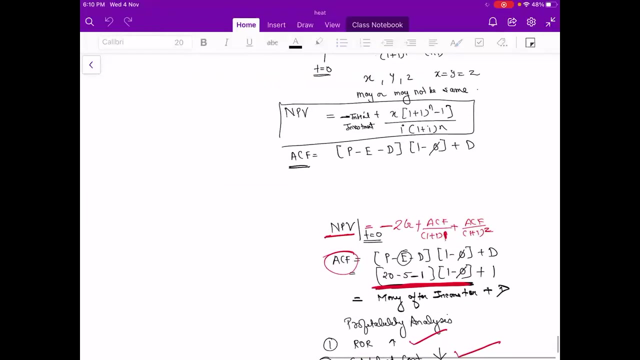 present value. so that much amount of that much amount of discount is known as okay, that much amount of discount is known as you, yeah, wait, wait, yeah. now it's okay, discounted, okay. i think this. this is completed. wait for a second. okay, the screen is caught and 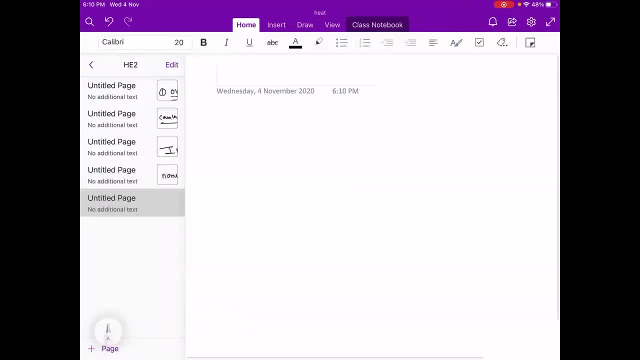 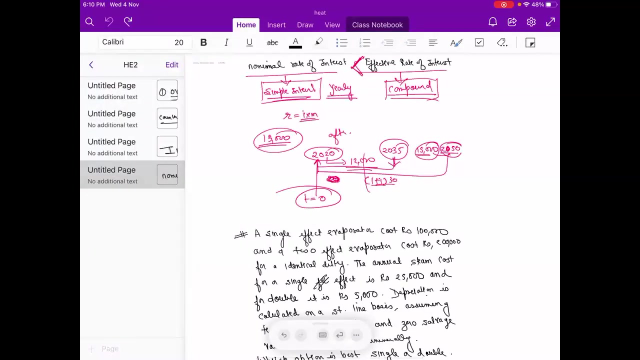 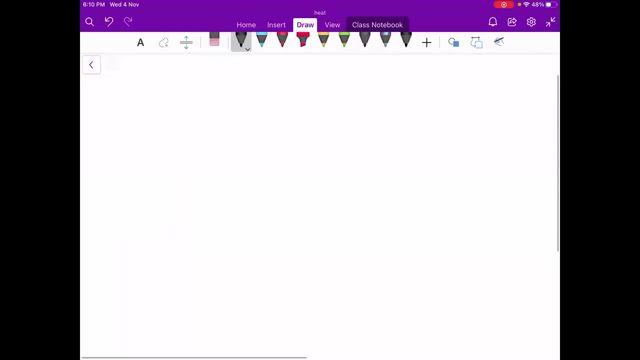 let's have start with new page, okay, fine, wait, let's see. suppose you have 100 rupees. you have given that 100 rupees to anyone else, so he told that he will return back to you 150 rupees after one year. okay, after one year period, okay. 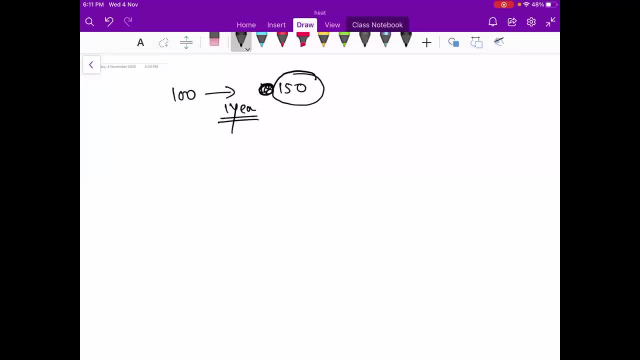 so that 150 rupees is the future value. the present value should come hundred rupees. okay, if it is not coming hundred rupees, it means that it means that he is giving rs, is giving wrong money. okay, because he is not calculating money as a function of time. 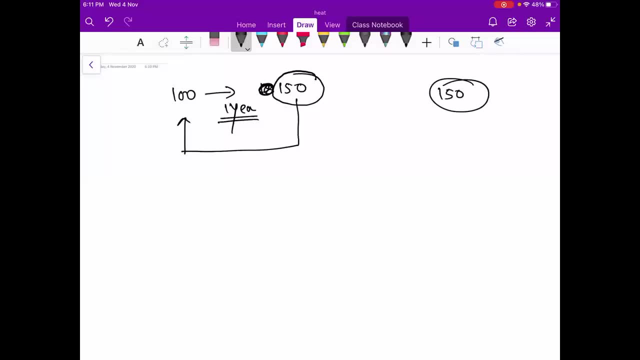 it means that, suppose 150 rupees, what is the interest? what is the interest to come back to the 100 rupees. okay, we'll say, just solving like this. see here, 100 equals to future value will be 150, 1 plus any rate of interest. you take 7. so this should be come back to 100. so you are giving. 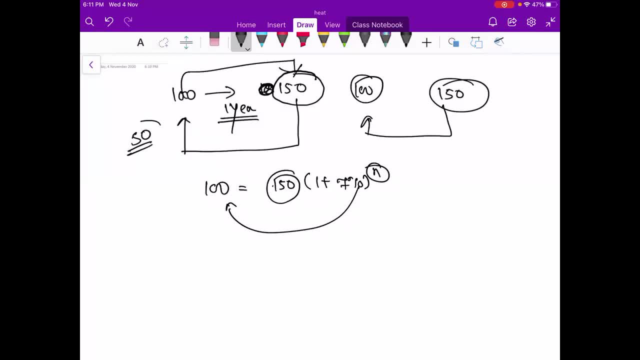 discount of 50 rupees. okay, you are giving discount of 50 rupees because you are coming back from 150 to 100. okay, from future to present. so that is why it is known as discounted cash. so it is nothing. but when we are going see, it is just simple. when it is in the numerator it is just like 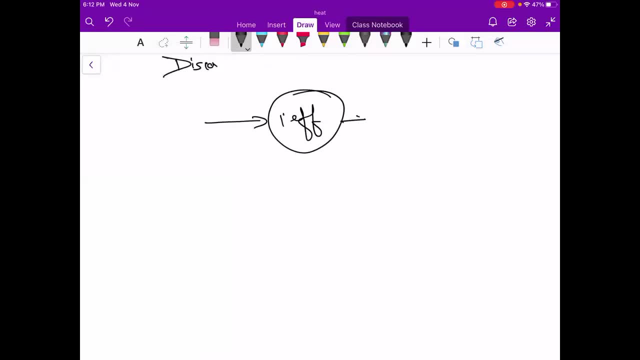 i effective we are calculating. okay means i effective is used when you are okay. i effective is there when you are going from present to present. future okay, and you are using discounted interest when you are going from future to present. so that's it. you see here, 100 equals to 150. so when you divide this, 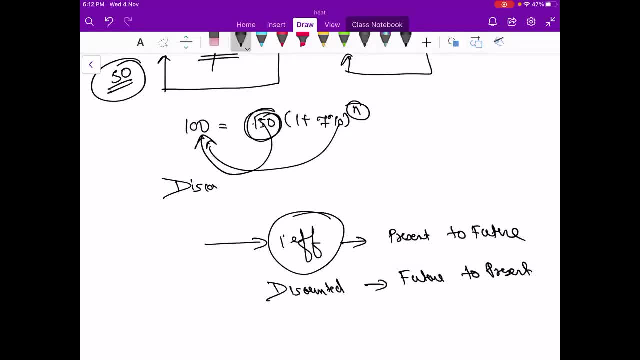 okay, when you will divide this 150 rupees with this. okay, so this is the future and this is the way you will solve that. okay, so this is the meaning of the discounted cash flow. okay means here is the future. value, 150. so what will be is present. value will give you the 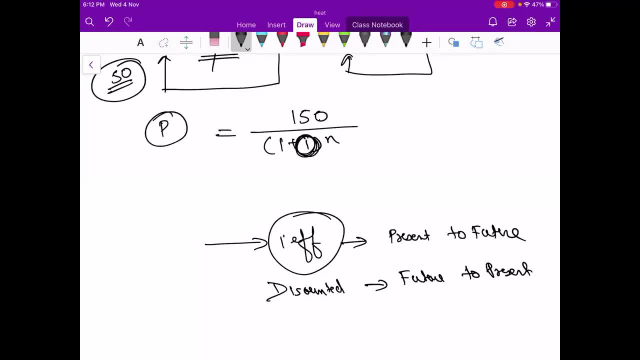 this is the discounted. okay, this is discounted interest. okay, everyone got this. now it is cleared means whatever value you are getting in future. so if you compare this with present value, it is always less than that. present value will be less than that, so the difference is known as discount. 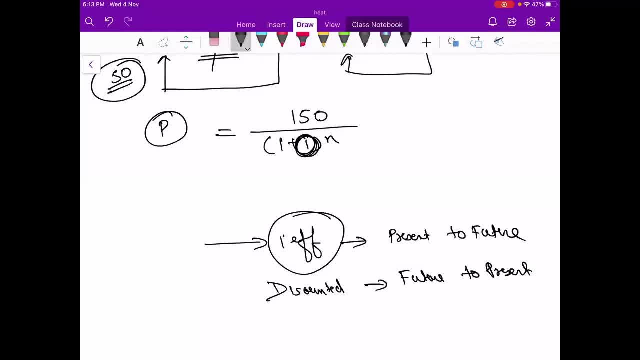 okay, the difference Is known as discount. everyone is cleared with this. okay, now i think everyone is clear. another thing so many students have doubt is ROR. it is nothing but rate of return. okay, everything is in the rate of return. the second is Feinstein's Camellia rate of. 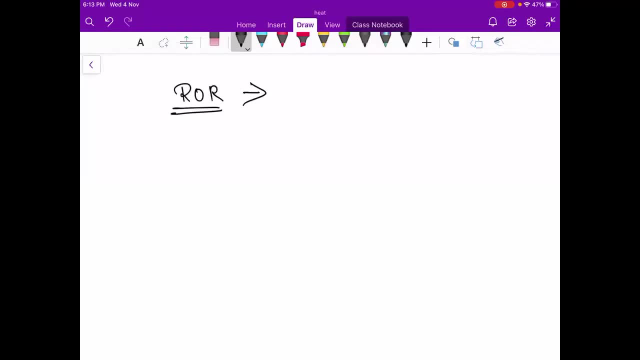 return okay. basically, it is calculating that how much money you have invested okay and how much profit you are per year you are getting. so if you are getting profit per year five lakh and you have invested 20, so it is multiplied by 100. so this answer will the how much rate of return you are. 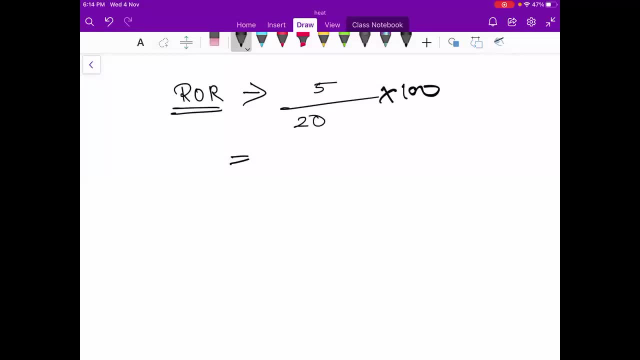 getting every year. okay, annually, you are calculating the rate of return. okay, fine, it is just like in bank: you have deposited some money and you will be getting some interest. total amount divided by how much you have interested, that is the rate of return you will get from the bank. okay, this is the rate of return. okay, everyone is clear. 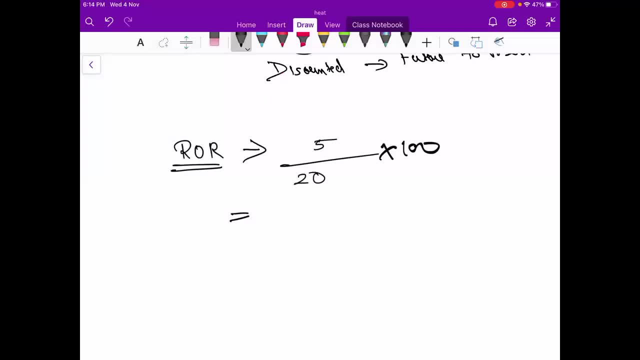 everyone is clear: yes or no, okay, okay, next we will move to our topic, that is npv. so what is npv? net present: okay, net present value. so what is net present value? calculating all your transactions: okay, calculating all your transaction. at time t equals to zero, okay, calculating all your transaction. that. 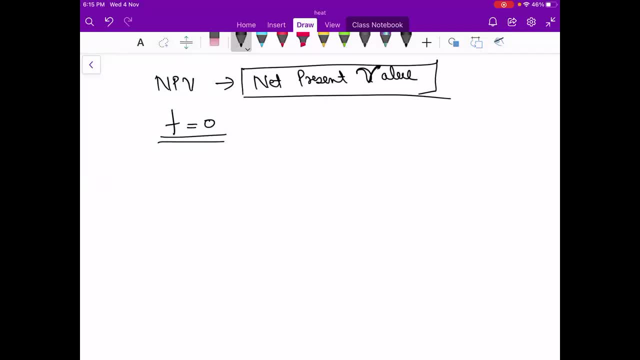 is whether it is profit loss or whatever the transaction is going in the your company. that should be calculated at time. t equals to zero. so for calculating every year transaction we have to calculate the money in terms of acf, which is known as annual cash flow, because initially you 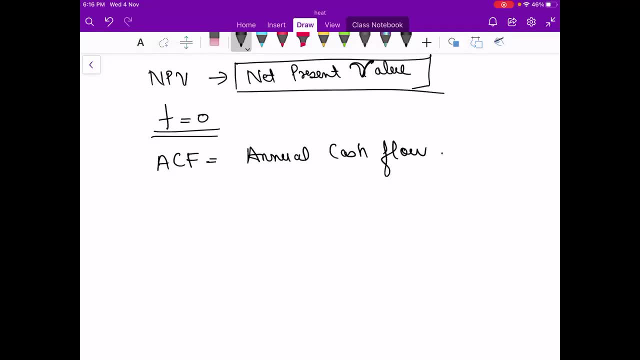 have invested some money. okay, again from the second year. suppose you are getting some profit. okay, so suppose it will be like this: annual cash flow will be like this: i have written, we have written formula: p minus e minus d, 1 minus 5 plus d. okay, this we have written. so basically, what is? 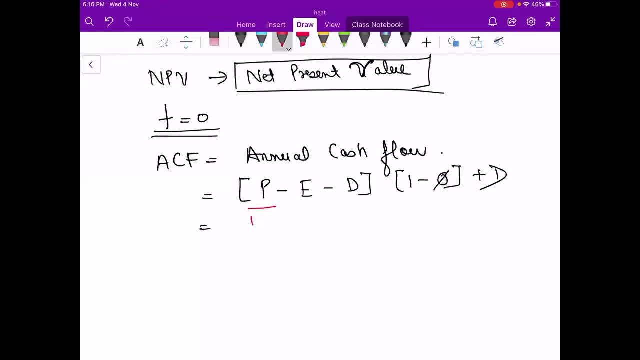 p here. what is p here? profit is expenses, d is depreciation, phi is income tax percentage. okay, so this we have done. okay, so this we have done for the system, okay. so profit was basically, if we have calculated from 12 x 10 x 2: okay, so we have converted 14. 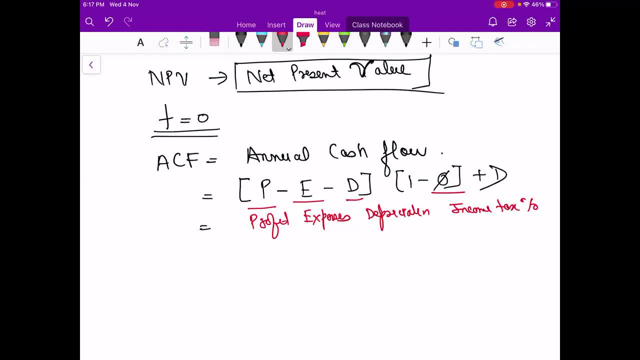 stadtine into 236. nowadays and the interest operating capital you haved advise. então you keep 24000 rupees, so you have solid. so this is your profit coming right now and it's going to be 10 000. okay, how many propositions after your pouquinho just going to power a lot, because are the money what you are getting? okay, that is not your money which is going in your pocket earthy. okay, suppose you have that. you have sold some. I accept, you have sold the IAT worked, so, Ok, suppose you have sold some i makeup. okay, so suppose you have a profit of r 10,000. okay, so is it that this is the money directly going to your pocket? no, from r10,000 you have to subtract some expense. 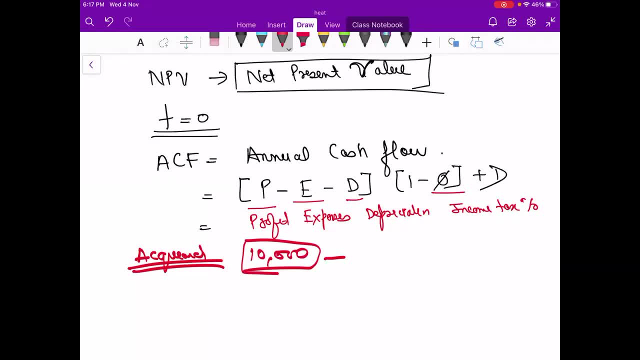 subtract some expenses. okay, suppose some transportation expenses, okay, okay, now then you have to subtract your electricity bill and all that. obviously that is not your profit. okay, you have, you have to pay that money. electricity bill, okay. third is the contingency printer. you, you have some printer? okay, then in that ink is required, so all that you can say contingency. 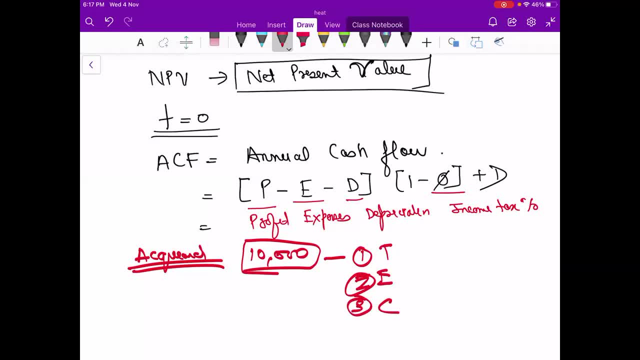 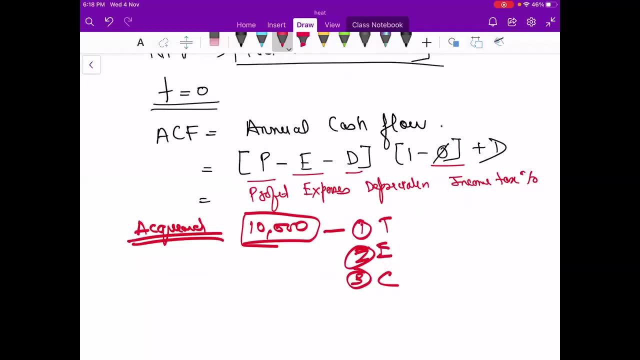 bills. okay, so that is the expenses you have to pay. okay, then d means why we are subtracting d from here: because government says you don't have to pay the taxes on the depreciation amount. okay, so don't have to pay the taxes on the depreciation amount. does that is the thing that i have told. 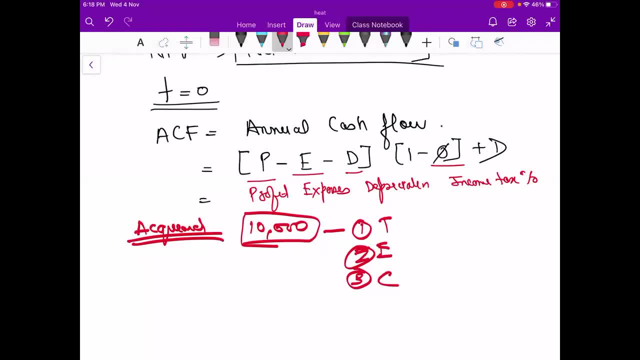 while i'm teaching the depreciation also okay, because depreciation is always okay. okay, that depreciation is always the things. uh is for the you can say government okay, but for us it is not the depreciation okay. so that is why we have to subtract it from here, because government says you don't have to pay the taxes on the depreciation amount. 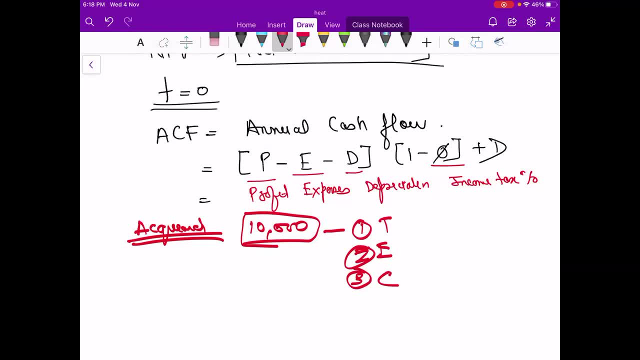 depreciation. so 1 minus 5 plus d plus d. why we have to do? because i told depreciation is not for us, it is for the government. okay, so simply, this is the actual annual cash flow for that company every year. okay, p minus e minus d, 1 minus 5 plus d. so this is the annual cash flow. 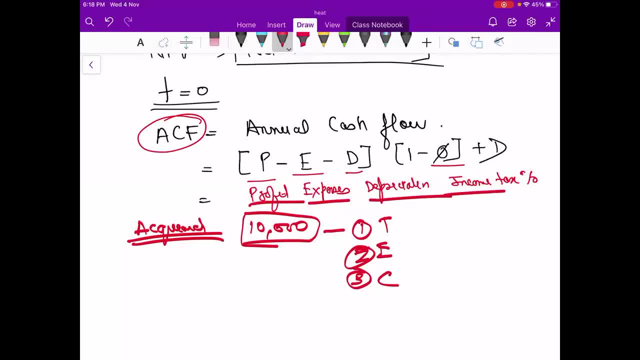 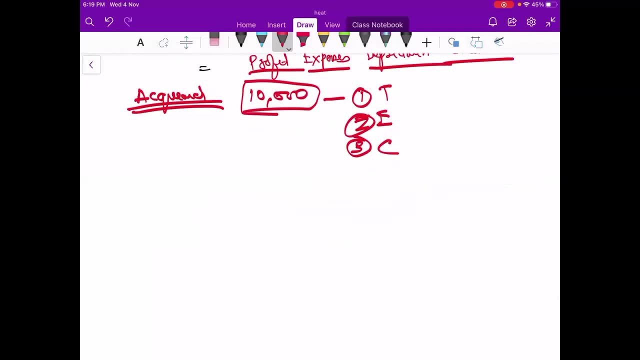 so this is profit minus expenses, minus depreciation, income tax plus d. okay, so this is the thing we are getting. so it means that when i have to calculate the okay, it means that i have to calculate the npv. at time t equals to zero, okay, at time t equals to zero. 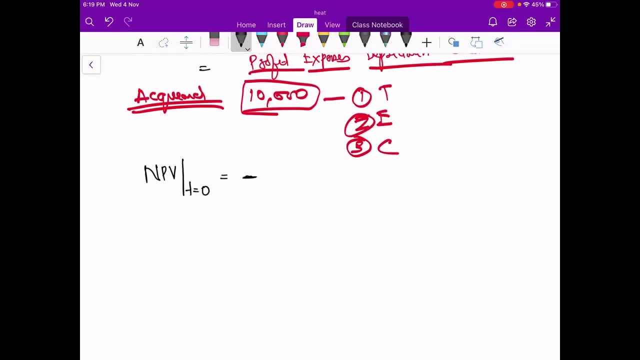 it will be the money i have invested, so it will be always negative. okay, invested money, because this amount of money you have invested every year, that acf will be every year. so it will be acf 1 plus i to the power n minus 1 upon. 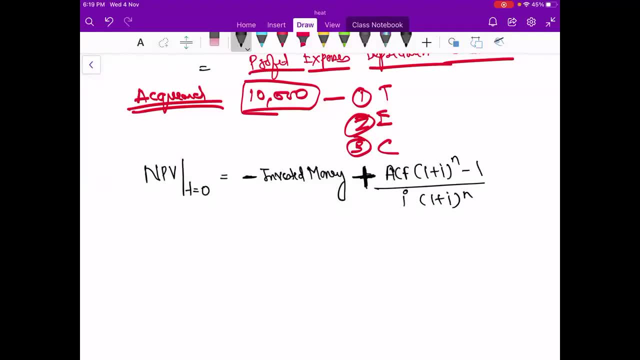 i, 1 plus i to the power n, so this will give me the npv formula. okay, so if someone- if suppose you don't have acf value and at time t equals to zero- someone will ask: suppose this is an industry for you. and someone has asked: you have invested 2 crore rupees, so initially you will be obviously 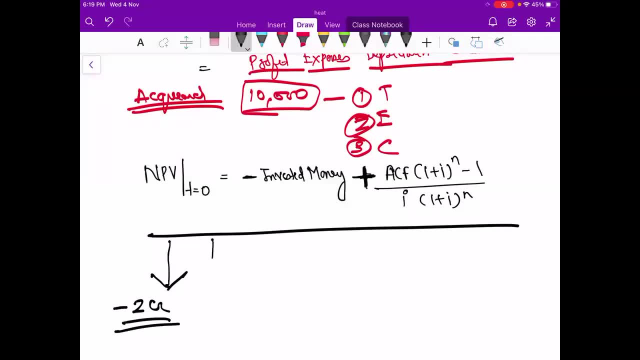 minus 2 crore rupees loss. but at the second year you will get some acf. it will get acf. it will come with your curve, will like go like this. so at some point it will be intersect with this one that at this point the npv is zero. there will be one point when i say npv will be zero, then it will. 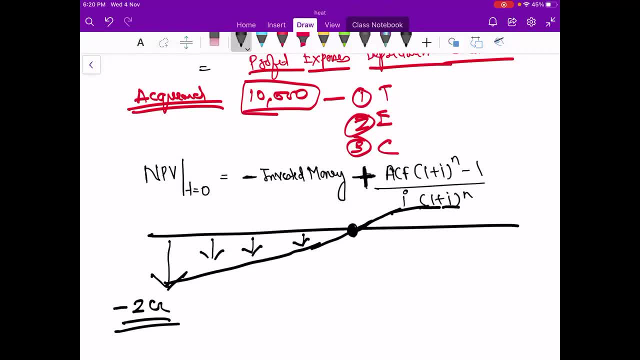 go up like this. okay, so this is the thing of npv. okay, so everyone got this point. yes, t equals to zero means the moment your plant will start. okay, t equals to zero means the moment your plant will start. yeah, this is the formula of nvt. okay, this second term is the formula of nvt that we have seen. 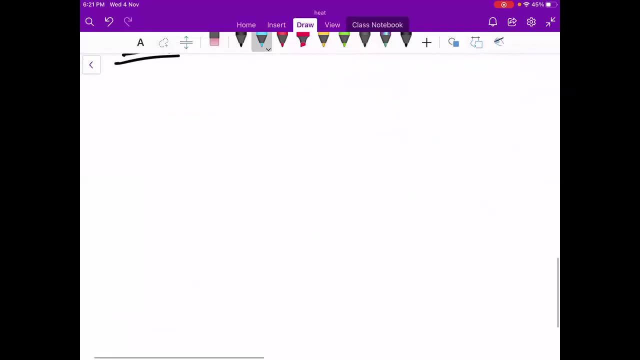 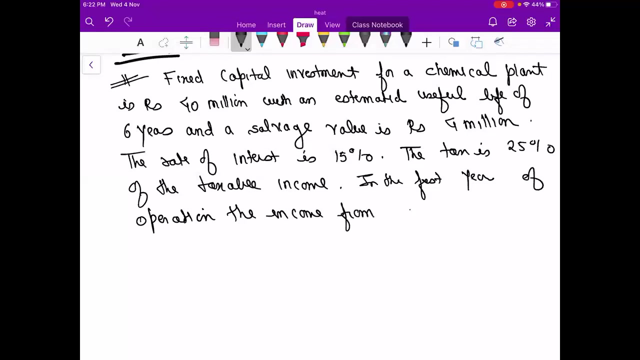 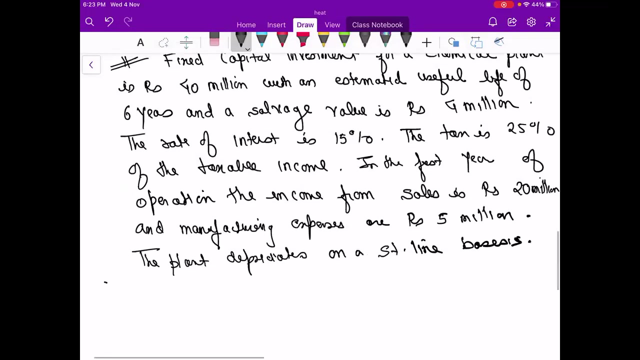 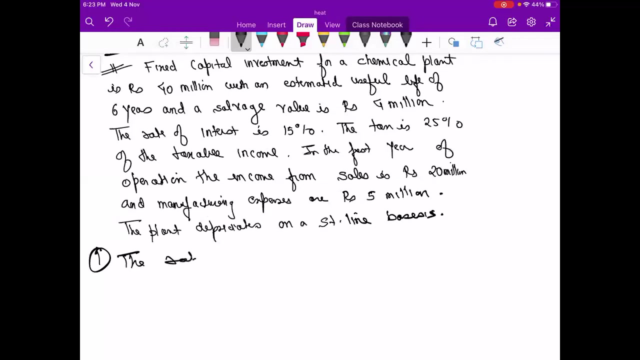 okay, let's see a question. then. most other students, which you have doubt that can be cleared. okay, fixed second npv at the start of the year and at the end of the year of operation. okay, calculate this. so let's take a time, read the question properly and then solve it. okay, it is a great question for a four mark. 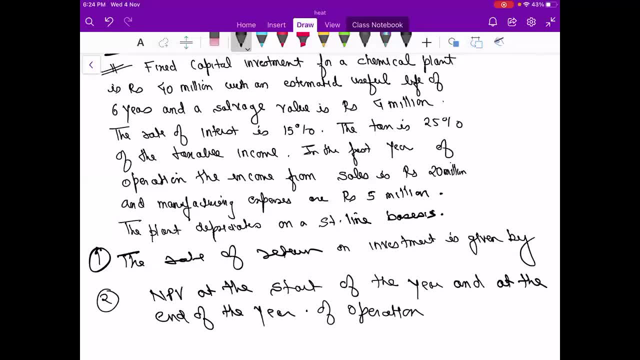 after this, i will clear all your doubt. okay, first attempt this question to answer: how to solve this question, okay, okay, this is very important question actually. it will clear all your doubts. you solve this. you, you, you, you, you all this very important question, think on it. all this very important question, think on it. 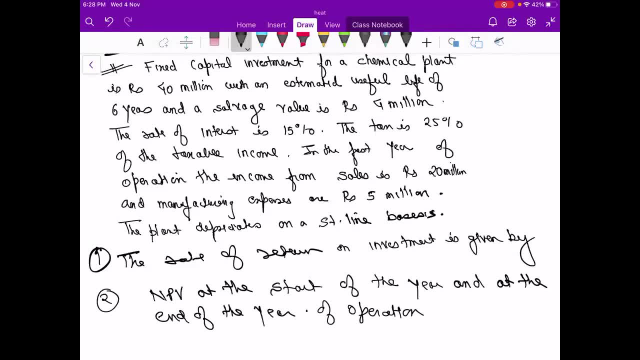 are the, the are the, the are. so many students are getting correct answer. very good, yes or no? your all answers are correct. okay, read the question. fixed capital investment for a chemical plant is rupees 40 million with an estimated useful life of six years, and the salvage value is rupees 4 million. okay, 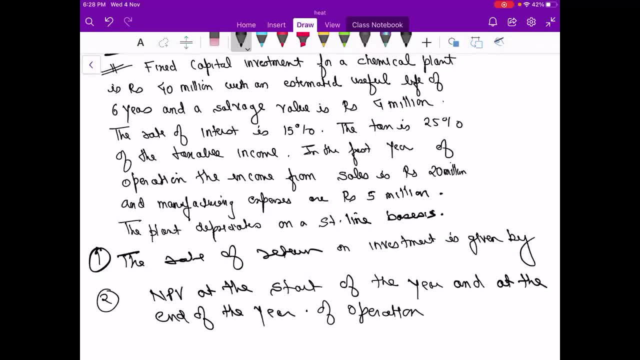 the rate of interest is 15 percent. the tax is 25 percent of the taxable income. in the first year operation the income from the sales is rupees 20 million and manufacturing expenses are 5 million. the plant depreciation on a straight line basis calculate the rate of return on investment is: 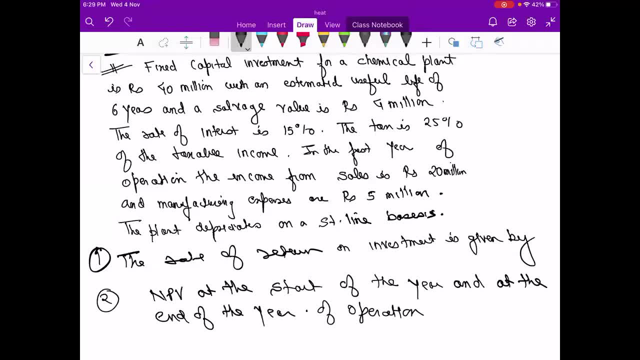 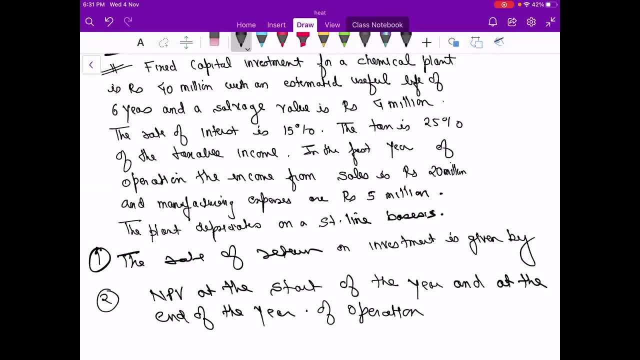 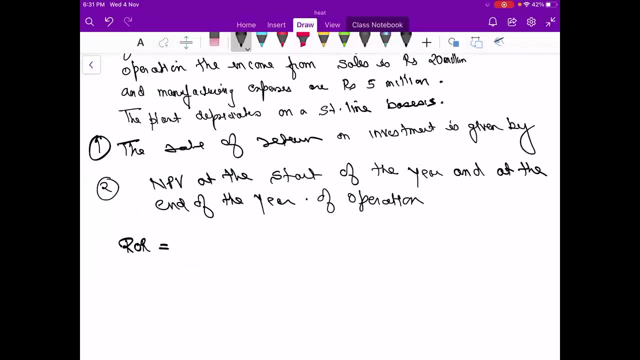 i think ror value. everyone has calculated correctly, almost everyone has given the correct answer of ror. so see, ror will be very simple. it will be 20 minus 5 upon 40 into 100. so how much it is coming? i think it is 37.5 percent. okay, and then, unless it, 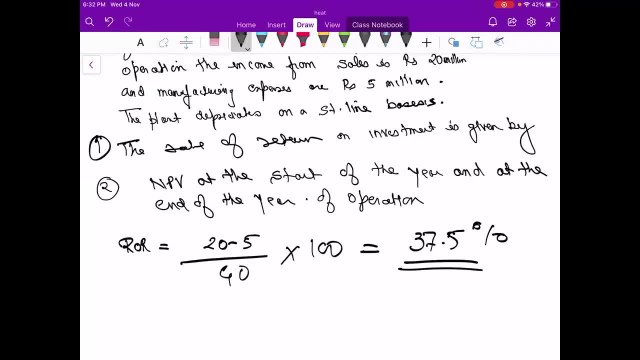 is not mentioned in the question that you have to calculate the profit after tax. you don't have to develop the tax money. okay, by default, every time the ror means the money or the profit which is before tax. okay, so this point you can write in your notes until. 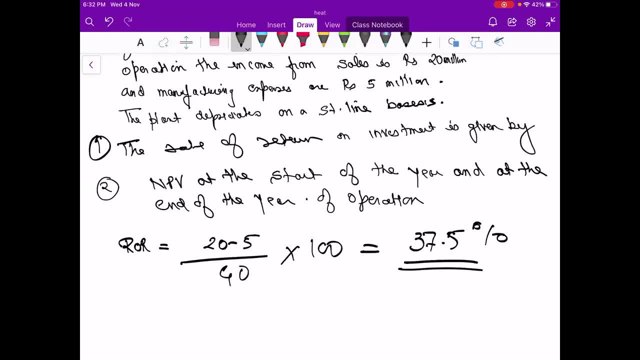 and unless it is not specified, 0000 the money or the profit which is before tax. okay, so this point you can write in your notes. until and unless it is not specified in the question, you have to always calculate the profit before tax if it is given in the question. 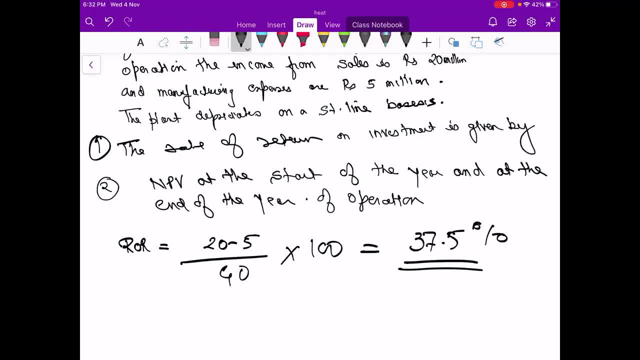 if it is given in the question, then you have to calculate profit after tax. okay, so this point you can remember, because someone say that, uh, from that profit, uh, we have to pay income tax. yes, we have to pay income tax, but by default, the profit for ror is without paying. 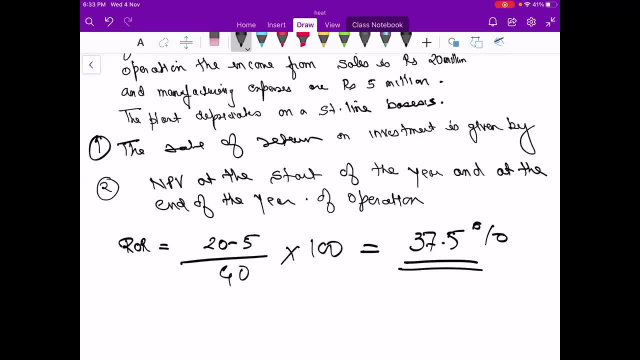 income tax. okay, you can write this by default for ror: the profit is without paying income tax. if it is mentioned in the question that you have to take profit after income tax, then you have to calculate that, okay. so in this question they have not mentioned anything, they have just written. 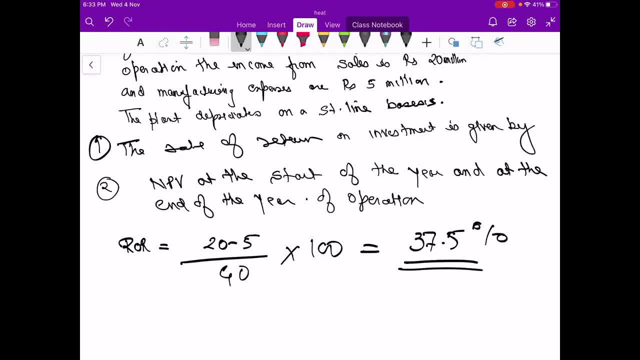 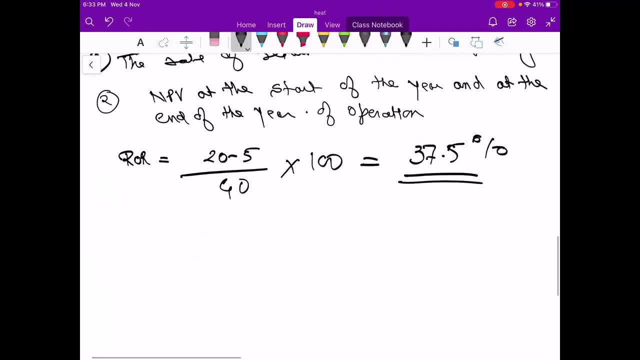 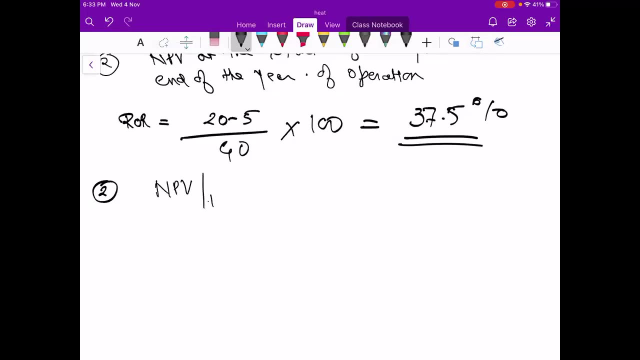 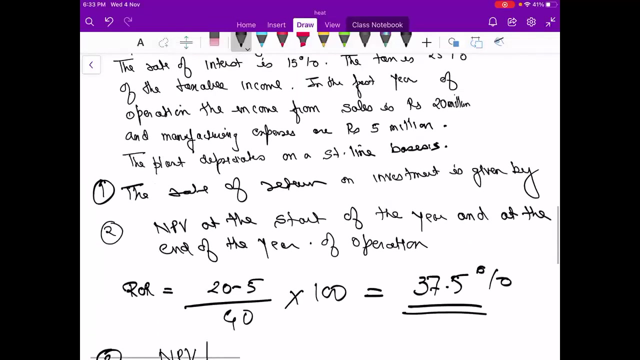 that, okay, they have just written that it is. the rate of return on investment is given by. okay. next second, they have asked the npv. okay, they have asked npv. at time t equals to zero. okay, so at time t equals to zero. you have invested a money. how much invested? how much money you have. 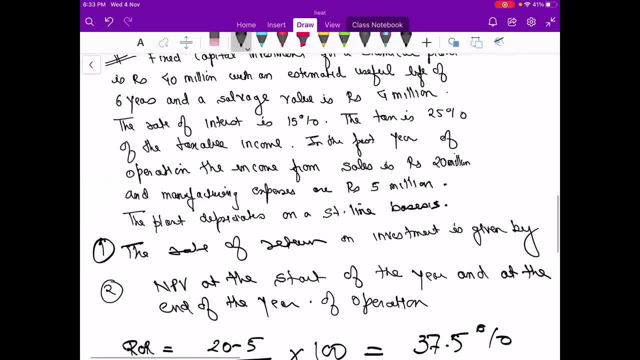 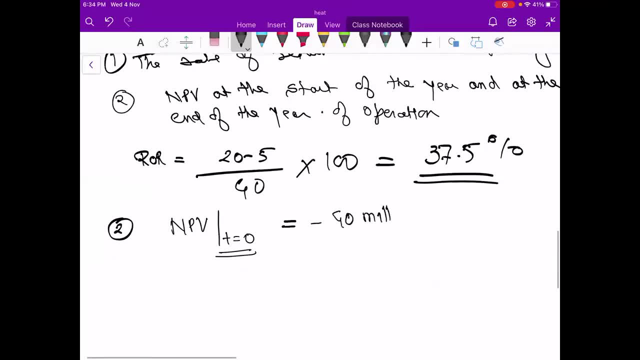 invested. it is 40 median. okay, so that is the rate of return on investment. so correct answer is minus 40 million for the first part. okay, then they have asked npv. at time t equals to one year. okay, this one year npv they have asked. so it will be minus 40 plus acf upon. 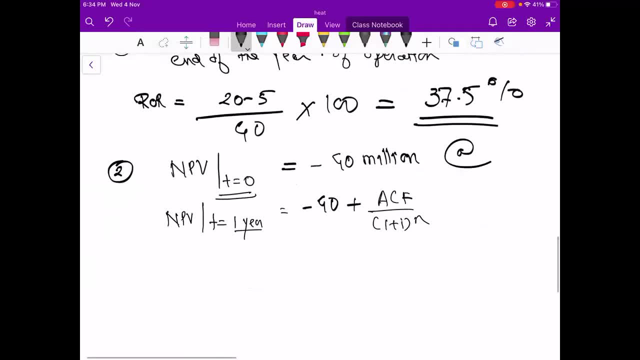 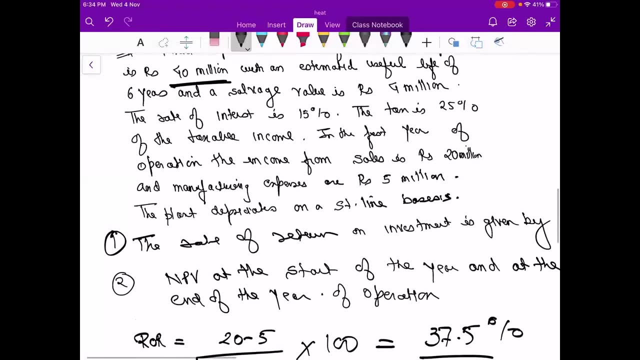 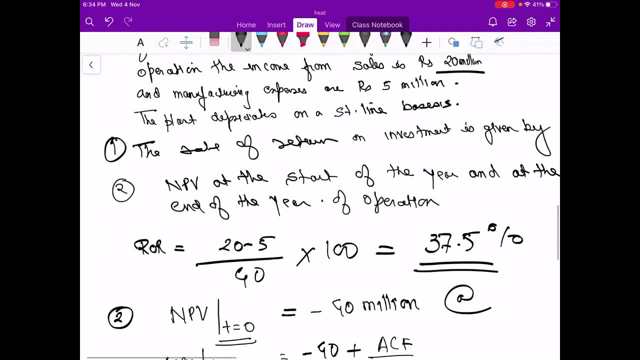 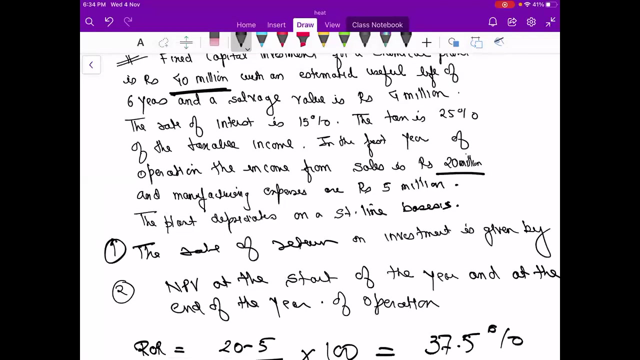 one plus i to the power n. so first you can calculate the value of acf. acf will be how much profit you are getting. your profit is where is profit? 20 million, okay, this is given 20 million. so 20 minus 5, minus depreciation. what is the depreciation amount here? tell me. 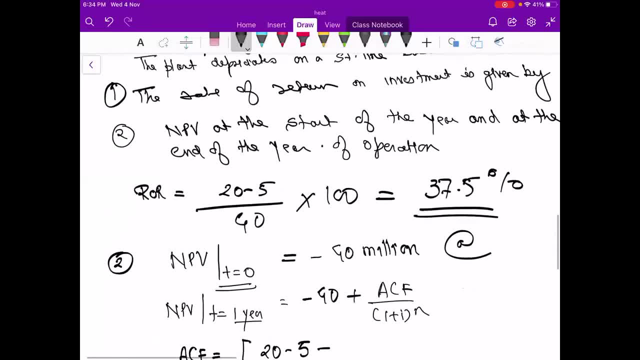 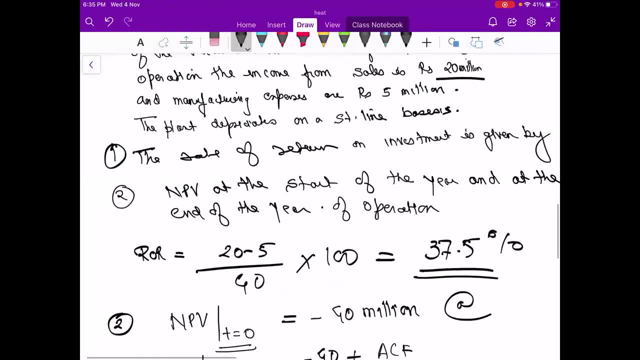 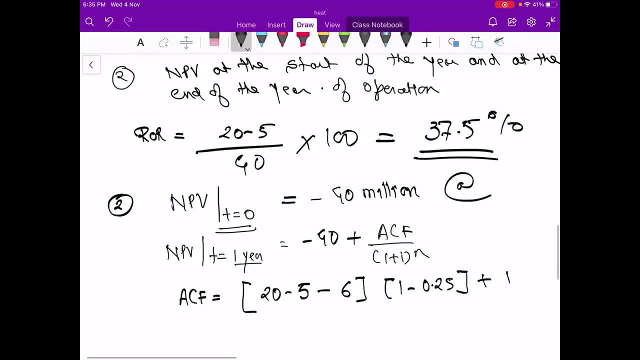 six. okay, so depreciation amount is six. okay, so it will be one minus five five. how much rate of income tax? it is 25, so 1 minus 0.25 plus d. okay, so it means plus six. okay. so how much acf is coming? yes, absolutely. 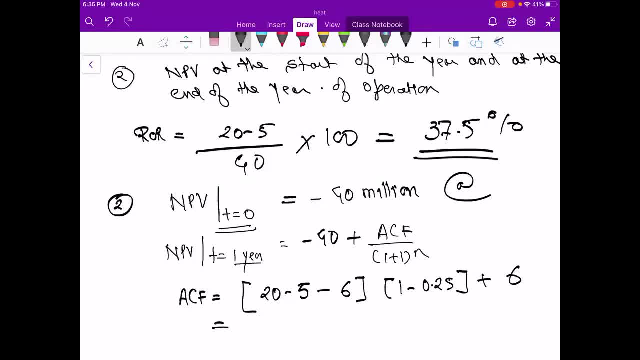 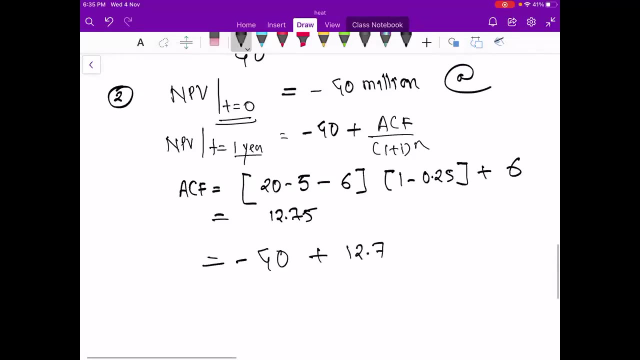 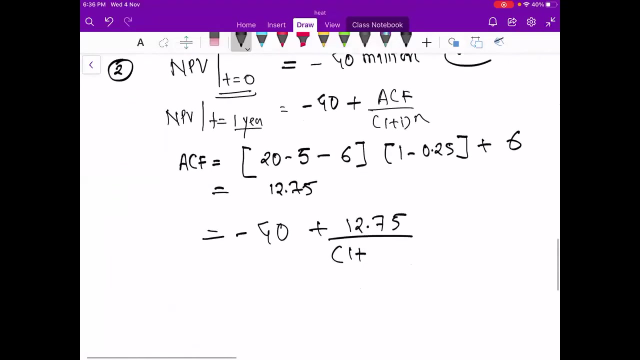 if you keep it up, you will be right in the bottom. you will announced: so the answer will be: minus mo 12.75. okay, so it is coming. 12.75. okay is rate of interest: 15 percent 0.15 to the power 1. that's it. so how much answer you are getting. 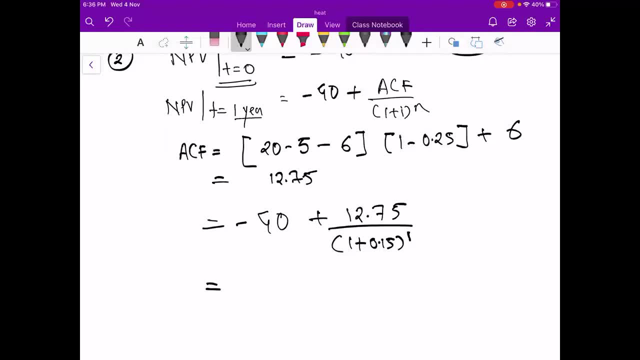 how much answer you are getting, minus 28.91. okay, so this is the correct value. see here, this 20 is the profit, but this is not the profit which is going in our pocket. okay, so that is why we have to calculate the value of acf. so you have to deduct the value of. 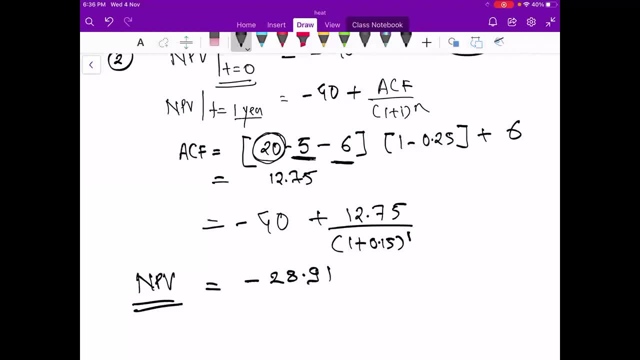 expenses minus, you have to deduct the deficit depreciation cost because the government says you don't have to pay the tax on depreciation amount. okay, so this you have neglected. again you have to add a depreciation cost because that cost of the equipment is your money. okay, so this is your actual wealth actually. 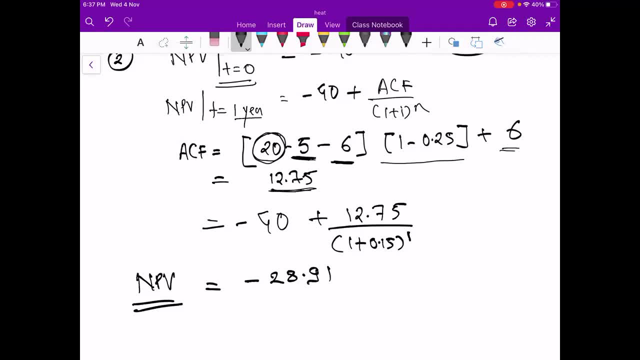 okay, so that is why it is coming 12.75 and you have to again solve like this: okay. okay, so the amount it comes in you have to subtract the receivables. okay, so you are adding that it is 19.98. okay, and you can take a matrix in that matrix. 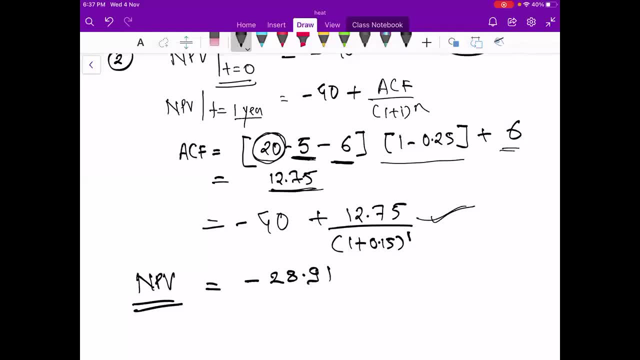 and you have to add a multiple factor meter. that's the life. that is OS for it. so basically it is. so let's change it into the variablezej and just try to catch that Detroit dot month. so, as you see here, this chemical is 19.97. okay, this is so. 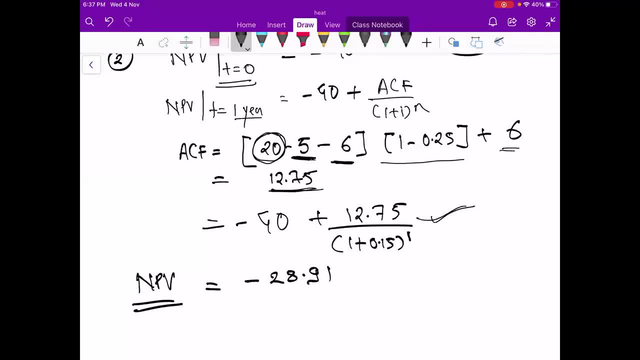 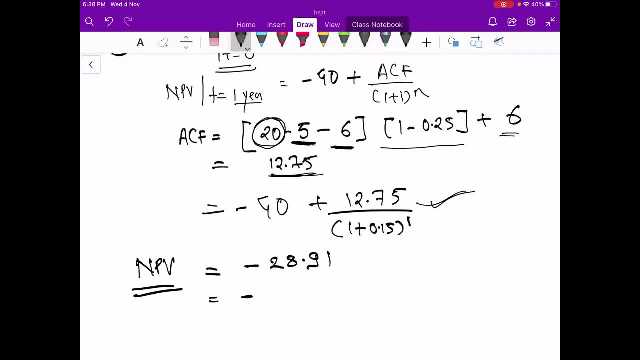 this, this: this is the JP profit I was given. I was given aे, but people were notсing 이 and roll number. what is your name, ranjan? you are telling that i have changed the formula of npv. okay, just see what is the formula. here i have used minus invested value. 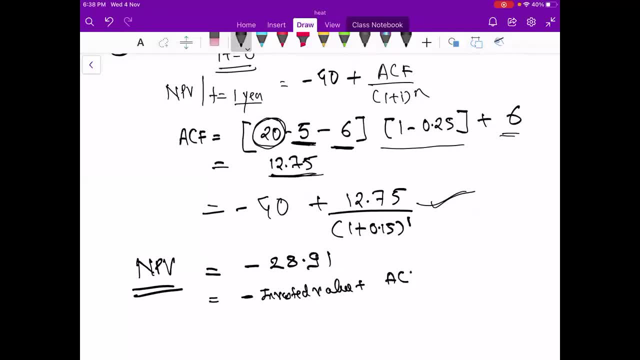 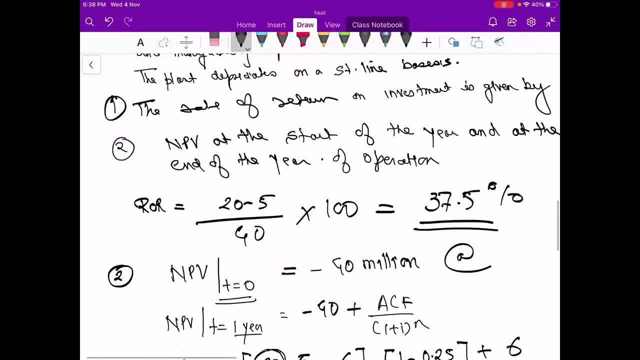 plus this is acf. okay, so if it is annuity, every year, you can just solve it like this. okay, you see here, one plus i to the power n. this is the formula i'm using. okay, this is the same formula which i have written here. what is the change here? 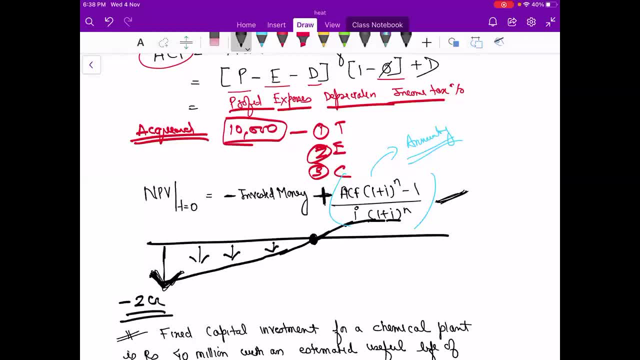 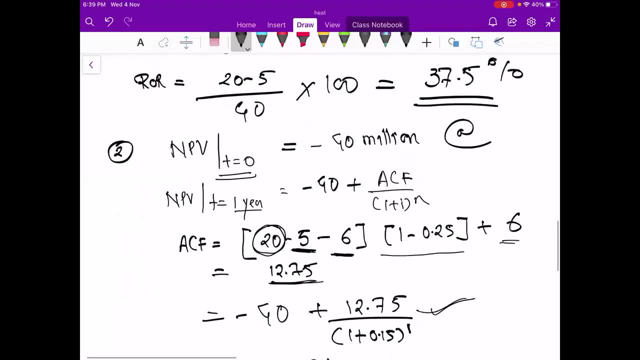 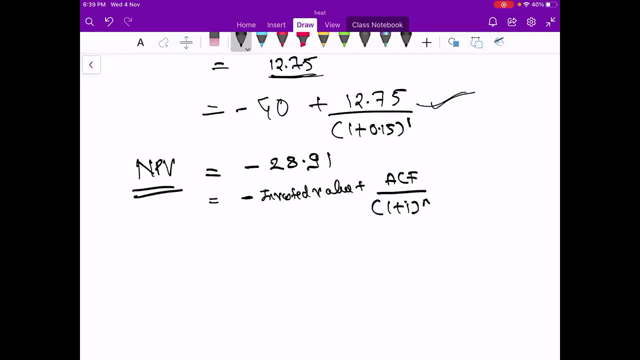 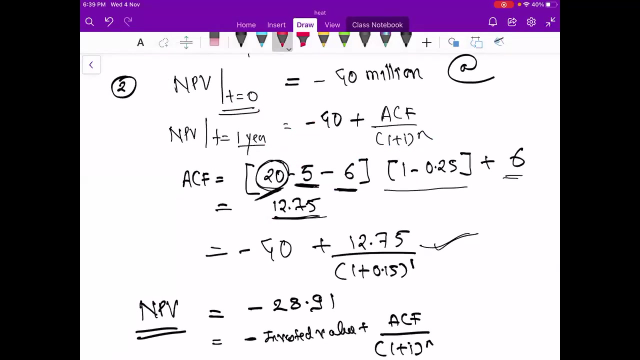 okay, ranjan. there is okay, sir, for ror we took profit as 20 and for acf we took only 15.. where i have taken 15, both 20, now both are 20. here also 20, here also 20. why, where i have changed, 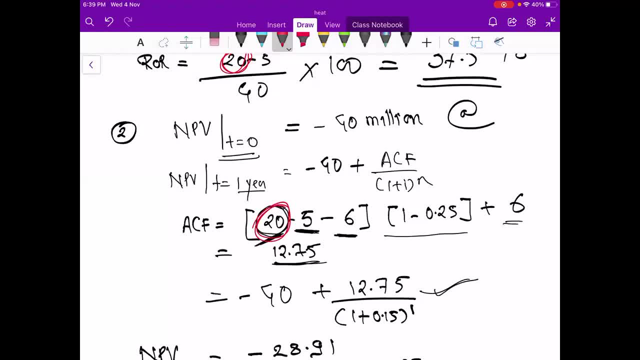 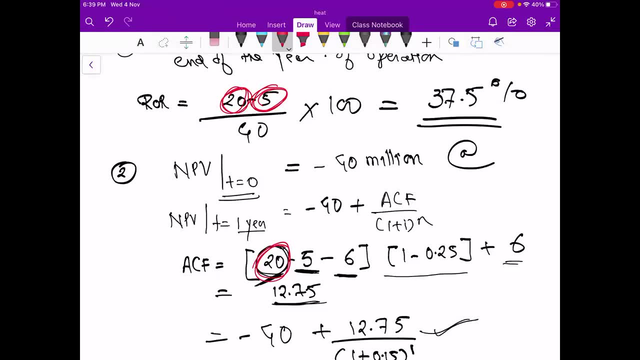 anurag gupta. why we will subtract 5? because it is expenses. now, expenses is not our profit, anurag. okay, expenses are not our profit. that is why we have to subtract it. okay, so in ror for the annual net profit. why we are not taking depreciation? because for ror we don't. 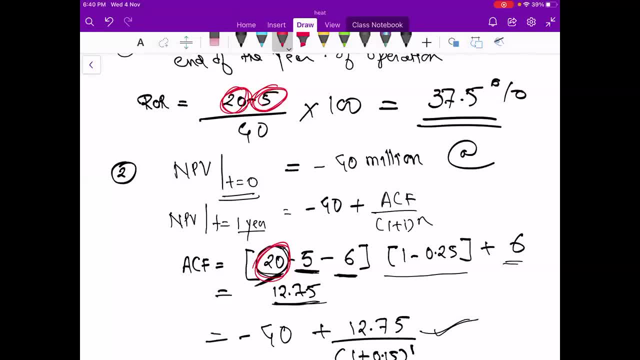 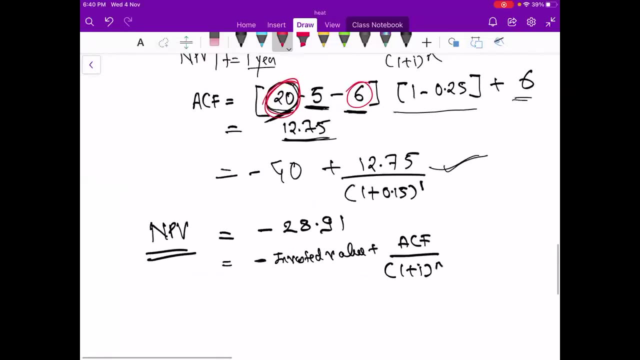 take the depreciation amount. okay, if we are taking depreciation amount, then what is the difference between the this, npv and all that? okay, every for every concept has different formula. okay, they have particular definitions. six students told me that it is six million depreciation. is it wrong? calculate it now very easy: how much. 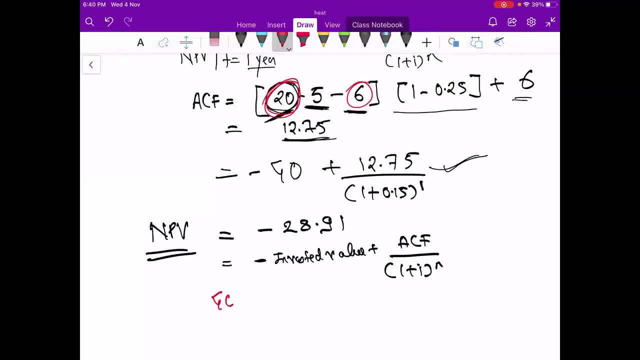 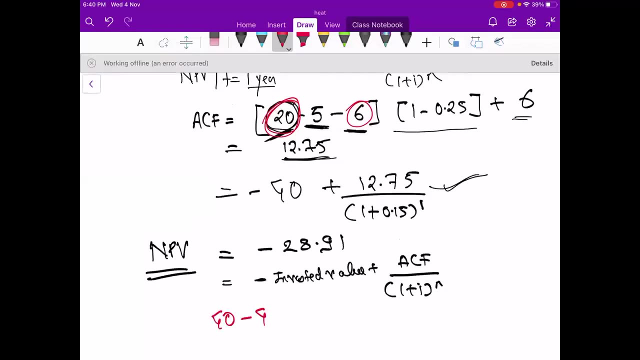 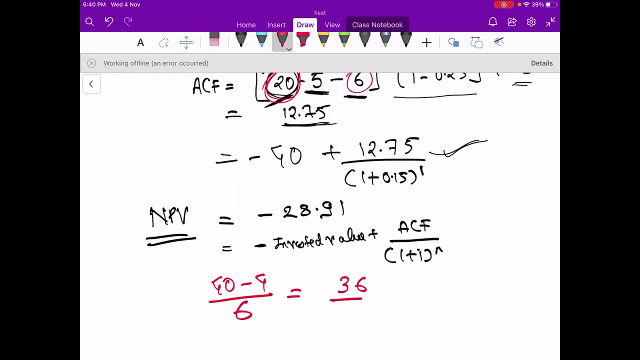 fixed capital investment is 40. what is this? what is the salvage value? and the salvage value is minus four. what is the live service life? what is the service life given six? so how much it is coming? 36 by six, six, one, just six, six, six are 36.. so d equals to six, okay. 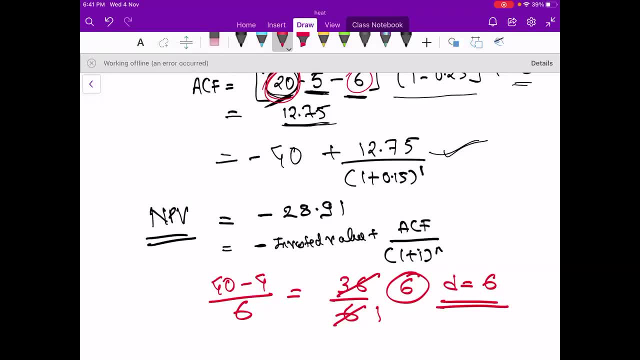 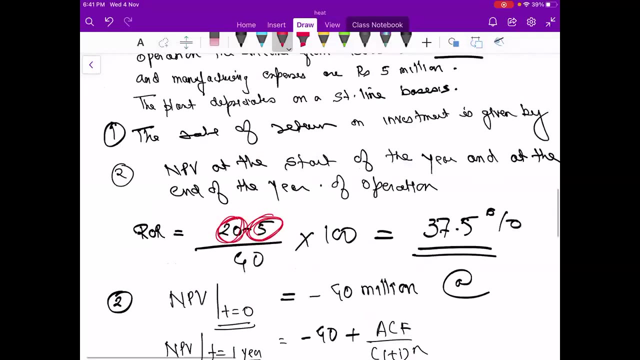 in this question we are focusing npv, okay. so that's why i have not written the detail step for depreciation. this is very easy enough, arnab agrawal. sir, in question it is end of year operation to six year. it is mentioned in the question uh, npv at the start of the year and the end of the year of okay, okay, sorry, sorry. 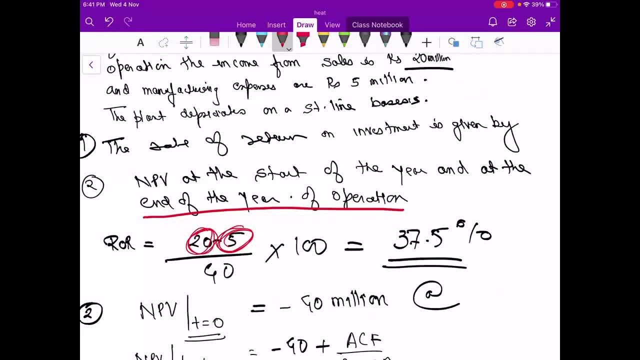 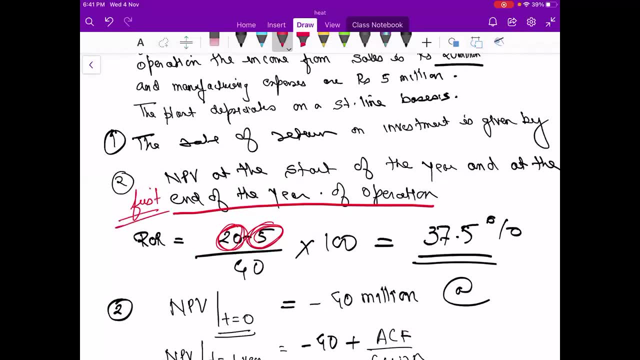 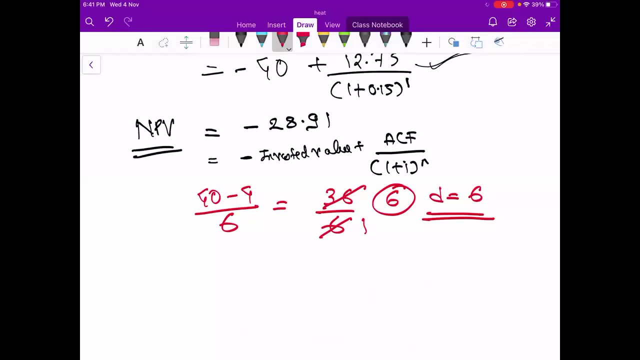 sorry, okay, okay, end of the year. operation is being given. okay, it is. uh, i have calculated, assuming it as a first year. okay, fine, fine, okay, okay. so if you calculate for the sixth year, we can calculate. okay, so this is npv. i i told here actually this is t equals to one year, okay, 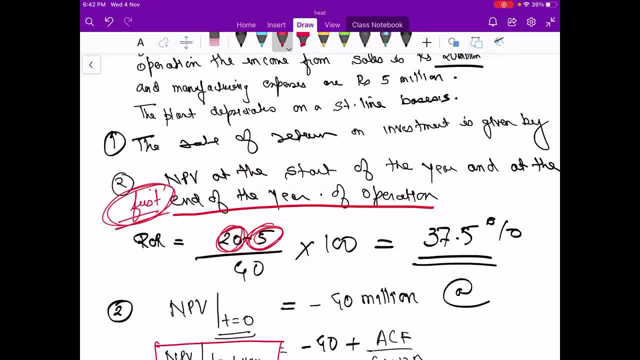 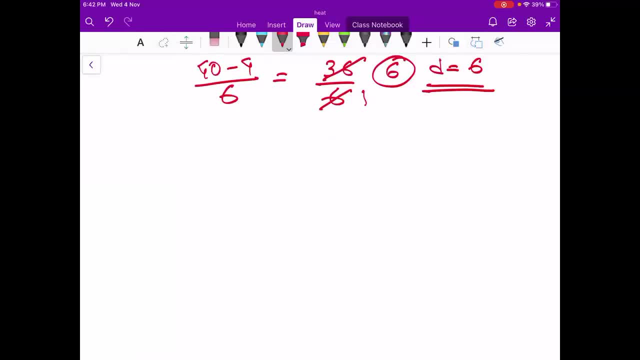 i have mentioned here. i have forward to mention this is first year. okay, actually it is end of the first year of operation. okay, yes, the question, actual meaning, is you have to calculate at the end of the sixth year. so then what will be the formula? solve it? 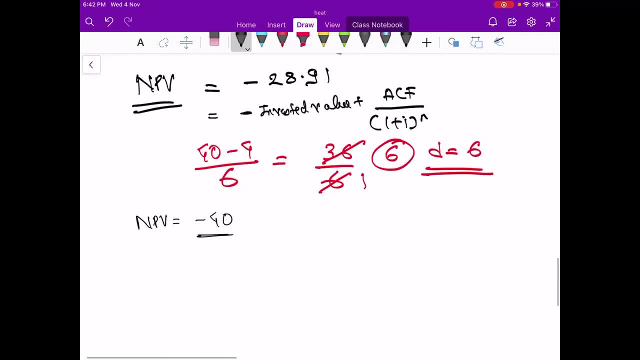 npv equals to minus 40, y minus because this money is going from our pocket. okay, so that is our minus plus acf, 1 plus i to the power n, minus 1 upon i, 1 plus i to the power n, so it will be minus 40. 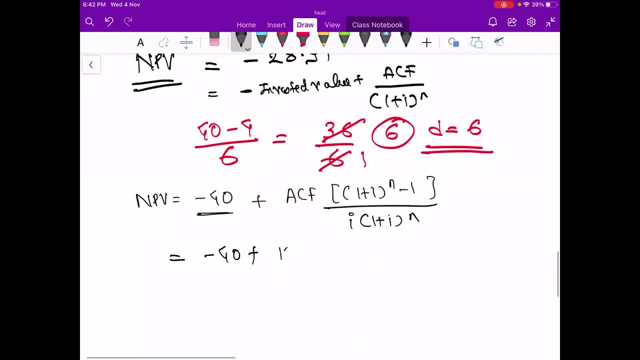 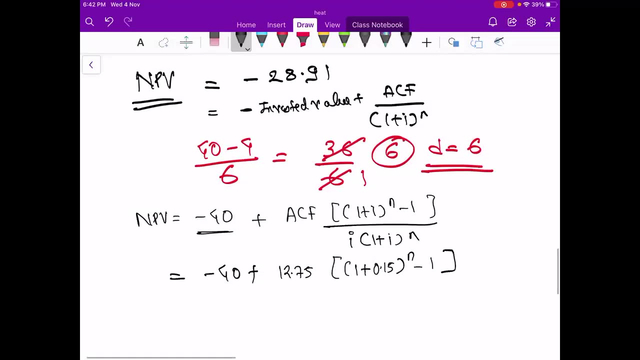 how much acf. we have calculated 12.75. 1 plus i. how much i value is coming means how much i value is given 0.15, 0.15 to the power. n minus 1- okay upon 0.15. 1 plus 0.15- okay to the power. all are 6. this is 6. calculate it how much you are getting. 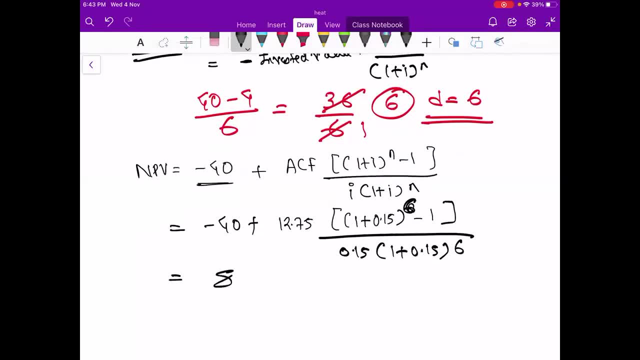 8.25 billion, okay, million, okay, calculate it. is it right or wrong? 8.25 million: okay, so this is the npb. so where npb is this? this is at t equals to 6 here. okay, yeah, samitwa survives, profit 20 and expenses 5.. it is given question. read the portion, see. 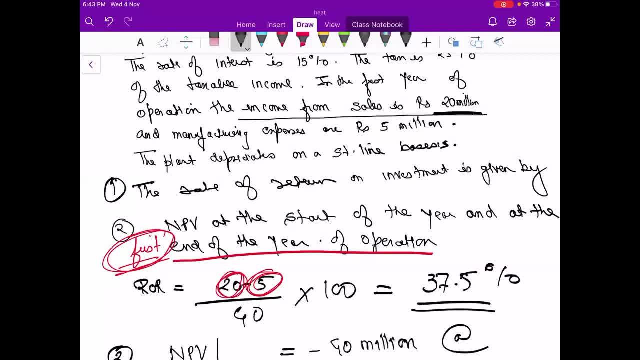 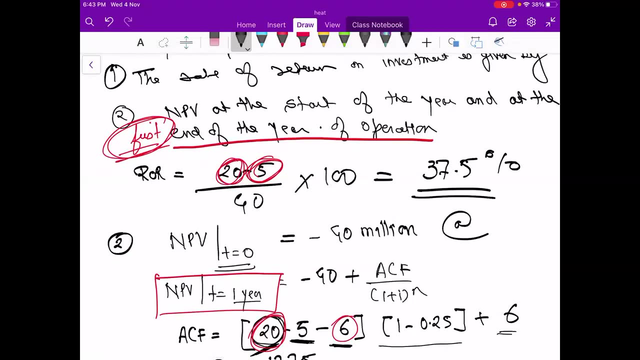 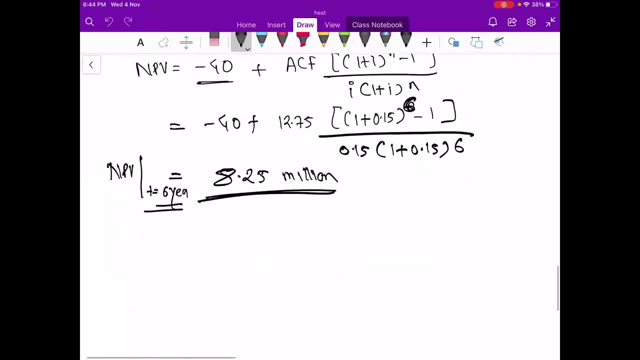 20 million, the income from sale is 20 million and the manufacturing expenses are 5 million. they are mentioned in the portion samitwa okay, where you are not taking depreciation roll number: double two, double zero, three, four. what is your doubt in the ro are you are saying: 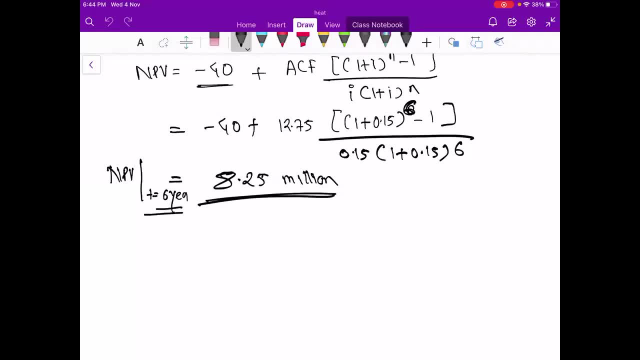 yeah, that is the formula for war. that's why i told now ror will see rate of return in bank. suppose you are getting some interest, okay, so in that you take the amount of depreciation, you don't take care of that depreciation in that, okay. so r of is rate of return, so in rate of return we don't consider the depreciation formula. 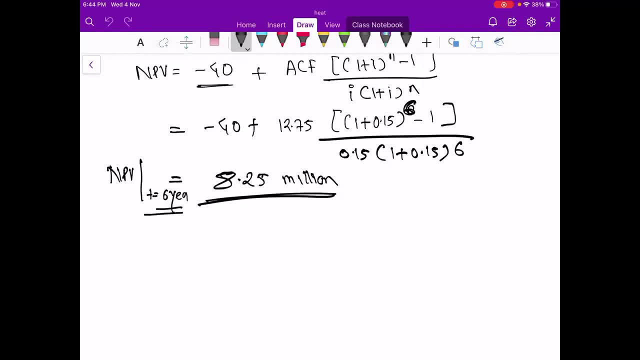 so last day in ror the formula in that 10 legs on a problem, the formula was reverse. no, it is not reverse. now we have calculated 1.5 lakh per year. how much invested money? 10 lakh. okay, two double one, three, eight, two. yes, there is no depreciation in the ror. this is the government. 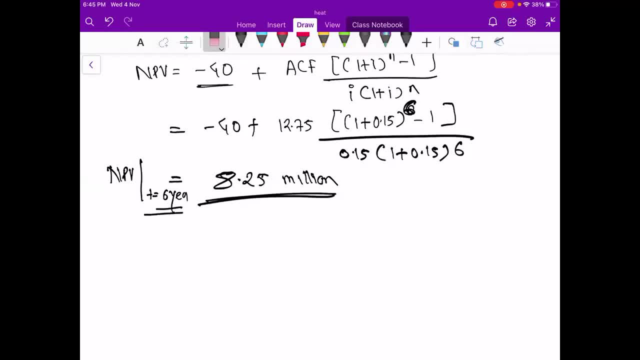 rules. now we can't say in this, okay, this is a government rule- that in ROR we don't have to consider depreciation. this is just a rate of return. if you, you can ask your father, okay, where you you have invested money- suppose in bank or anywhere else, you will not calculate depreciation amount there. okay, because ROR means 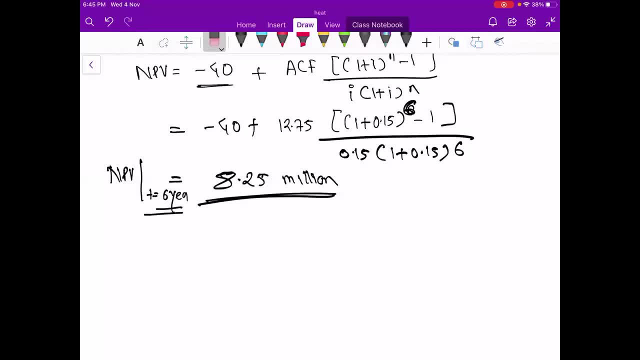 whatever you have invested, that is the rate of return. we generally, in our home also, in every home, we invest money in the bank. so that is certain amount of ROR for that, okay. so that is the thing. okay, you can ask in your home also. so basically means: whatever is the profit, is that we? 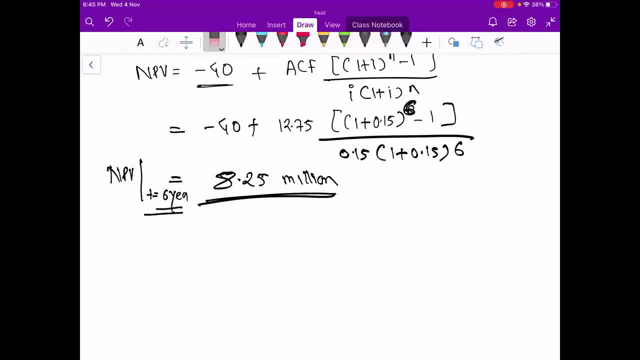 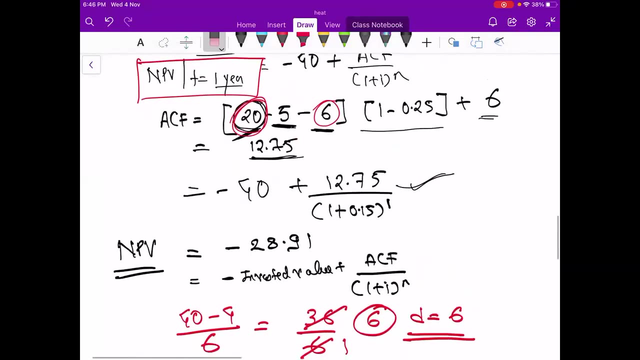 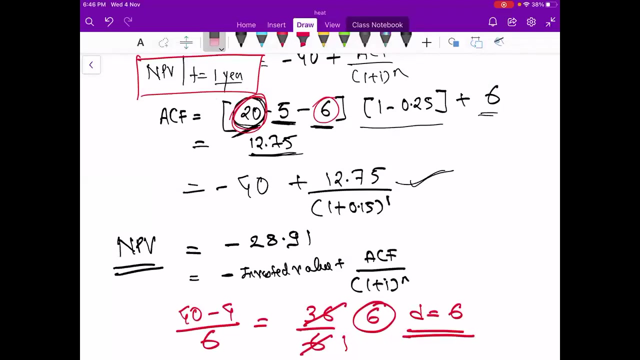 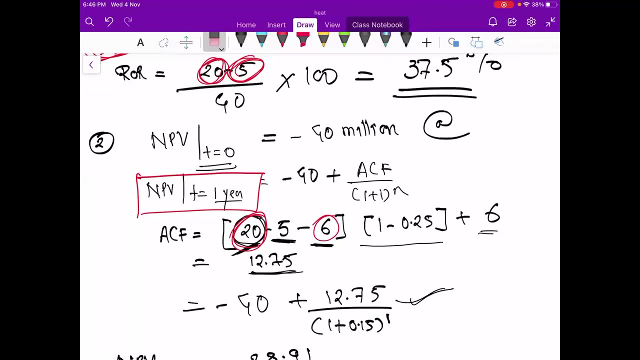 just subtract the expenses from that. okay, what you want to explain: 220084. what is your doubt? NPV formula for first year. yeah, we have calculated NPV for the first year. this is for first year, ACF part. okay, where is ACF? this is ACF part. yes, 20 minus 5 minus 6. 1 minus 0.25 plus 6. what is the? 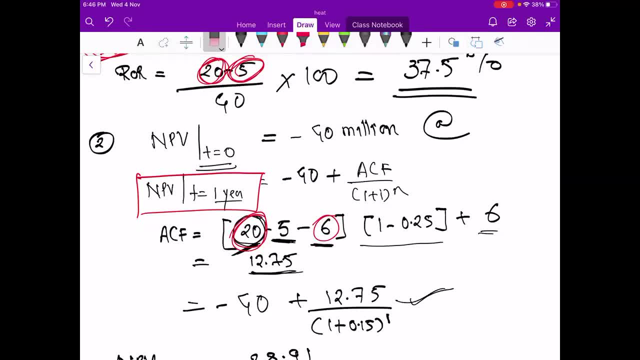 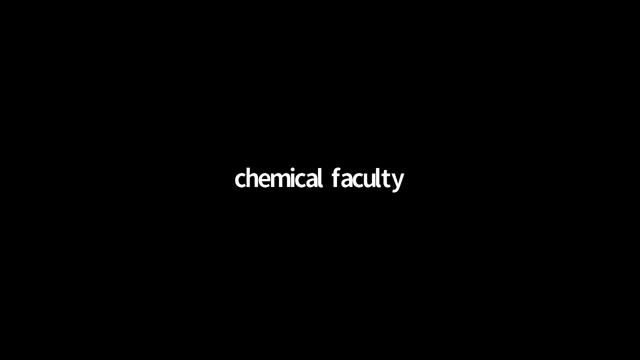 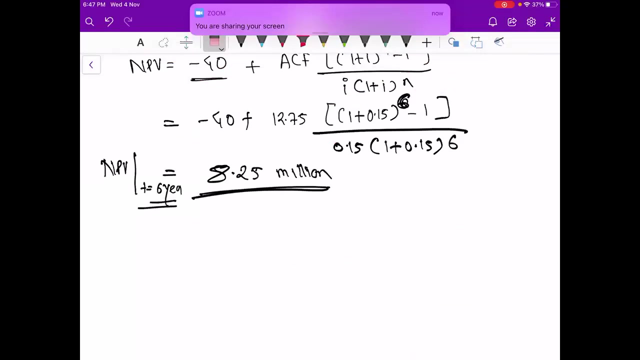 doubt here. ok, rebyting is a very good idea, if we just know it from this table: 15 milj wieder w isto. 14, 25, 27, 28, 30, 31, 46, 35. Yes, we can apply the ACF formula and annuality only when the ACF is same. 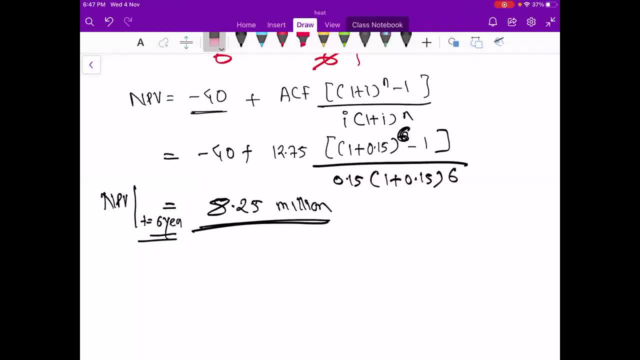 ACF can be different because here we are using a straight line method. If you don't use a straight line method, ACF of first year is equals to ACF of second year. equals to ACF of nth year is only for straight line method. 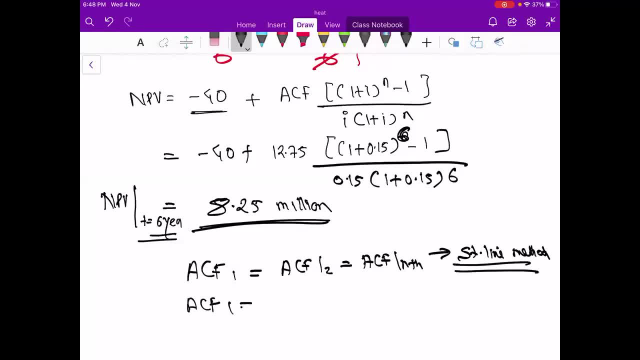 Other than straight line method. ACF of one is not equals to ACF of two, is not equals to ACF of nth year, Because for straight line method only the D value is same. We have calculated D from every method, So we have seen that ACF is different for different methods. 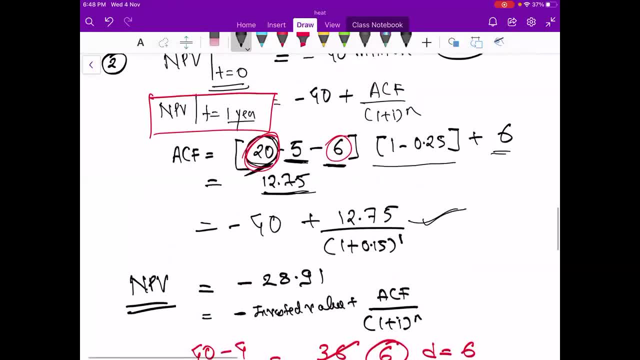 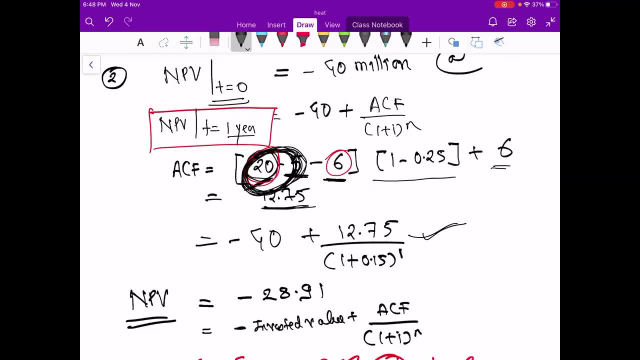 Naveen Kumar in ACF. I have taken 20 minus 3.. I have taken 20 minus 3.. I have taken 20 minus 5C, Where I have written directly 20.. It is 20 minus. We have taken 20 minus 5.. 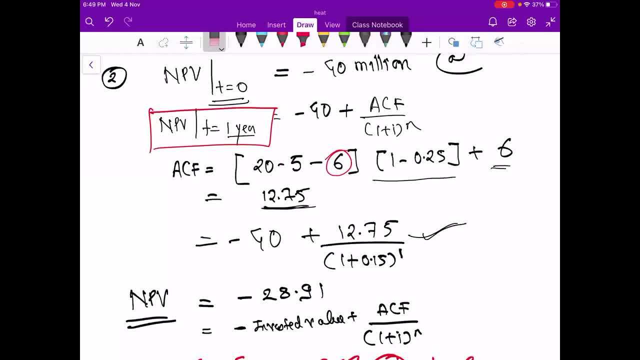 Where I have written directly: Naveen, double two, double zero eight four. you use it general formula. okay, you calculate it from the general formula and tell me the answer how you will subtract two times minus five, expenses will be only one time. so say here: 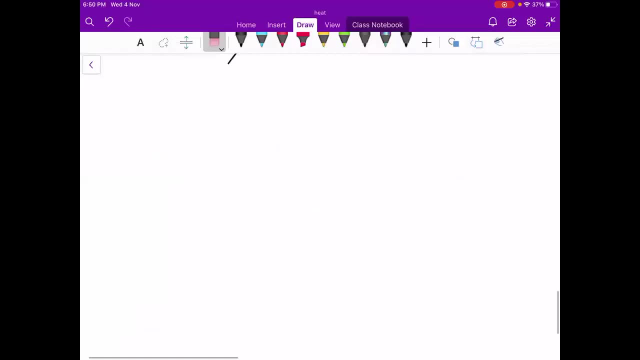 in? r? o? r. we have to take the profit after subtracting the expenses. so what is that twenty minus five? okay, twenty minus five. this is the profit actual. in acf it is twenty minus five. twenty minus five minus six, that is depreciation. that's it why you are confusing, why you are saying, why you will write twenty minus five, minus five. 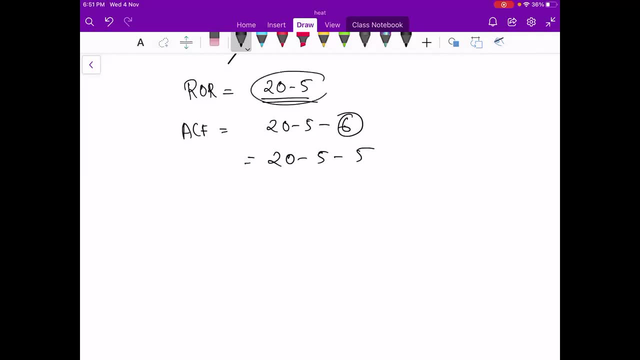 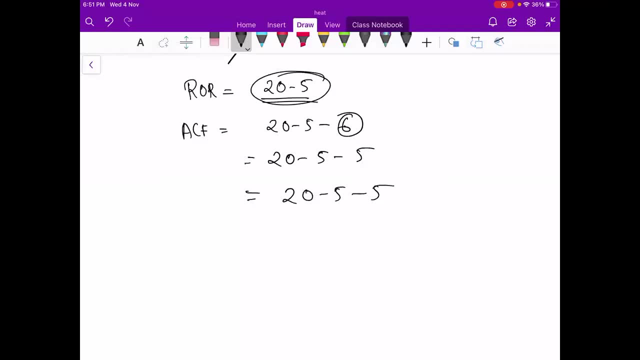 okay, so you will have to pay the taxes and all that. why you are confusing in this twenty minus five minus five how this will come. just use some common sense now. okay, so you will have to pay the taxes and all that. why you are confusing in this twenty minus five minus five how this will come. just use some common sense now why i will subtract two times minus five. 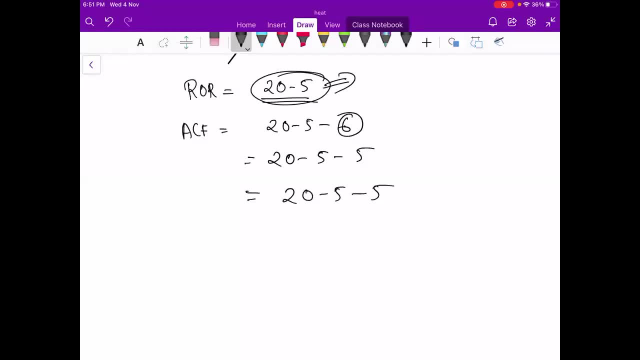 okay, so you will have to pay the taxes and all that. why you are confusing in this twenty minus five minus five, how this will come. just use some common sense now. why i will subtract two times minus five. here i'm using the word profit after expenses. here i'm using the word acf. both are different but this is the twenty. what is twenty representing? twenty is representing the money which is coming in your pocket. okay means the money which you are getting it from that you have to pay the expenses. that is, you have to just subtract it. why you are saying that it will be twenty minus five minus five. why you will do two times subtraction. 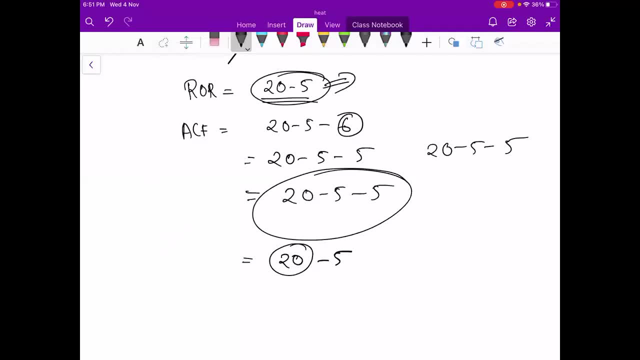 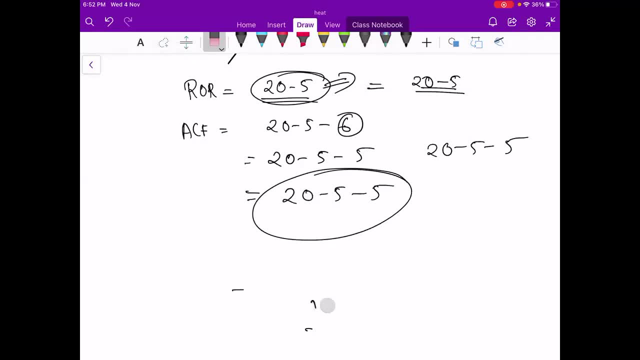 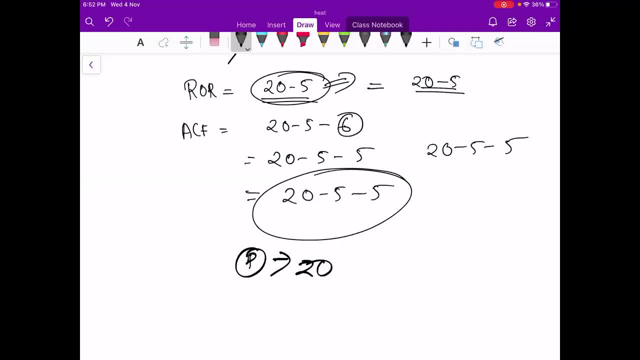 anyone has doubt can ask. okay, clear, you're all doubt, it's okay. okay, you are getting and confusing it, it's okay. anyone has doubt? ask. 66.6 percent on a last day, sir, 1.5 by 10. i'm not getting something to what you are asking. 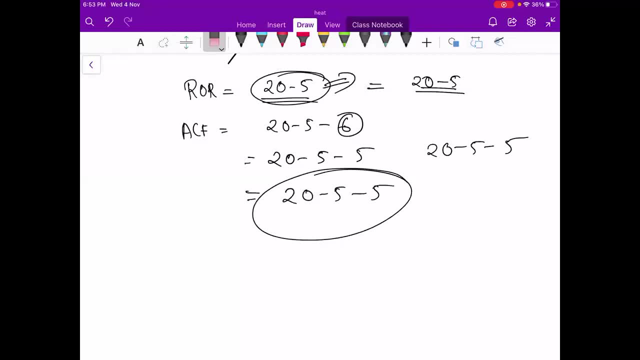 why is income from sales here denoted as profit? i just told it is a denotion. okay, don't confuse with the words. okay, don't confuse with that words if these are just notations. okay, see, you have. uh, you have done with the pdc. in pdc, if there are some students are with, you will see a means area also and a is amplitude also. 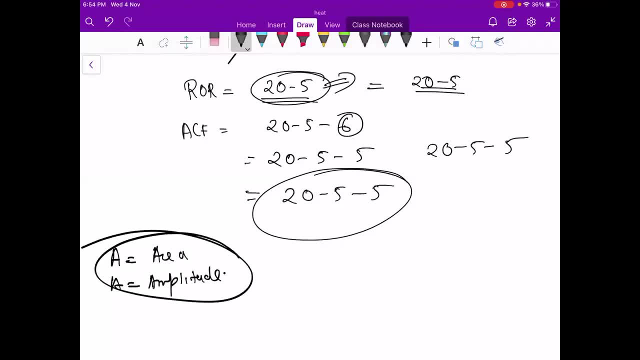 those who are in final year. they can understand: a is area also and a is amplitude also, but both have different meaning, okay. so in this same way, don't go with the wordings. okay, see what i'm telling? that? what is the actual meaning? this p is actually the money. 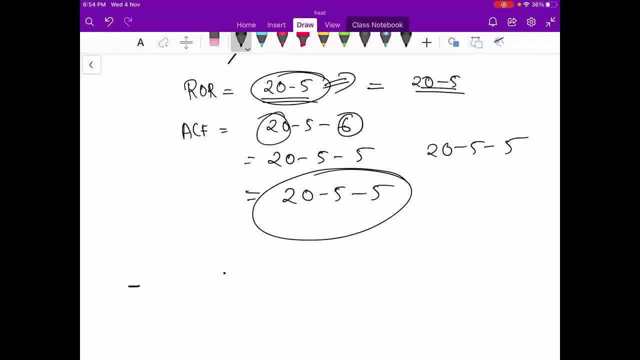 okay, this is the money which you are getting after selling. okay, is that your grant, would you? and therefore you should be able to pay the final amount. what are you appear to? again, broken mean in the meaning. i told you i'm also one of my students. um, i think that is very interesting, okay, um, so let's get somePass, etc. 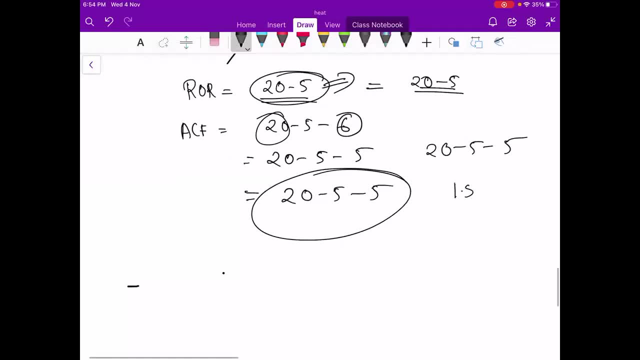 we came to the second step and the last saints. yeah, uh some, with your last problem we have done. it is, i think what i remember is 1.5 lakh per year is our profit upon 10. this we have done. i think you are asking same. 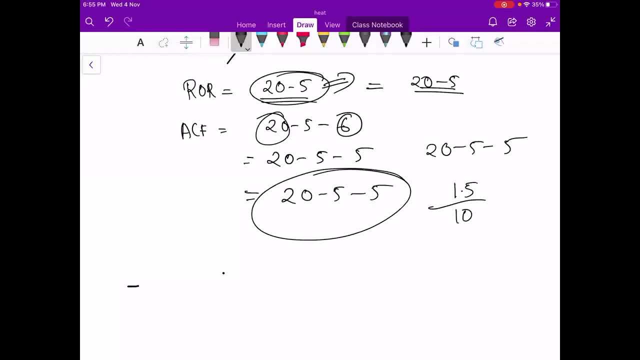 I think you are asking the same, Okay. Yeah, I think you have written wrong answer. Okay, So anyone has another doubt can ask. Just clear all doubts. Okay, That is important. Any other doubt to anyone related to NPV, ROR and anything else. 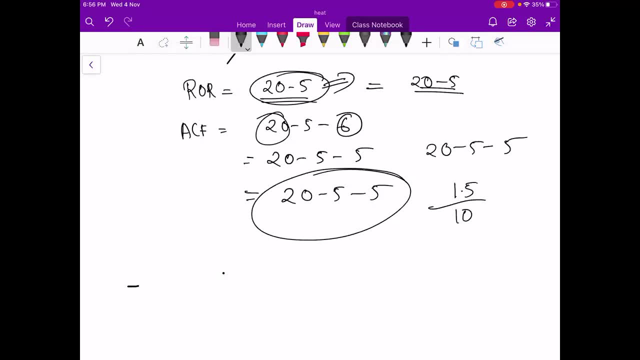 Okay, Everyone is clear. Anyone has any doubt can ask now. Okay, Anyone has any doubt? Ask or yes or no. at least Samajh mein aaya ki nahi aaya Bolo haan ki na. Please reply. Only some selected students are giving reply. Okay, Please reply If anyone. 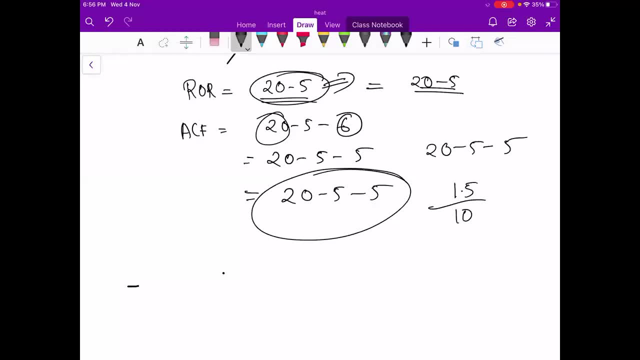 has any doubt can ask: Okay, So that we will move forward. then Which term to subtract Numerator for ROR if it is given to calculate after paying tax? Okay, I will. Okay, So doubt is in ROR. Okay, So doubt is in ROR. you have to calculate. first thing is that 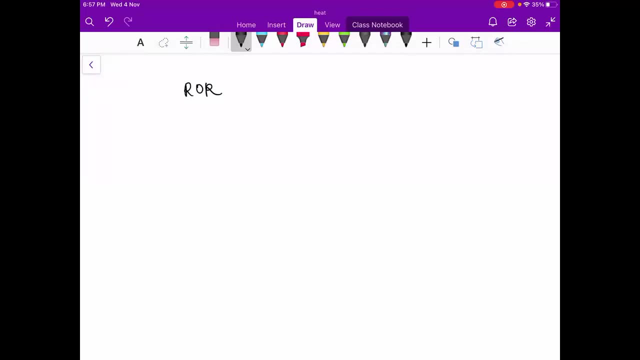 99%. ninety in ROR and you don't subtract income tax. Okay, If that's given to calculate the tax, then use ACF. Okay, then use ACF upon denominator will be same total investment into 100.. Okay, but this is not used in practical life. Okay, this formula is not used in practical life. 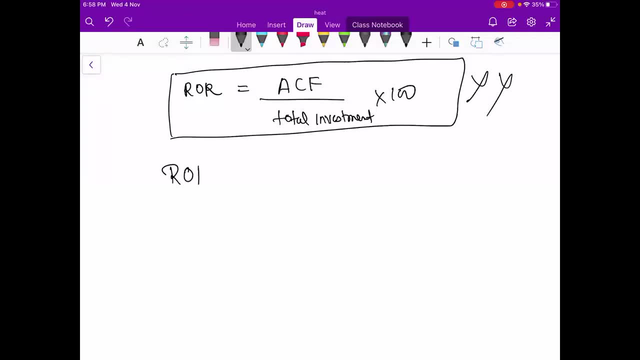 Okay, ROR means in the industry or in the bank, in the today's bank, or you can ask to anyone, okay, you can ask your father, okay, anyone who is investing money in ROR. we don't consider. we don't consider after giving tax, we don't consider the money after giving tax. 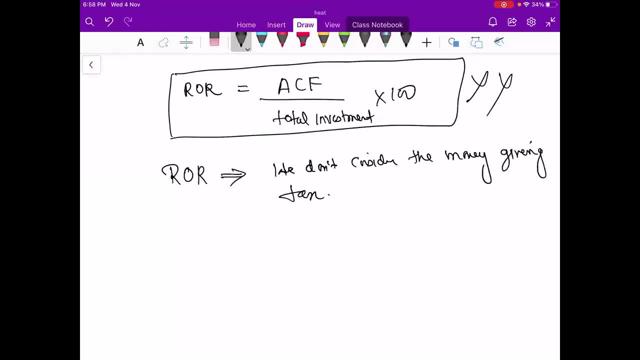 Okay, Now everyone is confirmed. What is your doubt? 211382? ROR. Okay, everyone understood or not understood. So money is not a function of time in ROR. Yes, you can Say. Okay, How ROR is used. 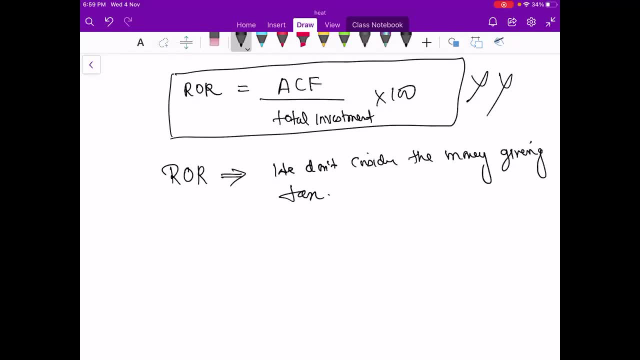 ROR is just a technique, that how much return you are getting. it is the significance is that the money which you have invested- okay, the money in which you have invested in the system or in any bank system or any other way. So what is the rate? 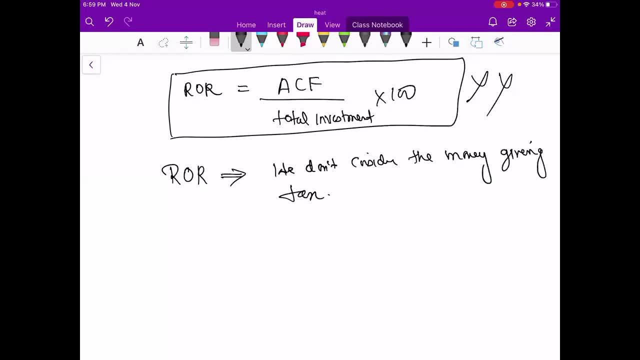 ROR is the rate of return. Okay, so this is the only thing. It is the rate of return. Okay, so this is the only thing. It is the rate of return. Internal rate of return is just a terminologist which we use in the banking system. 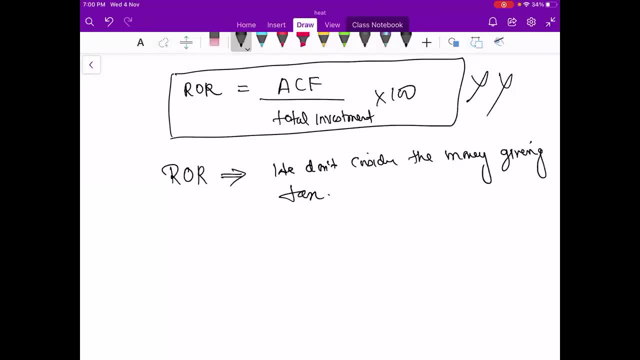 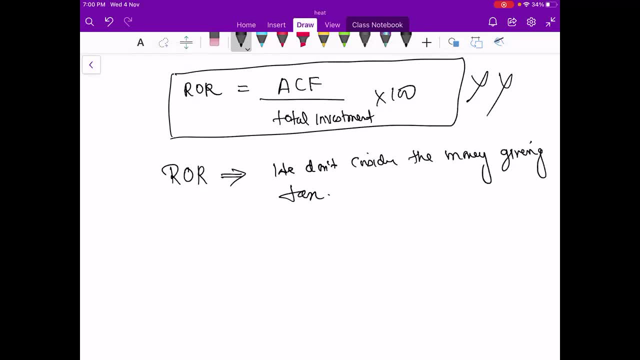 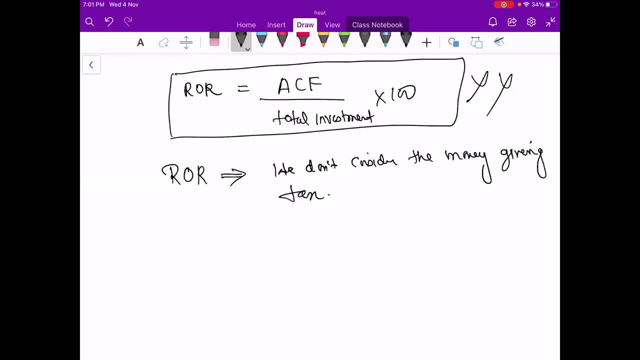 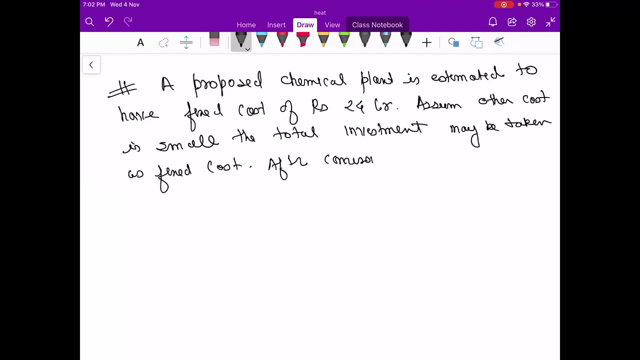 so write that question. a proposed chemical plant is estimated to have fixed cost of rupees 24 crore. assume other cost is small and the total investment may be taken as fixed cost after commissioning at t equals to zero year and annual profit before tax equals to. 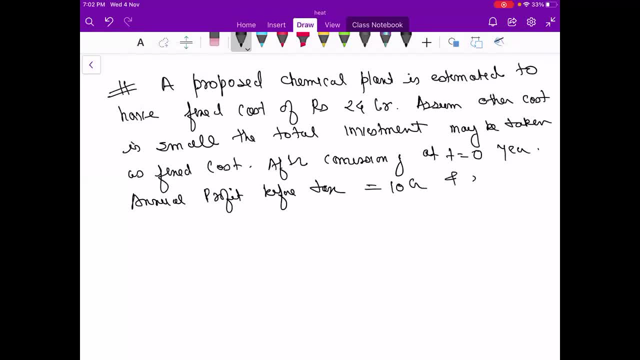 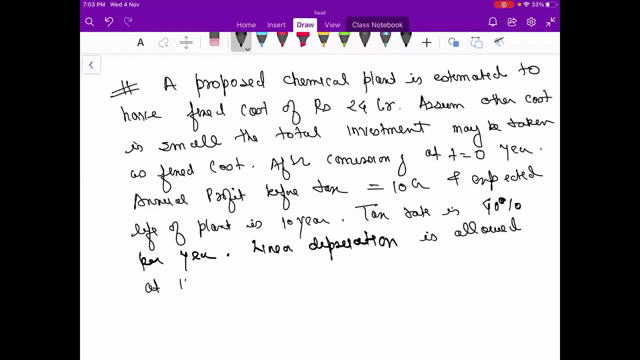 10 crores and expected life of plant is 10 year. tax rate is. tax rate is. you can take 40%- 40% per year. linear depreciation: linear depreciation is allowed in the annual rate of interest at 10% per year. if annual rate of interest. 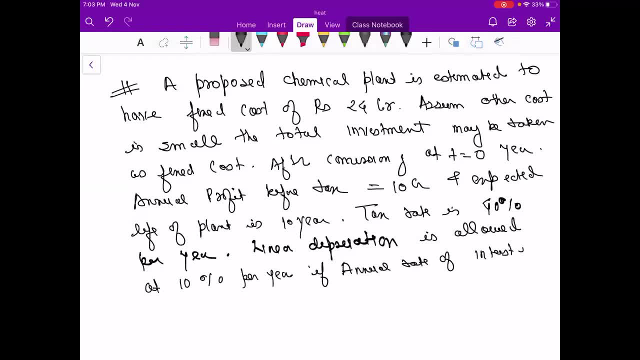 if annual rate of interest is 12%. calculate the NPV of the plant. calculate the NPV of the plant. calculate the NPV of the plant, every plant, the NPV size, the equivalent table version, the middle row industry area. we we define a narrow sub. 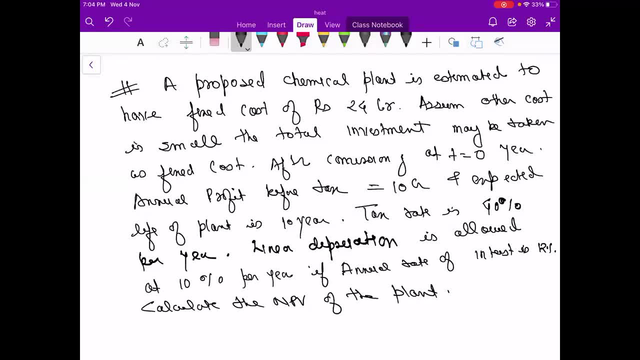 range of fewer value- cent Its- you can. If it is not mentioned, calculate NPV of the plant means you have to take care of all the failures. Anurag Gupta, perpetuity means indefinite time. NVTE for indefinite time. Total Invest, Samvitva, you are correct. 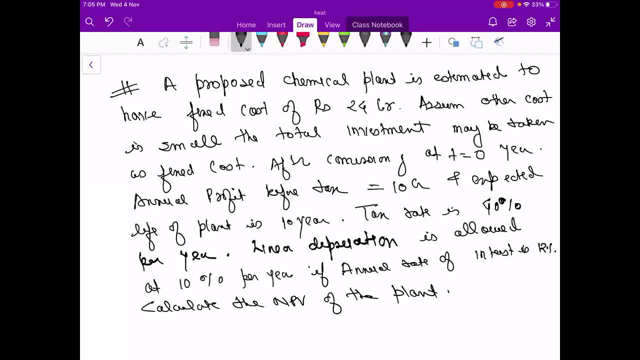 Just read the question properly: 211094, 220083, interest is the amount. Okay, It is used for banking system, specifically Okay, Rate of return. you can apply for any business. 220034, basically, it is the profit, Okay. 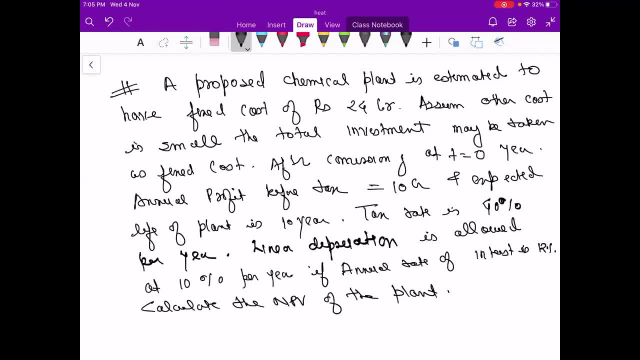 After selling the products. So let us see the question. So I hope I have given all the answers. So solve it. A proposed chemical plant is estimated to have fixed cost of rupees 24 crore. Assume other cost is small. 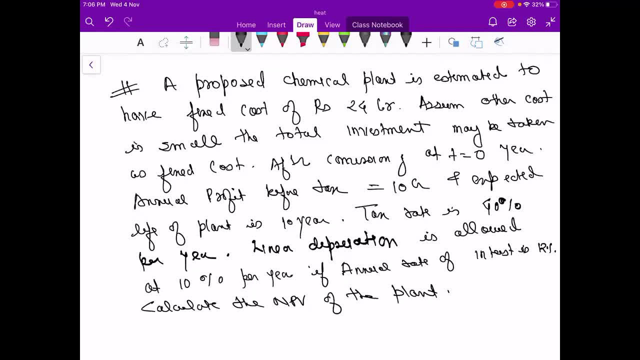 A total investment will be taken as fixed cost. cost after commissioning at time t equals to zero year. annual profit before tax is 10 crore and the expected life of plant is 10 years. the tax rate is 40 percent per year. linear depreciation is allowed as 10 percent per year. annual rate of interest is 12 percent. 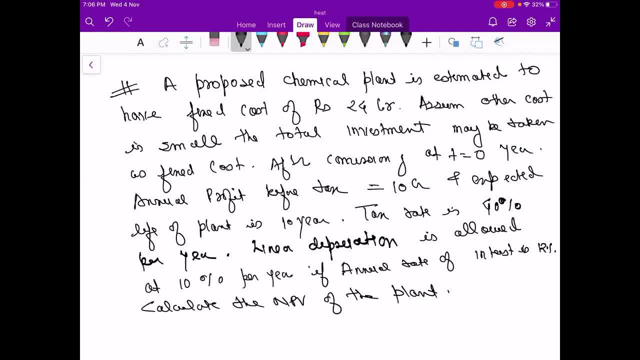 okay, calculate the npb of the plan. so you will see what is the answer. just solve that question. so solve it, so so you will see what is the answer. okay, so have a patience, let's everybody solve the question. so so, all solve. so some are getting nine answers, some are getting 50. 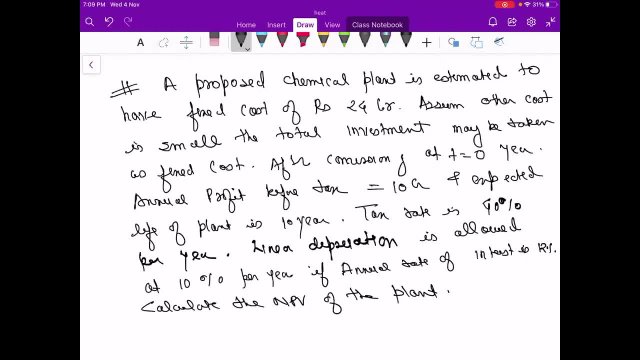 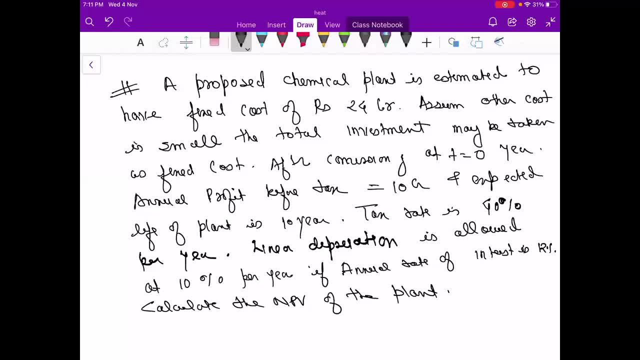 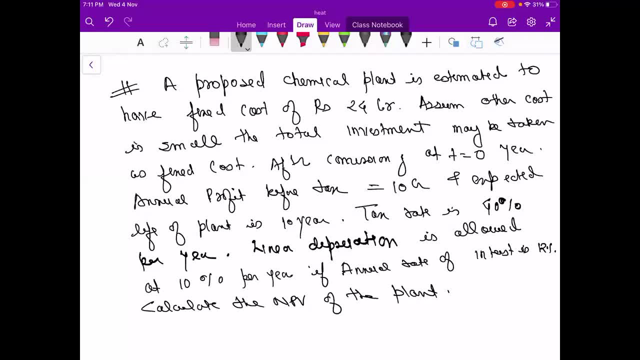 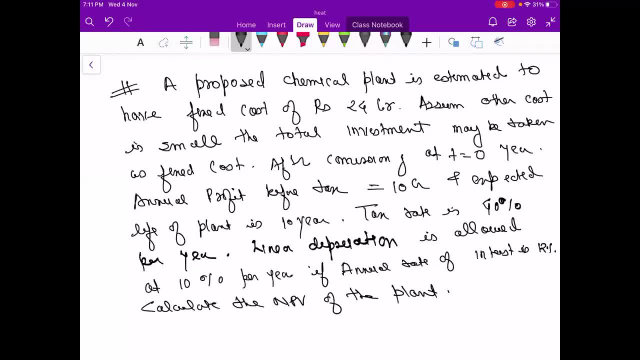 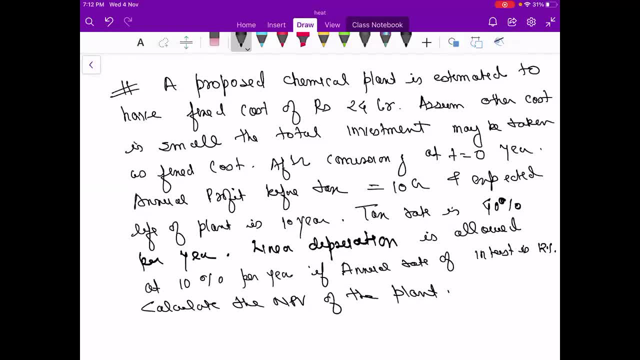 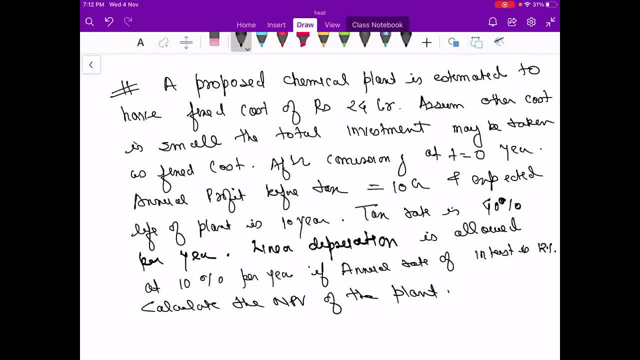 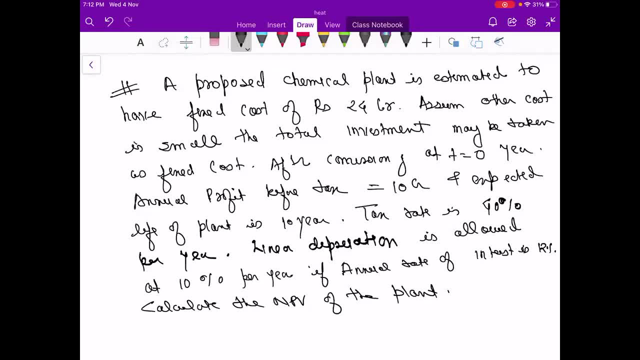 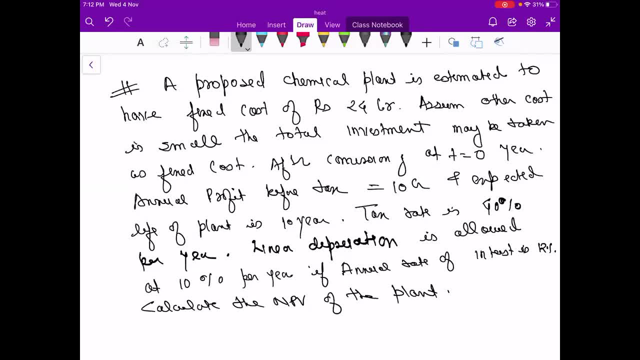 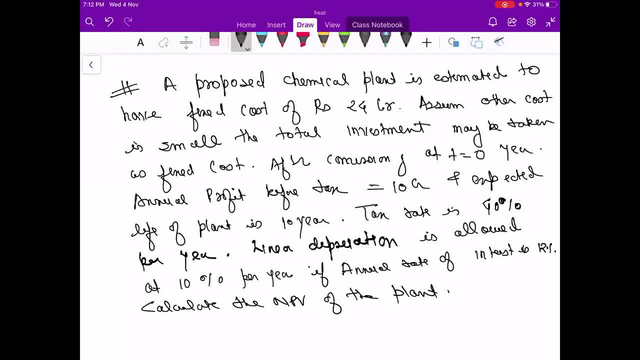 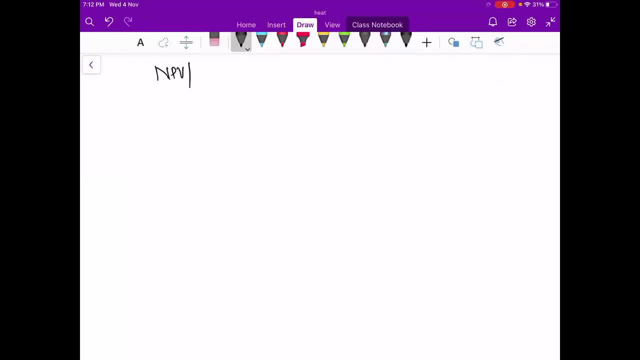 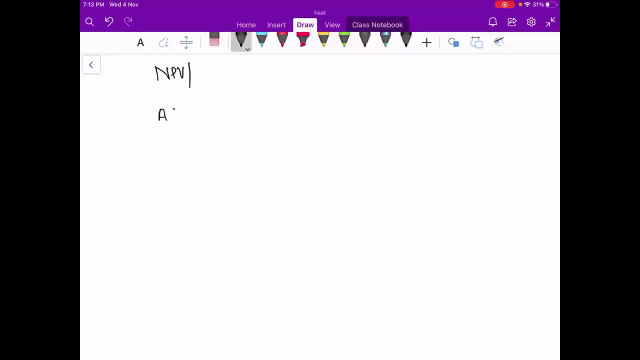 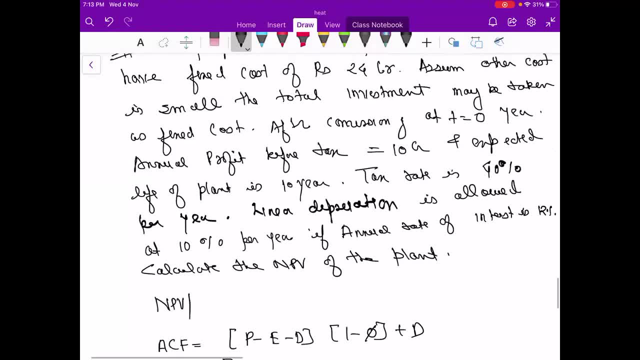 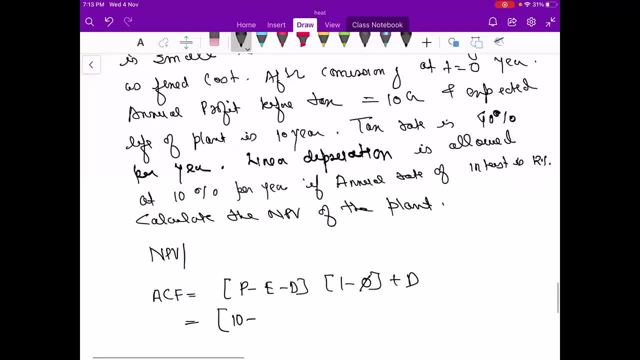 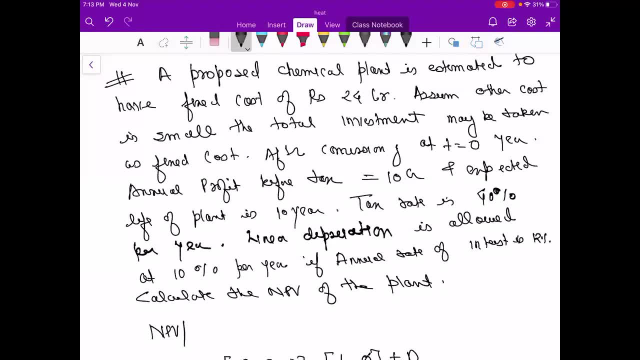 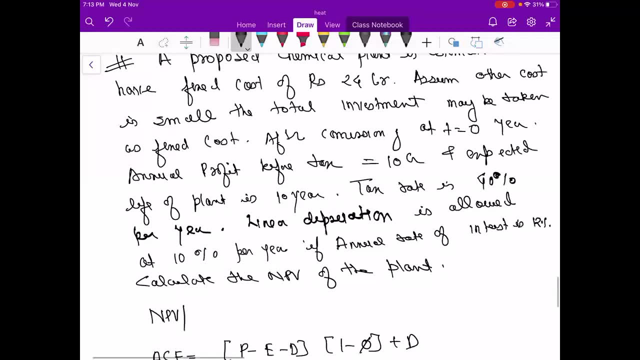 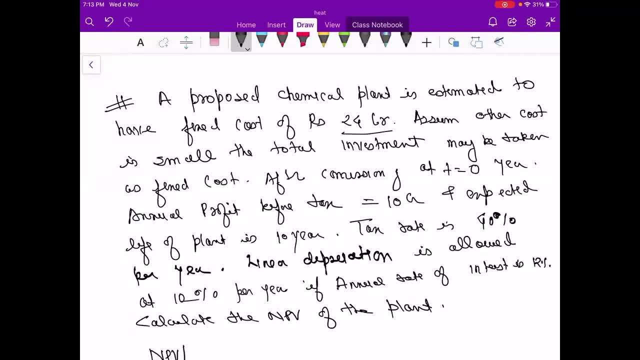 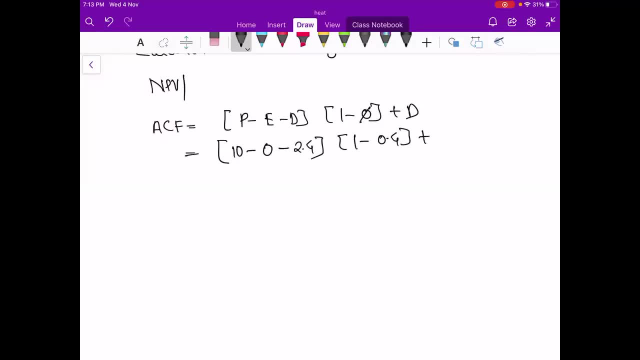 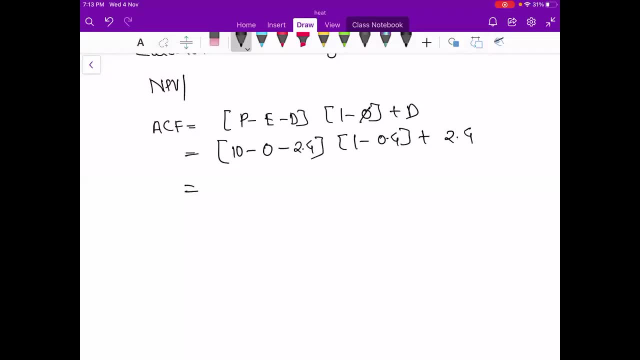 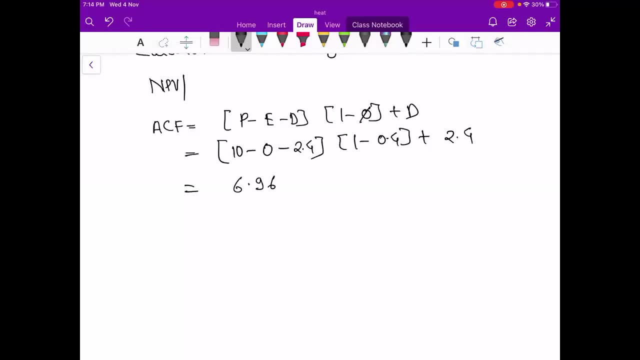 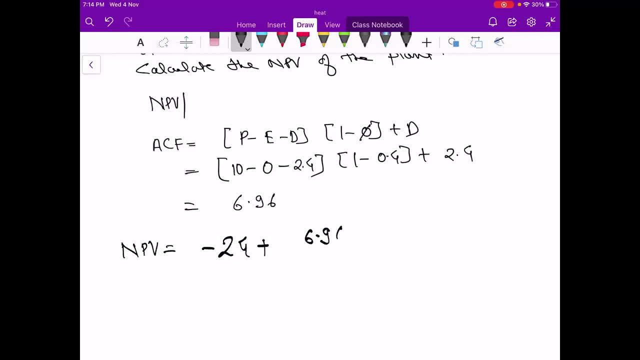 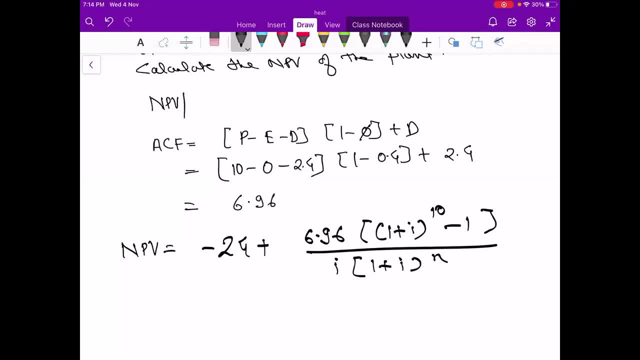 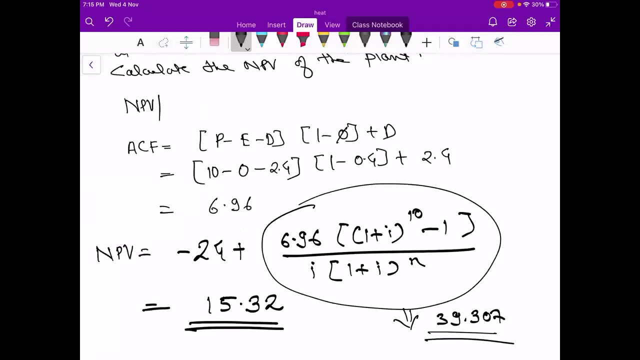 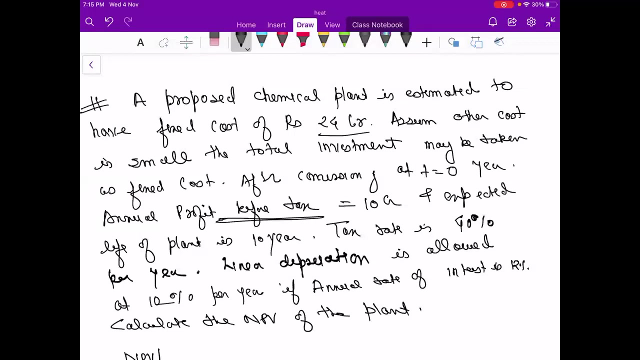 i 1 plus i to the power n. so i think correct answer is 15.32. most of the students got the correct answer. okay, yes, this answer is coming. i think this answer is coming. some student has written 39.307. okay, okay, profit is after tax. it is given a before tax again what you are reading see: before tax. 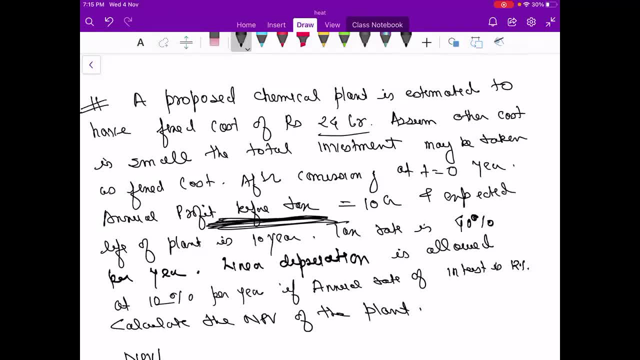 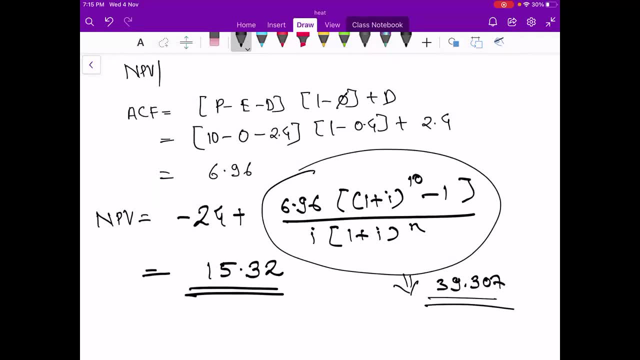 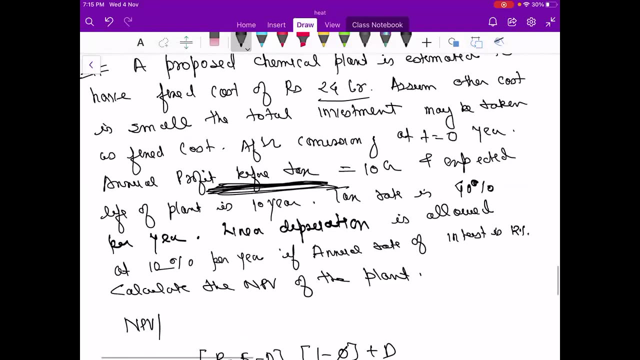 clearly mentioned, depreciation is not 2.4 by 10, it is 24 by 10. how it is 2.4 by 10? it is 24, so it is 24 by 10. why are you writing 2.4 by 10? 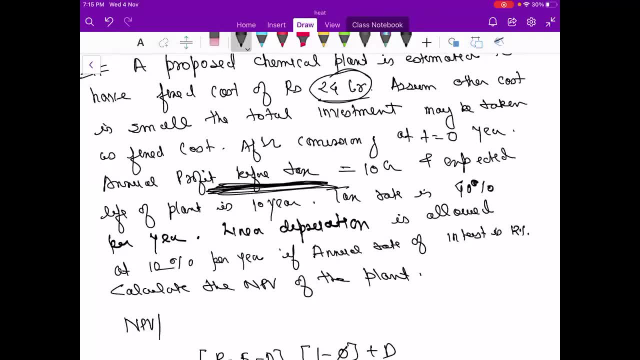 yeah, so it is 24, 10 years. they have mentioned now life of plant is 10 years. they have mentioned this 10 years and this is 24 crore. okay, anyone has other doubt? ask? clear your all doubts. okay, everyone is clear. okay, okay, okay, okay. 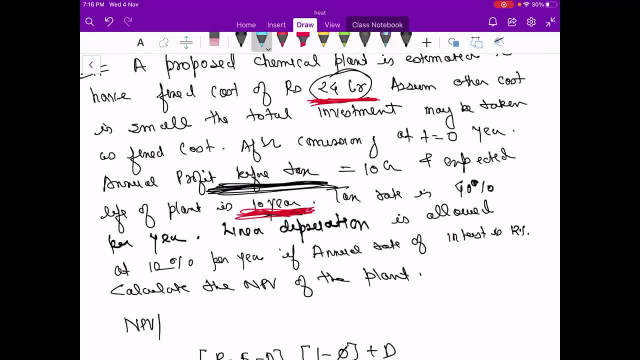 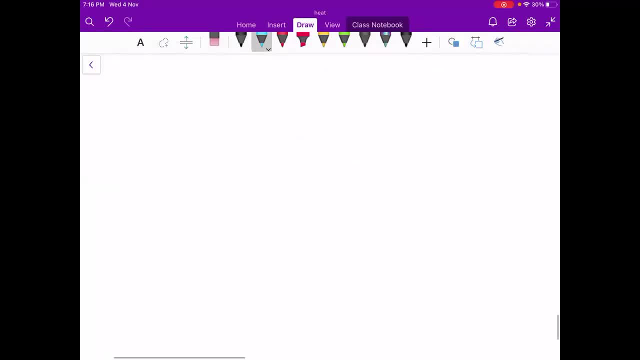 okay, okay, okay, or okay, or happy, happy day. what time do you mean yes? so what time do you mean yes, 2, 116, yes, 2, 1176, okay, so now in this question, suppose we want to calculate npv. at time t equals to 0, how much it is minus 24? so calculate it. 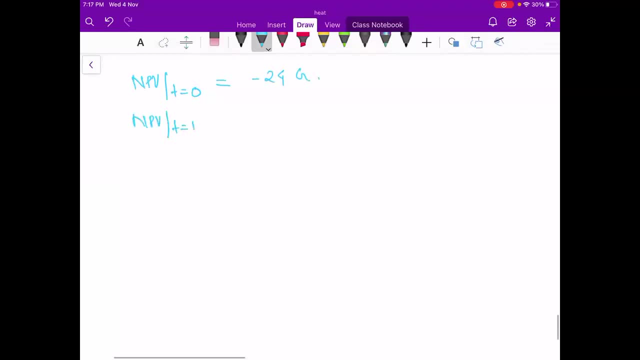 fast. for npv, time t equals to 1. calculate it fast, how much you are getting. calculate it after that. calculate npv for t equals to 2. after that calculate npv: t equals to 3. after that calculate npv equals to t equals to 4. 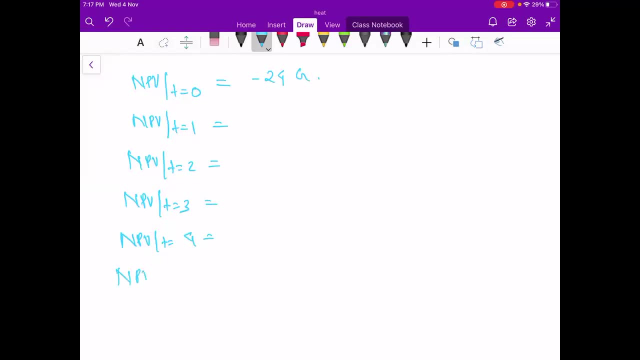 okay, after that, calculate npv: t equals to 5. calculate fast all the values. i think someone has written this is coming minus 17.7. yes, it is correct, calculate it fast. second, third, fourth: someone calculated for 5 directly. okay, someone calculated directly for 4. someone calculate for? 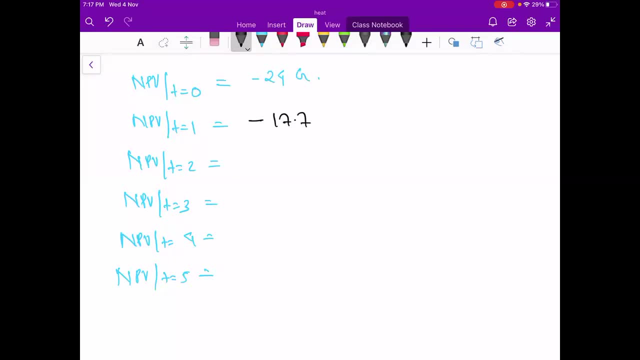 2, 3. do it fast. second year: fast calculate. why so much time? okay, someone has calculated directly for fifth year. okay, so it will be 1.0892, okay, 1.0892, 1.0892. okay, someone calculated for two year minus 12.24. very good, someone has calculated for. 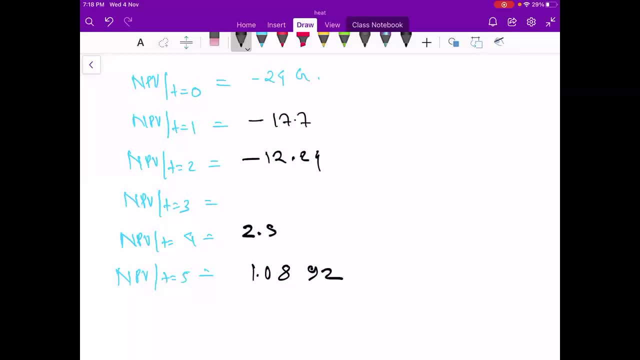 uh, fourth one: 2.896. calculate for third. yeah, it is minus minus 2.896. third, calculated fast. third, minus 19. i don't think so it will be minus 19. it should be less than minus 12. na, yes, it should be minus 7.28. okay, so it will be. see here it is 24 crore. it is minus 17.7. 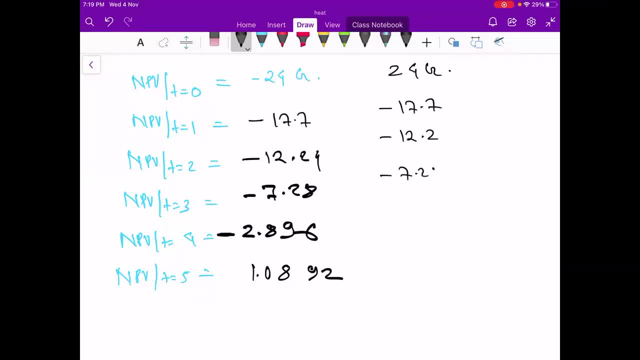 it will be minus 12.2, it will be minus 17.28, it will be minus 2.896 and it will be 1.08. so if you draw the uh, do the analysis how it is going on. see here: initially it is 24 crore negative. 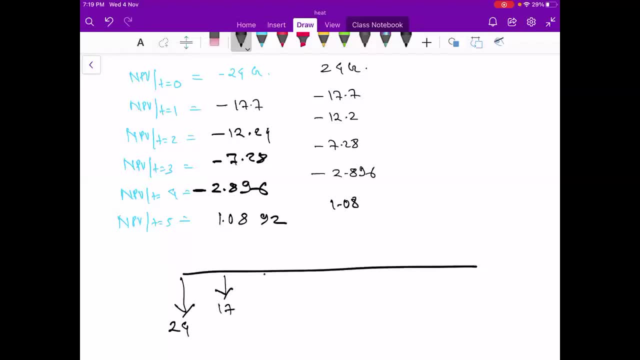 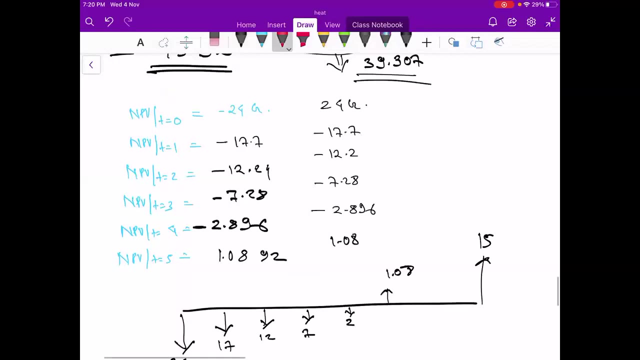 okay, then it is 17, then it is 12, then it is 7, then it is 2. now it is come upward: 1.0, 10 and at final it is- we have calculated it- that is 15. so your graph is going like this, see: 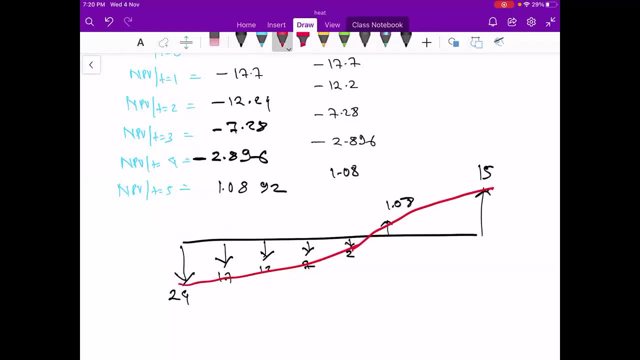 okay. in between between fourth and fifth it becomes intersected, okay, yes, below part, you can take it. this below part is loss, okay, and this upper part is profit. yes, below part, you can take it. this below part is loss, okay and this upper part is profit. sorry, so everyone got this. 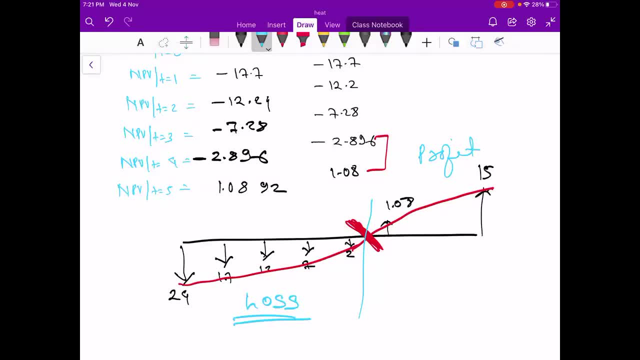 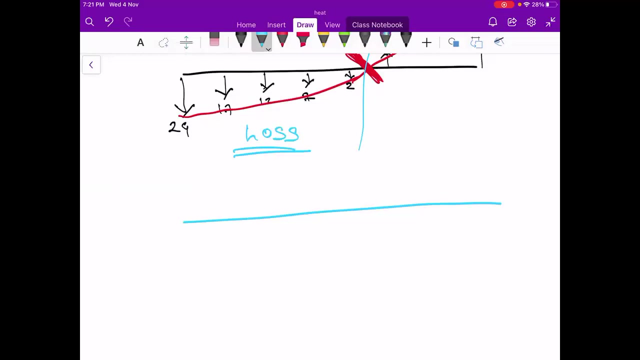 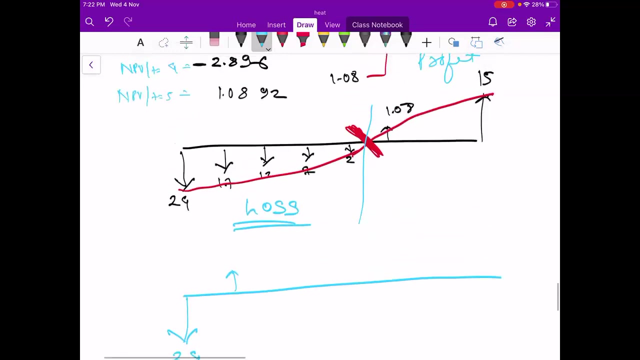 everyone got this or no. everyone is now comfortable. Everyone is comfortable. So, in general, if you draw a graph, so it will be like this: initially, here you have got 24 crore rupees. now, every time you are getting, every time you are getting some value. 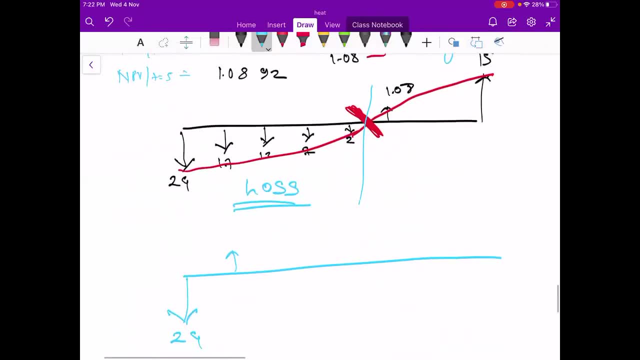 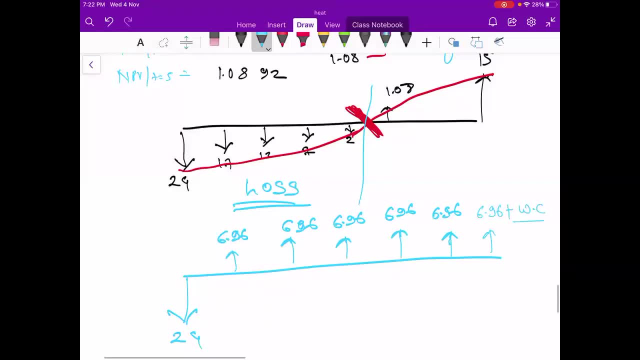 you will be getting 6 point 9, 6 plus working capital. okay, plus working capital, you will get Okay. What are you writing? 2, double 1, 4, 5, 9 for NPV. you gave two formula. no, I have given only. 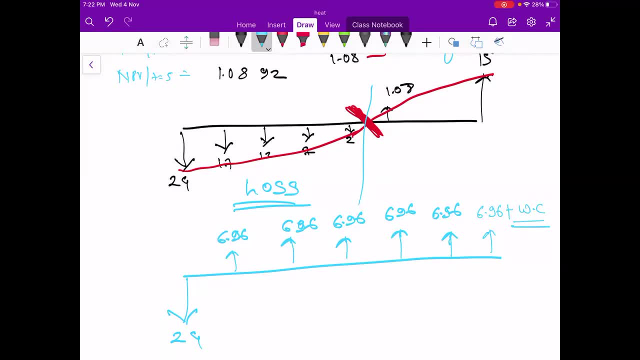 one formula, That's it Okay, One which you do now and other than you use it: NPV equals to minus investment plus x 1.. See, when you are saying that x upon 1 plus i to the power, n plus y upon 1 plus i to the 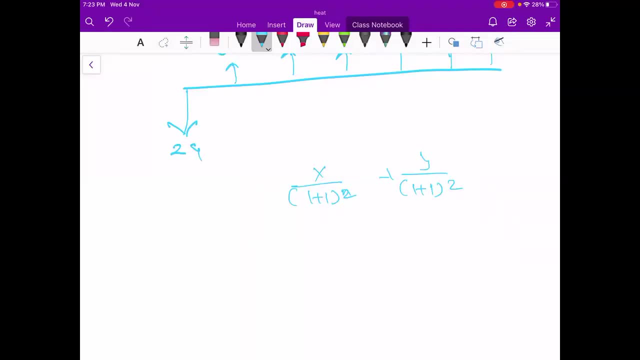 power 2.. Which formula is this? Rule number 2: 1, 1, 4, 5, 9.. Which formula is this? This is NPV formula. This is NPV formula only if x equals to y. If x is not equals to y, then you have to follow this method. 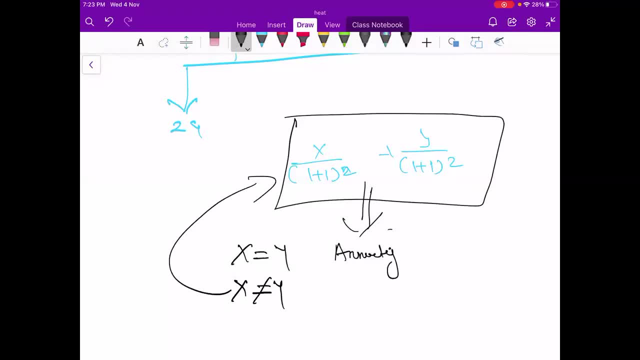 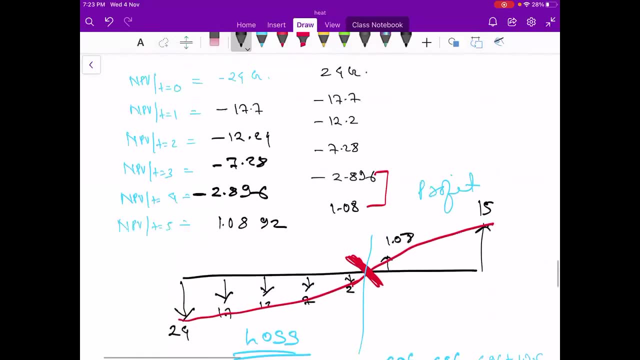 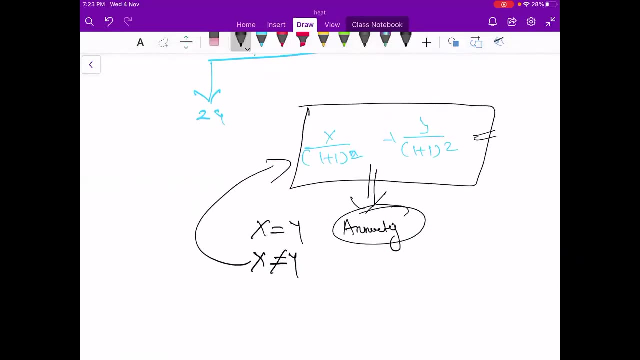 Okay, Okay. Okay, then directly apply the NVT. I have just given shortcut. You can use this also. You can just calculate it. You can do this for You: apply NVT formula for two years and you solve it like this. You will be getting same answer, because NVT is the same thing. OK, Yes, you. 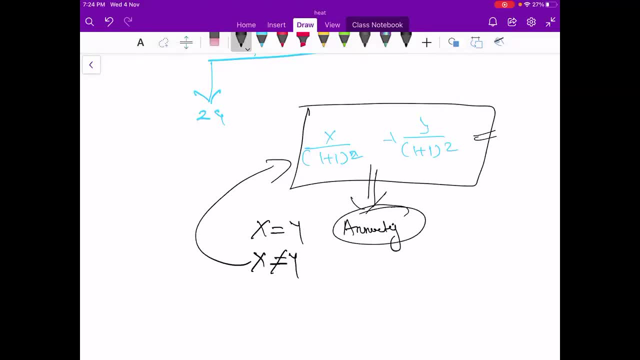 can say: double, two, zero, two, seven, three. OK, That is the point. But generally we don't do like this. OK, So in between, because four and five, you can say there is a point- You will be getting the same answer. OK, Because while calculating that we break even point. 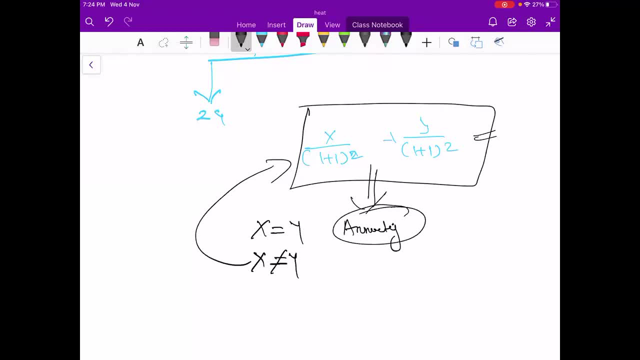 which strictly mentioned the number of products. What is the selling price, What is the cost price? Here we are not exactly mentioning that. OK, In this question, if you see, we don't know the working capital. OK, So that's why. 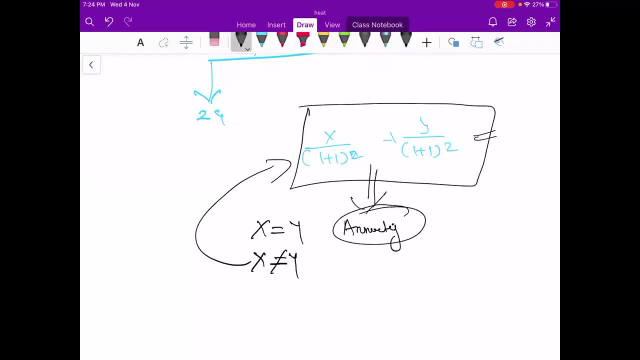 OK, Now everyone is comfortable, yes or no? OK, Everyone is comfortable. Bolo samajhla ki nahi, Samjha ki nahi Samajh ma aaya hai ki nahi aaya. Bolo haan ki naa Samajh ma aaya sabko. 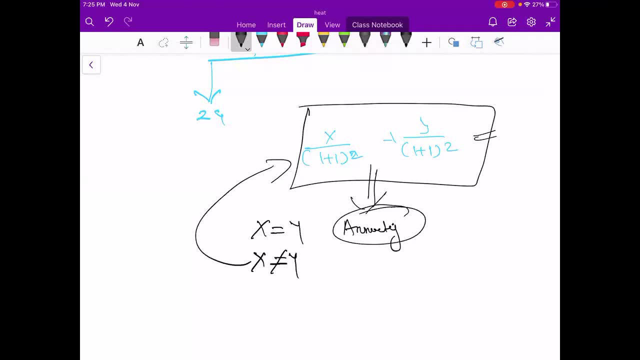 Saikat tum so gayi the kya. We will see, Samvit, if time is there. OK, It depends on time. OK, Everyone is comfortable, Hope everyone is comfortable. We will move forward. OK, As you can see, it's less than four numbers, but it is still correct. 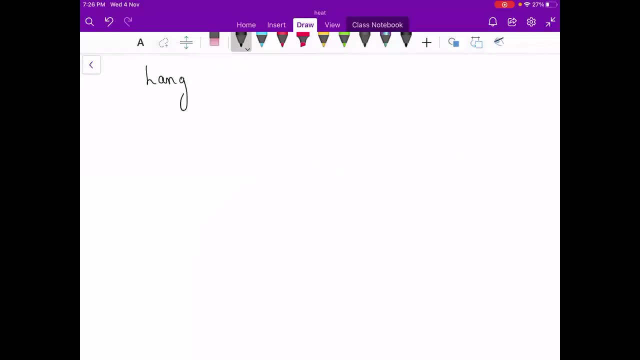 There is a term, Lang multiplication factor. OK, Okay, from this part, only from last 30 years Gate has asked only one question. OK, So basically, Lang multiplication factor is nothing but Wow. categorie lashes out: it is the approximation which is done by some scientist, economic scientist, he told that 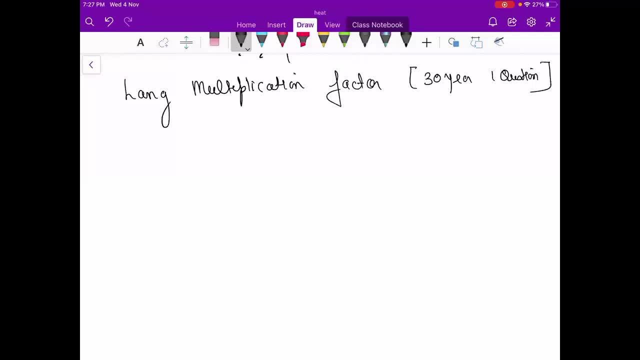 whenever you are going to start an industry. okay, whenever you are going to start an industry. so, depending upon the- okay, depending upon the equipment cost- okay, depending upon the one equipment cost, you can just calculate the approximate money is required for starting your plant. okay, because we know that when we say that we required a money, so it is approximated. 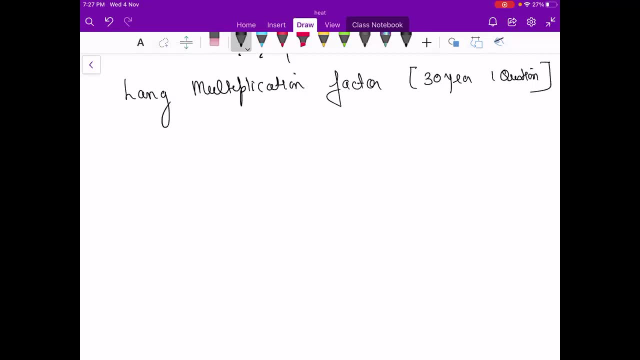 means whenever you you say that you are going to build a home, okay, so it will be approximated money. if you say it is 20 lakh, it is not going to happen that it will require just 20 lakh. okay, it is similarly when you are going to start an industry: you will just approximate that, okay. 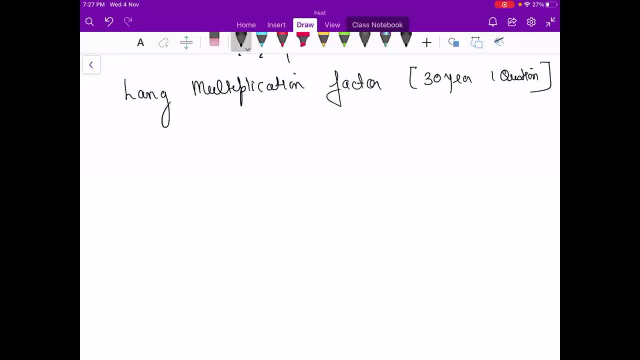 you required a 1.5 crore, so is it that you will be requiring exactly 1.5 crore? no, 30, 40 lakh is plus, minus. is okay for that, okay, okay. so, similarly, the land multiplication factor: is that basically based on his experience and 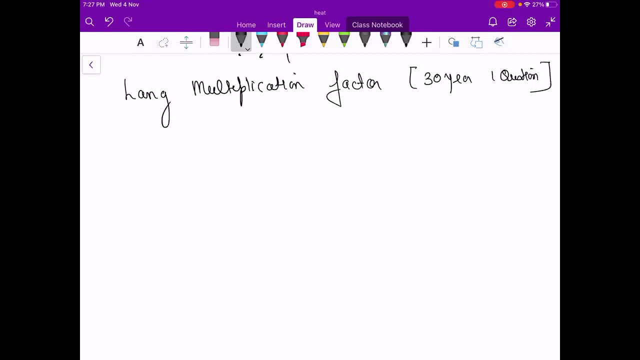 all that means on not on experience. we can say, based on the reviews of different industry and all that he had just mentioned, some constant okay and you have to remember the constant okay. so for solid processing we will do the question also which they have asked in the gate examination. 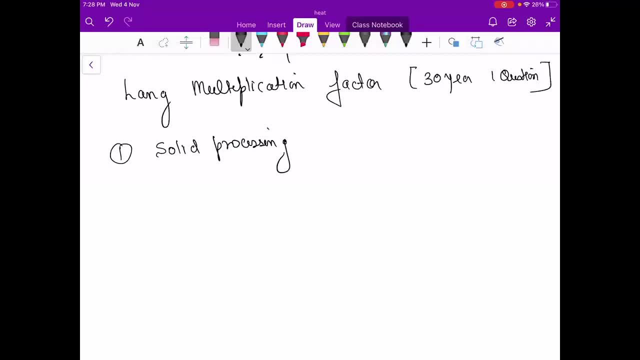 only for the one mark and that is only for one time. solid processing. so there are different types of industry. for the chemical industry, again, this will be a product, okay, solid processing. then you are processing a solid fluid processing, okay. third, is the fluid processing okay. so he has mentioned. 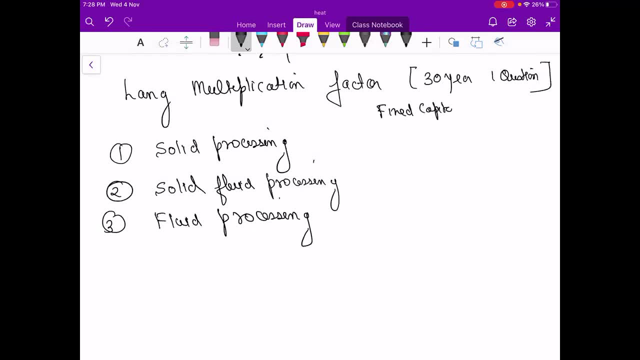 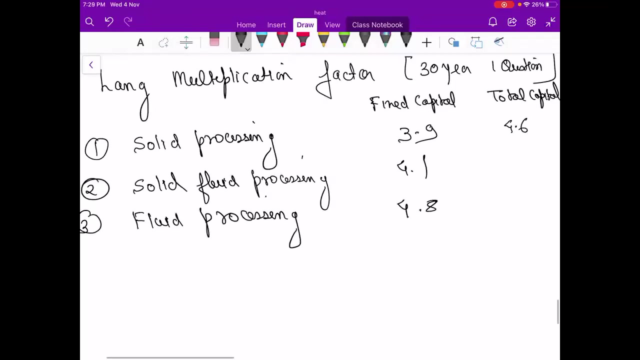 suppose fixed capital and total capital. so it will be like that: three point nine, four point one, okay, here it will be four point eight, okay, four point six, four point nine, and it will be five point seven. So you have to remember this. There is means, no shortcut. you have to remember this table. okay, I will tell you that how they. 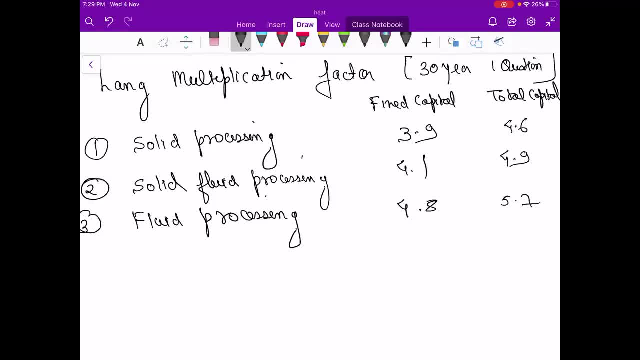 can ask the question uh, related to this, but you have to. you have to, you have to download it. I will tell you how it is from the link. Okay, so one question which they have asked in the grade examination. I will tell you the question. 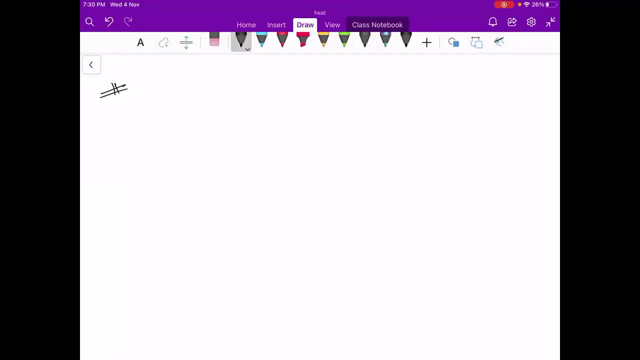 Okay, and so the question is like this for a solid. so the question is like this: for a solid, for a solid, for a solid, solid, for a solid, solid, solid, solid, solid processing plant. the delivered equipment cost is Rs 10,00,000. okay, using land multiplication. 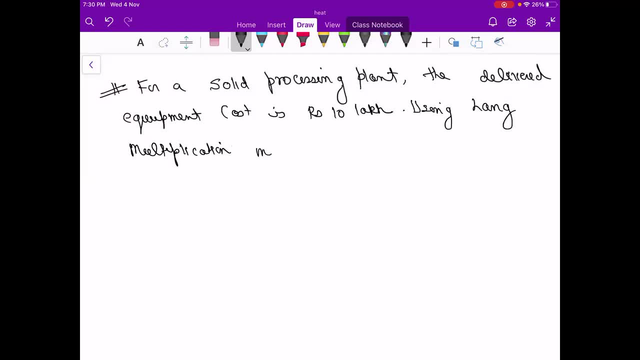 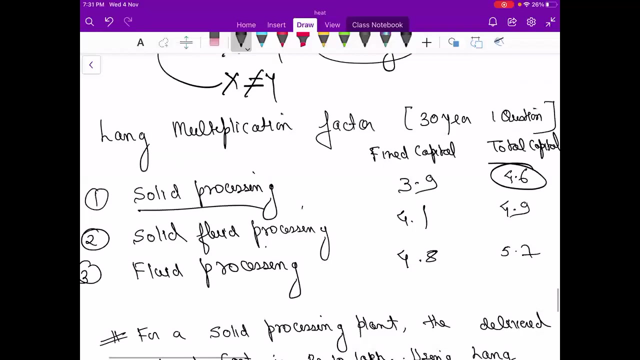 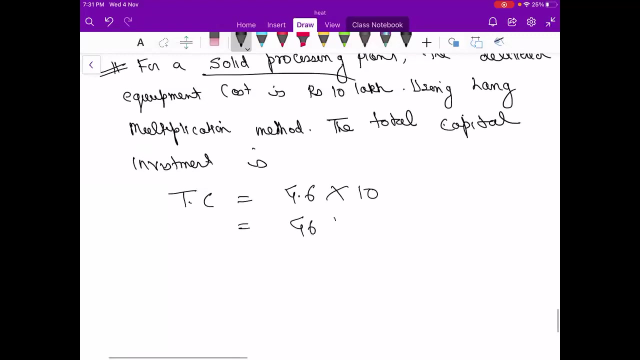 method. the total, the total capital investment, is, calculate it. yeah, the answer is directly, 46,00,000. okay, but for that you should remember that constant. okay, see here 46, and it is solid processing. okay, so it will be 4.6 into 10 it will be 46,00,000. so this approximated total. 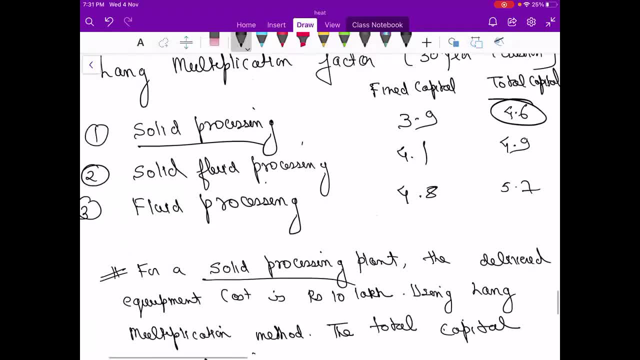 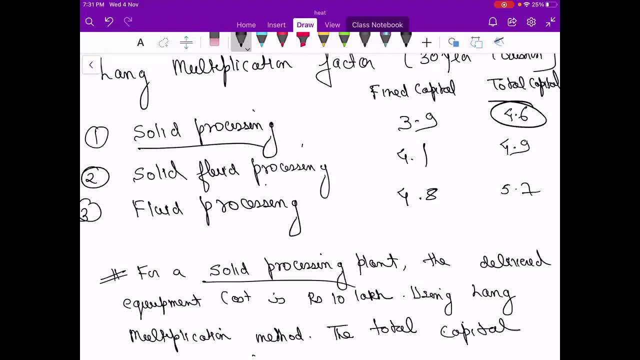 cost required for your system? okay, it will be 46,00,000, so you have to remember, okay, so this is the only question which they have asked in the last 30 years. okay, significance of this is basically that, depending upon the reactors, how much, what is the cost? 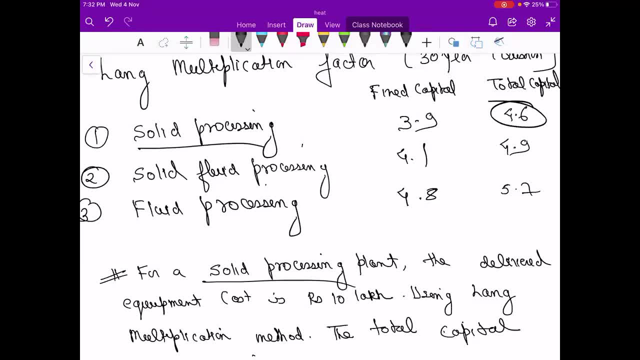 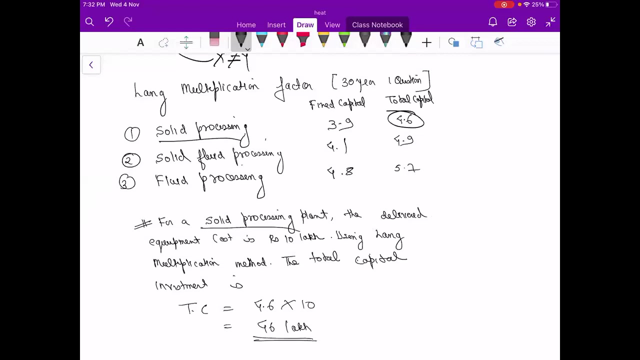 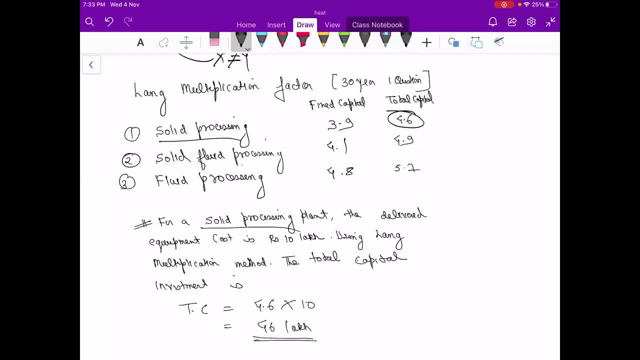 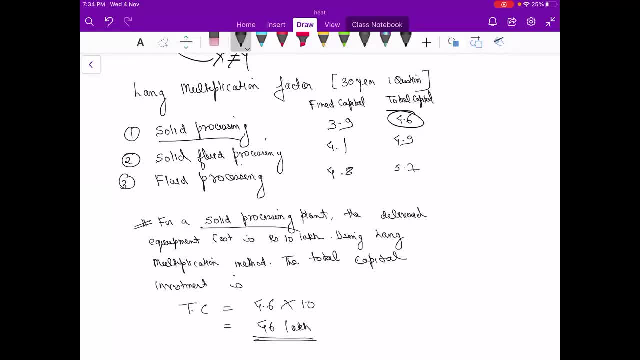 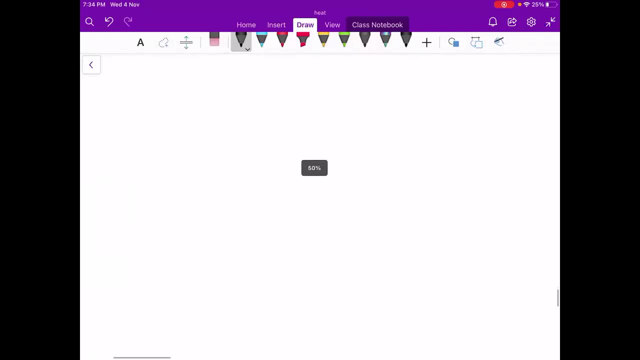 okay, so that is more technical. okay, I don't know from where you have seen this award. this tour is proof of the current related to somewhat share market and all that, okay, okay. next there is one also, formula: turnover ratio. okay, it is defined as ratio of gross annual sales upon fixed 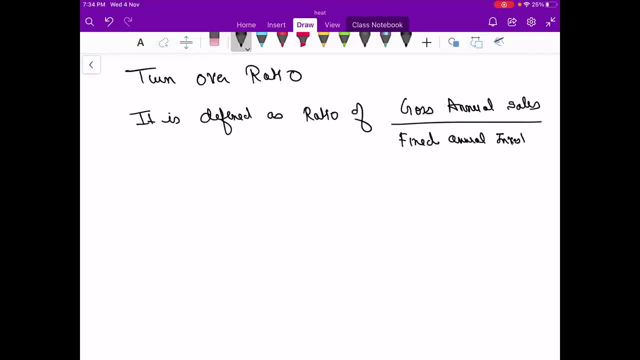 annual investment. okay, you can just write this formula: gross annual sales upon fixed annual investment. sorry, it's not annual fixed capital investment, fixed capital investment- okay. so from this point also, they have asked one question. question is: the total capital investment for a chemical plant is rupees. 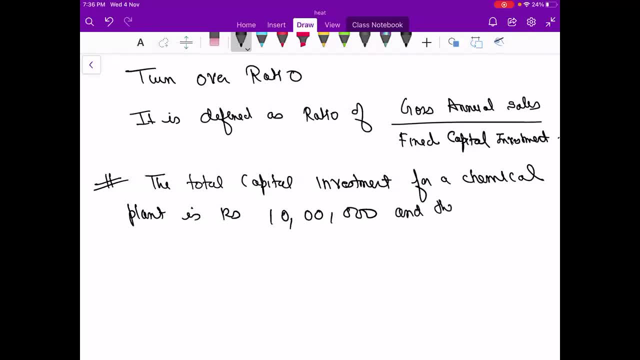 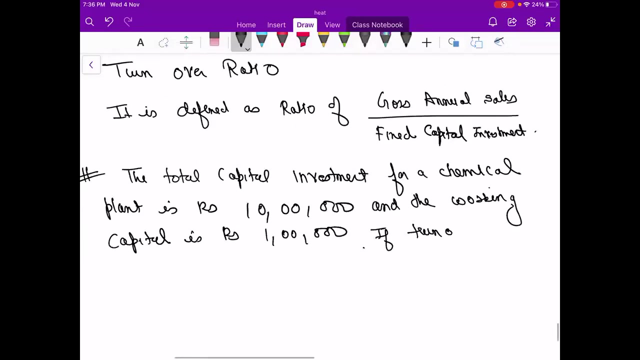 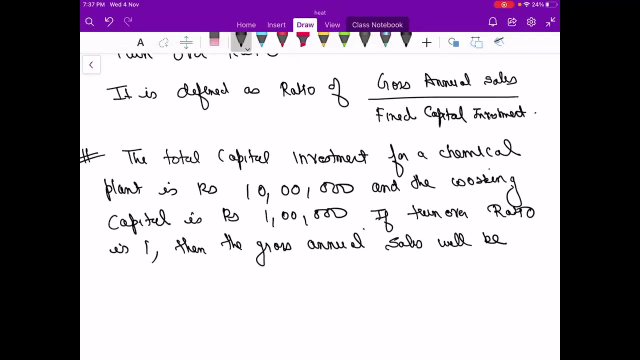 10 lakh and the working capital is rupees one lakh if. if turnover ratio is one, then the gross annual sales will be calculated. so some, tomorrow we will start the designing part. okay, yes, so many students are getting correct answer. so designing part will be start from tomorrow. okay, so today we will get first class answer. 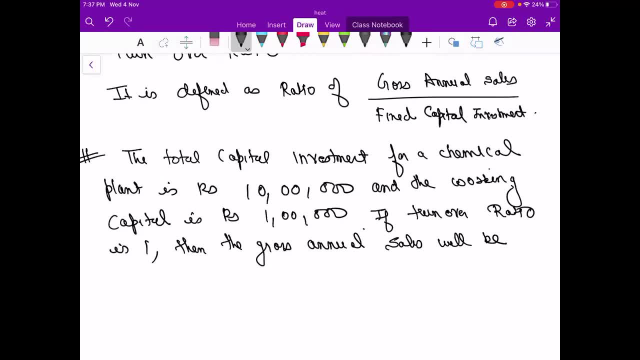 but if you are present in room, then what may be the rest of the session then yes. so when you get these answers, then you should first come back and say: is that value of current number this year or changes to the number finished, the term remaining? then we also take engine into account and this will be equivalent three lessons. this session will contribute to the final part of the training program stream and i will give a letter to you. okay, okay, deste pateальным victory. 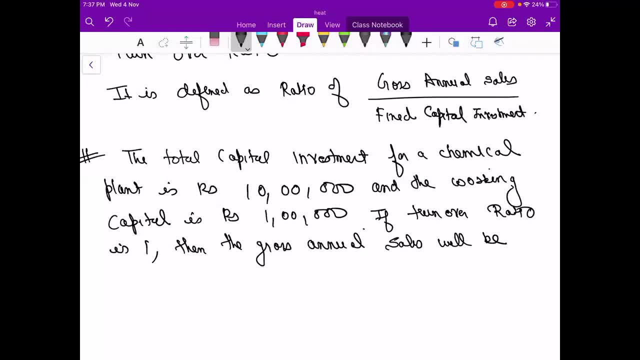 will complete the economics. So almost I think which lecture is this our? this is our sixth lecture or fifth? I think sixth, So it is our seventh lecture. I don't think so. Others confound. this is our sixth or seventh lecture. Some are saying sixth, some are saying seventh. 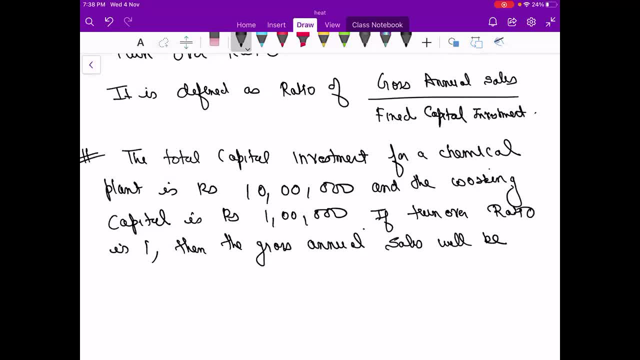 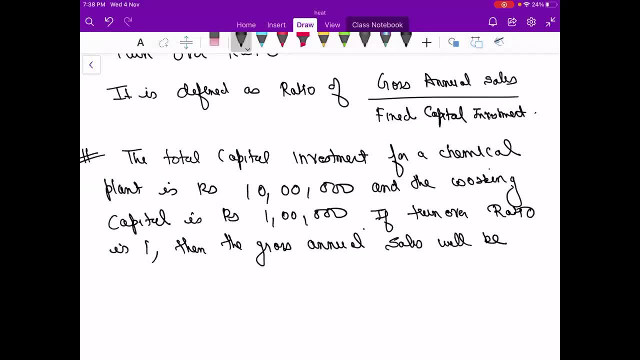 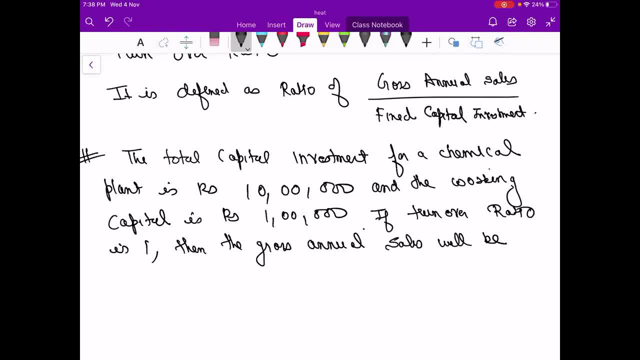 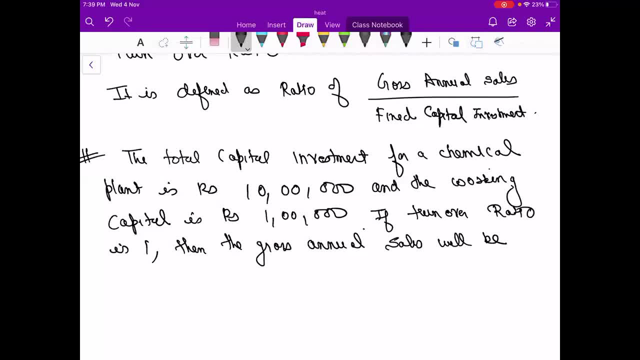 i think it is seven, 14, 14 or 14 and a half hours approximately. we have taken 14, 15 hours, okay, okay. okay, it's fine. 15 hours for economics, okay. so design part: you can expect tomorrow lecture one, two, three, max four lectures. okay means today is wednesday, thursday, friday, saturday, sunday. 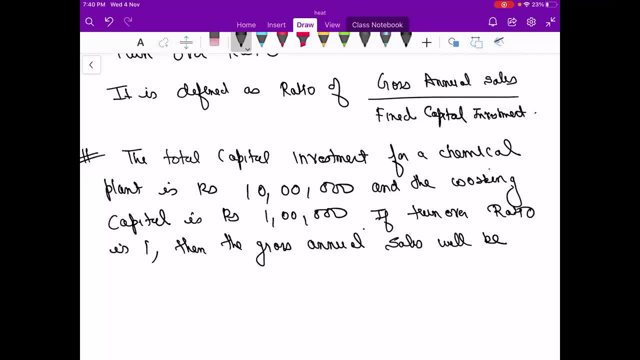 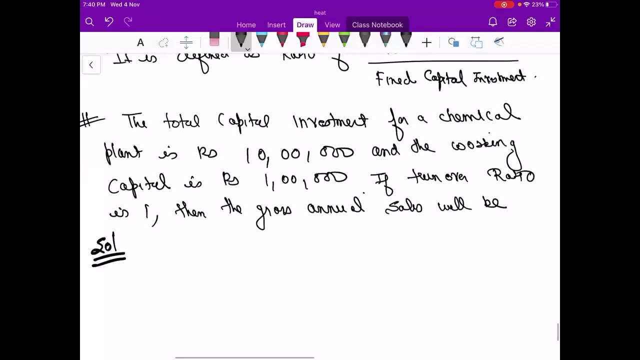 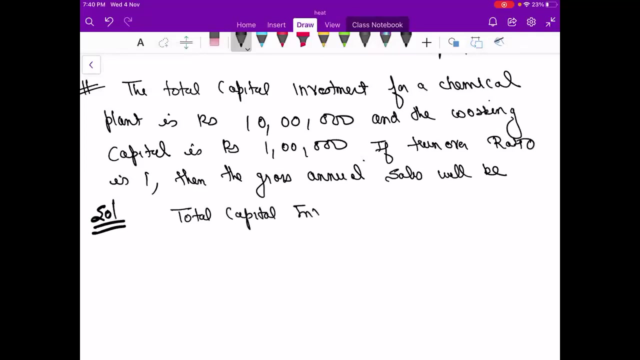 up to sunday. we will complete, okay. max up to sunday. okay, we will solve this question. yeah, yeah, we will solve this question. so it is given total capital investment, but we want a fixed capital investment. okay, so what is the formula for total capital investment? total capital investment equals to: 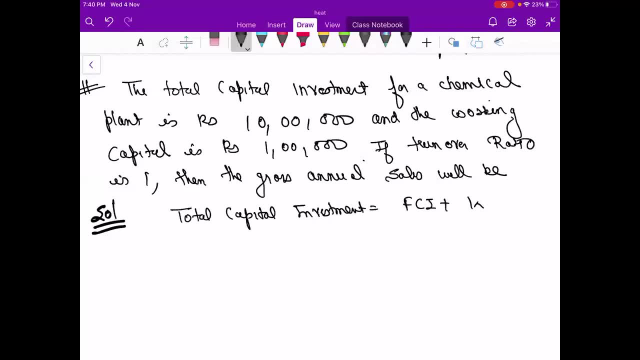 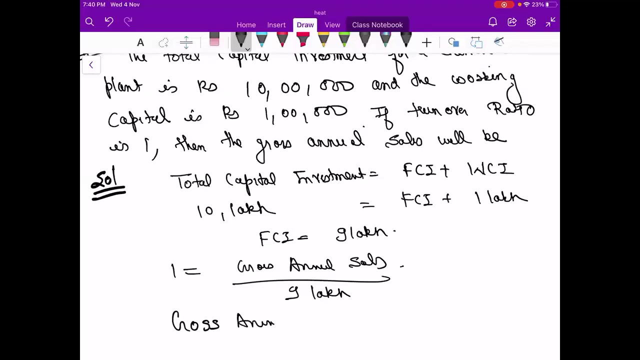 fixed capital investment plus working capital investment. so fixed capital, we have to calculate working. it is given 15 year, 1 lakh and it is 10 lakh, okay, so fixed capital investment will be 9 lakh. so formula is 1 to gross annual sales upon 9 lakh. so gross annual sales will be 9 lakh. 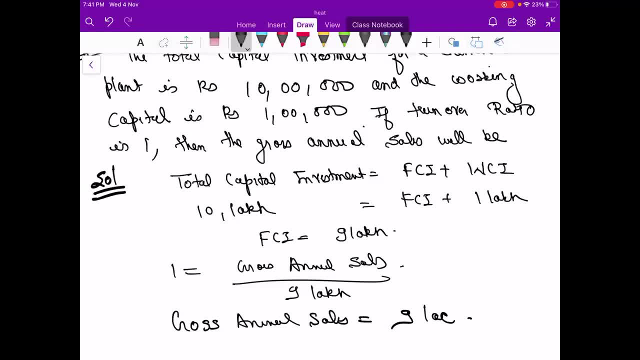 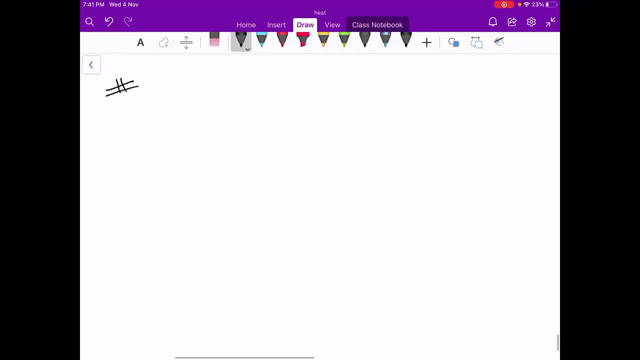 okay. next is investment ratio. okay, next formula is investment ratio, so it is nothing but 1 upon turnover ratio. it is just a reciprocal of that. okay, you, okay. what is capital gain tax? capital gain tax is nothing, but again it is related to the basically sale of a non-inventory methods. okay, so basically suppose you will. so sold some property. 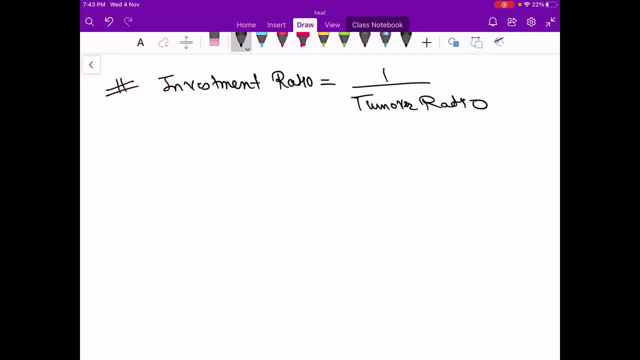 okay, from your home. okay, or you will buy some property. then you have to pay the tax to the government, so that is capital gain tax. so this is not in gates levels, okay, so write one question: if future amount is rupees 10,000. if future amount is rupees 10,000. 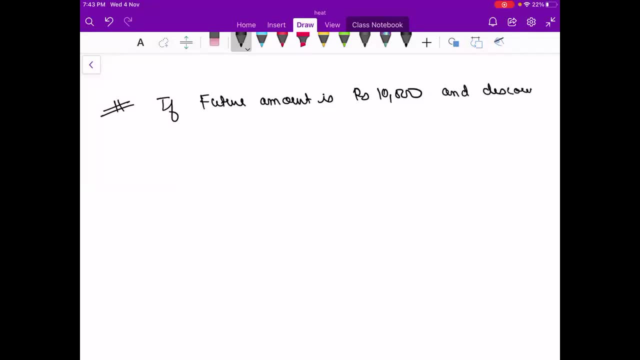 and discount rate of interest is 10% yearly. okay, what is the? what is the discounted amount for today? calculate this. if the future amount is 10 000, here you can write after one year. okay, so how much sale you have done? okay, yeah, it is nothing, but you have to calculate the present value. so present value equals to: 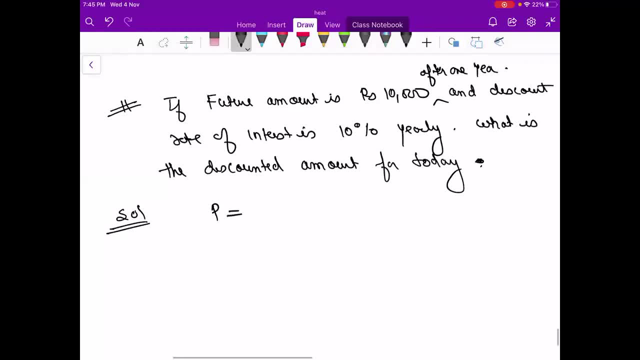 10 000 upon 1 plus 0.1 to the power 1.. so how much you are getting? nine zero, nine zero, okay. so what is the discount you have got? ten thousand one plus zero point one to the power one. so how much you are getting? 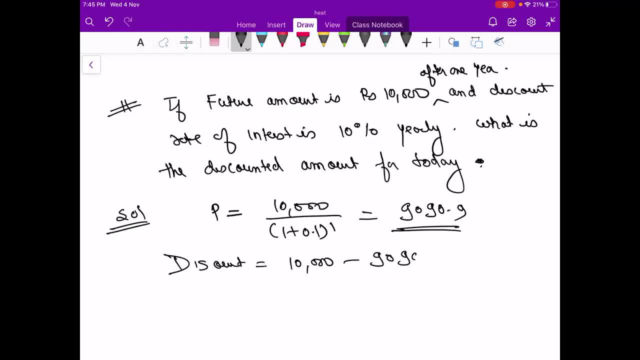 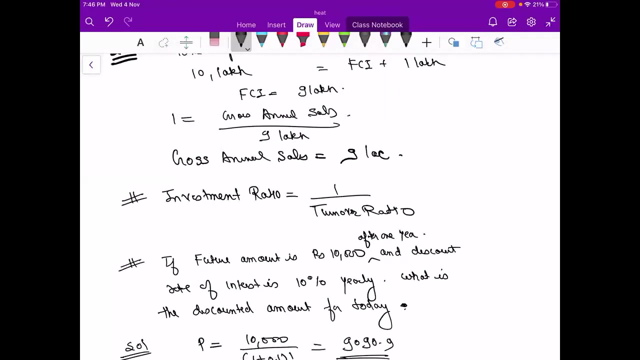 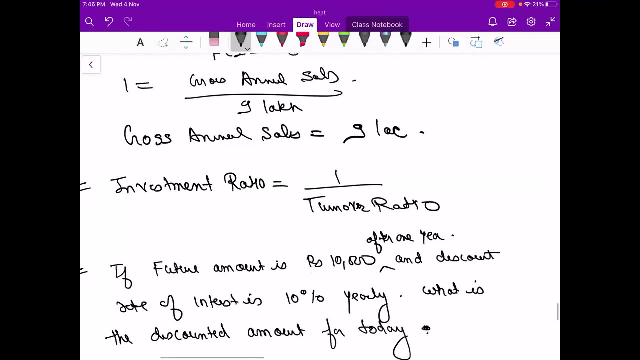 nine zero, nine zero, okay, minus nine zero, nine zero point nine, so it will be approximately, i think, nine hundred and ten, okay, so that's it okay. so this is investment ratio, that is one upon turnover ratio. okay, this is formula: investment ratio. okay, so we will solve some question. 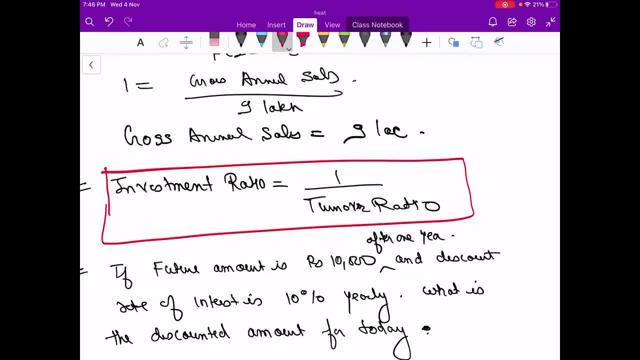 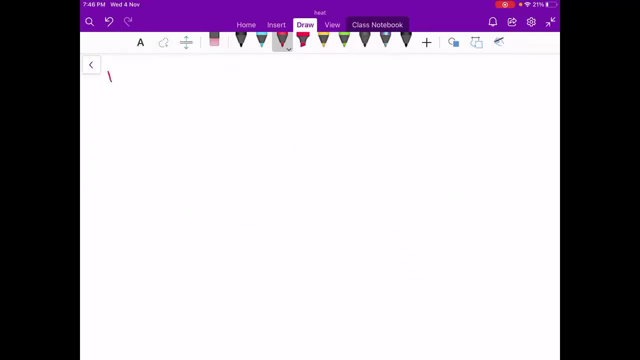 so so write a question: hat the continuous- this is a great question- the continuous to be designed. the following cost figures are estimated first, one is fix cost. okay, so it is cost. it is equipment. so it is six into ten to the power six. two into ten to the power six. four into ten to the power six. it is column, it is. 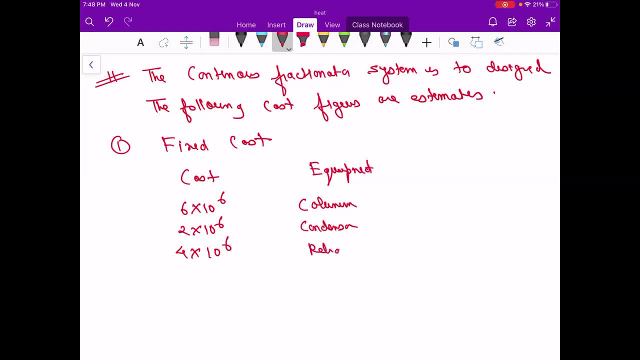 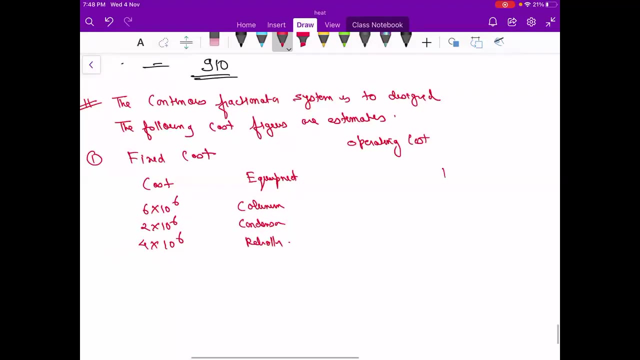 condenser. it is a reboiler. now next is operating cost. so again same thing. okay, equipment, and here it is cost. so cost is 8 into 10 to the power 6, 1 into 10 to the power 6. here it is cooling h2o. 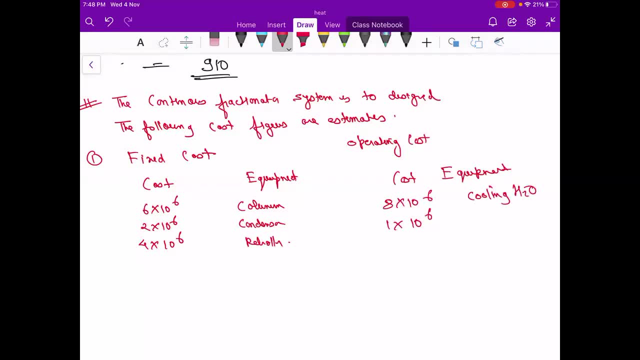 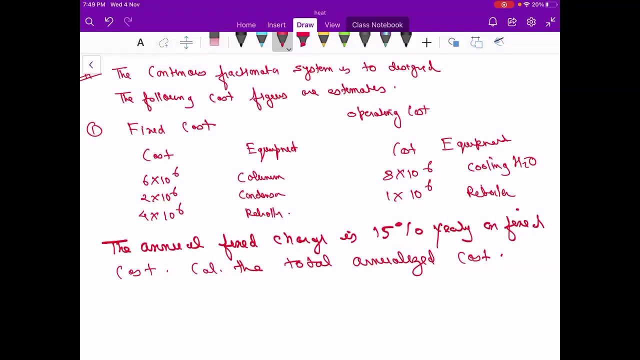 and here it is re-boiler, okay. so the question is: the annual fixed charge is 15. okay, yearly on fixed cost. calculate the total annualized cost, okay. so, calculate this, okay, okay, okay. calculate this, okay, okay, okay. oh, options are given. actually, i can give you the options also. 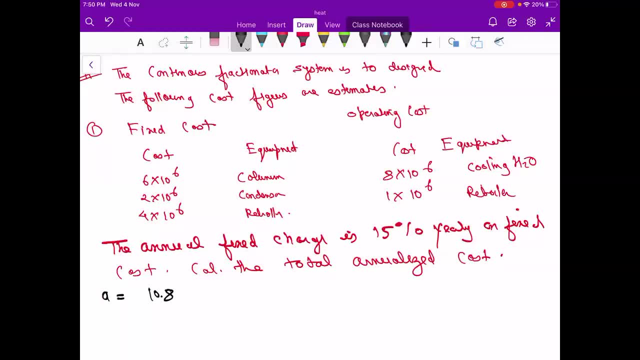 a, 10.8, b, 13.35, c, 15.9, d, 3.95. everyone has 10 to the power 6. multiply. okay, every term is 10 to the power 6, so they have given option 10.8, 13.35, 15.9, 3.95. you have to calculate the total analyzed cost. 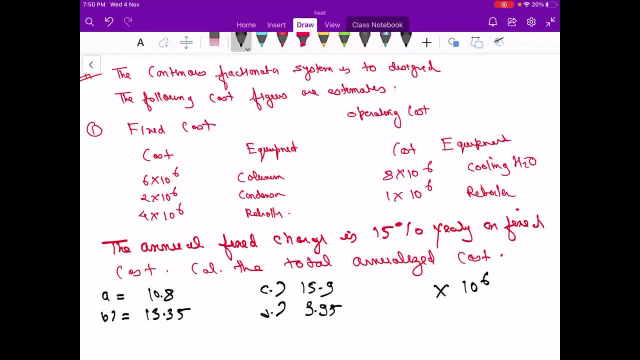 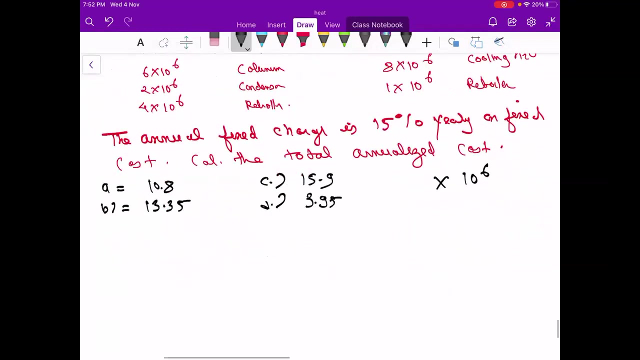 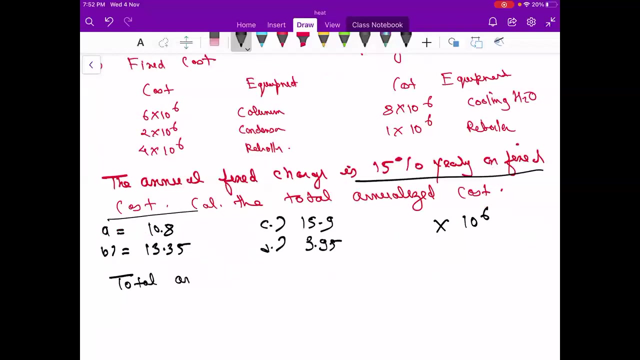 okay, shubham, correct answer. yeah, socket, correct window correct. okay, last one minute, solve fast. so almost everyone is getting the correct answer answer. Thank you, Okay, so we will solve. So they have told 50% on fixed cost. So what is the total annual cost? Total annual cost equals to fixed cost plus what is that operating cost. 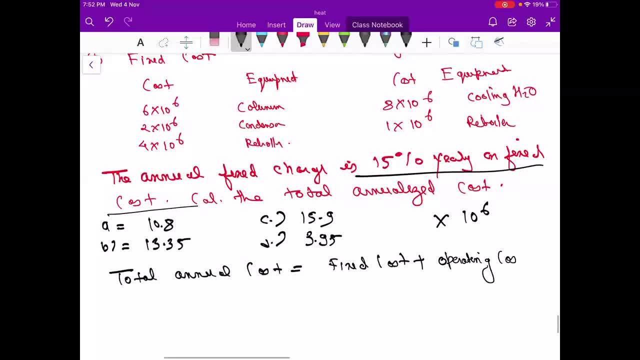 Okay. so what is fixed cost? Six plus two plus four, Okay, into 10 to the power six. What they have said, that 15% is charged on that. So you have to calculate the 15% of that. That is 0.15 plus operating costs. So there is no charges on operating costs. It will be eight plus one into 10 to the power six. 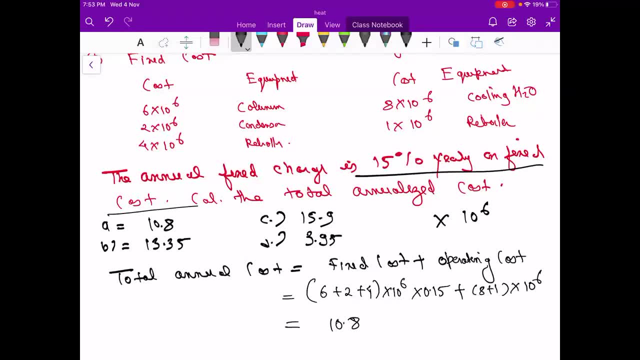 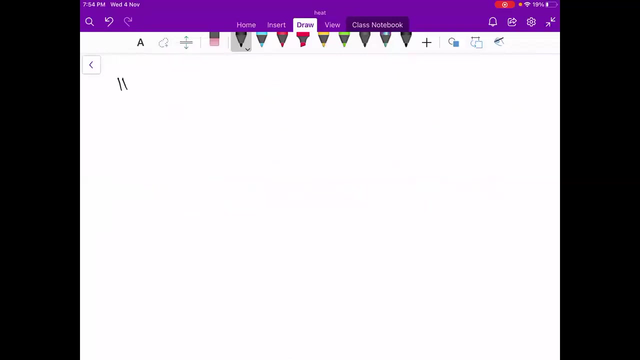 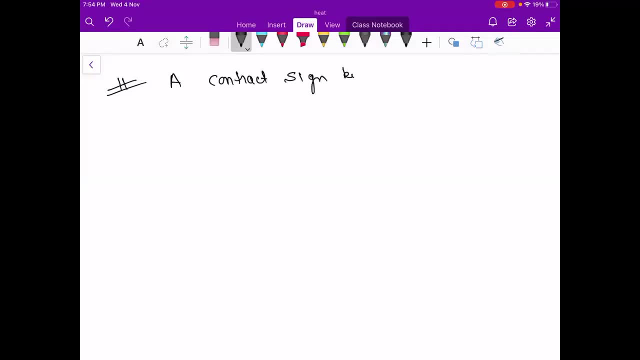 Okay, Okay, Okay. Chemical manufacturer is expected to generate cash flow 2.5 lakh per year at the end of each year for period of 3 years. The applicable discount rate is 10% yearly. Calculate net present worth. Calculate net present worth.